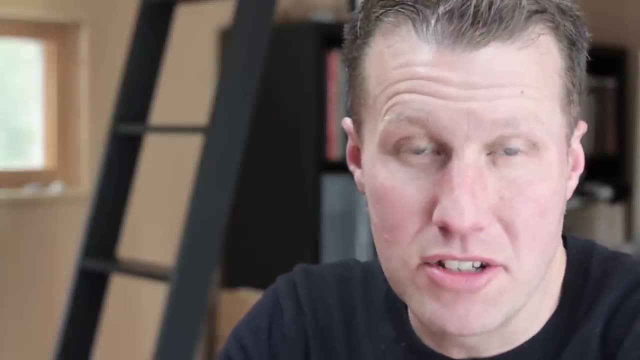 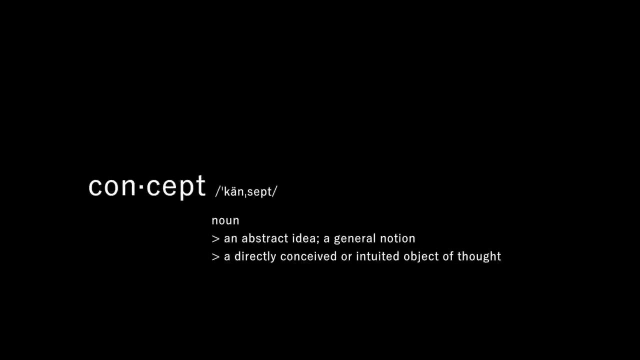 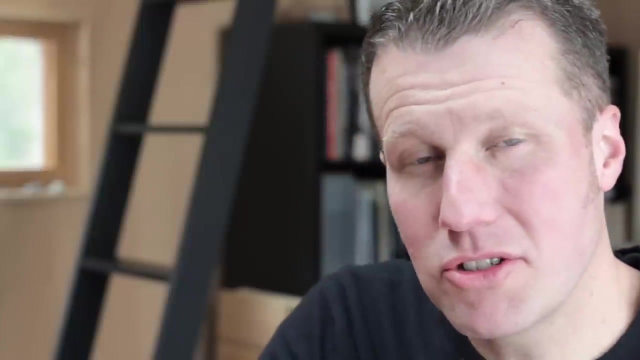 concepts, all illustrated with one of my residential projects. Very simply stated, a concept is an idea that underpins your project. To an architect, the concept is what distinguishes a work of architecture from a mere building. At its core, architecture seeks to solve problems. 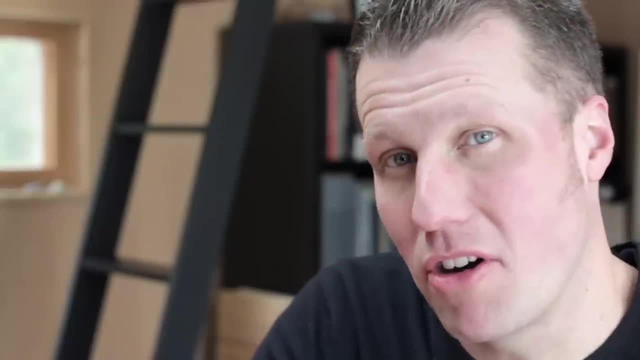 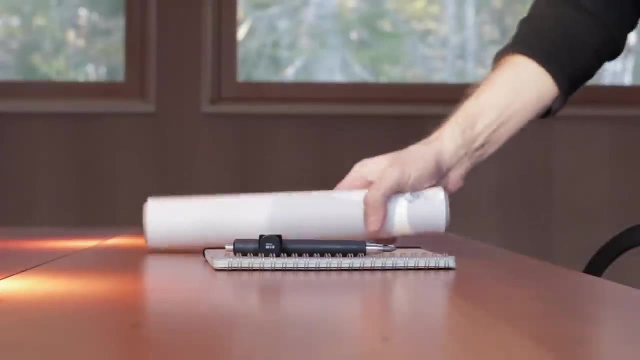 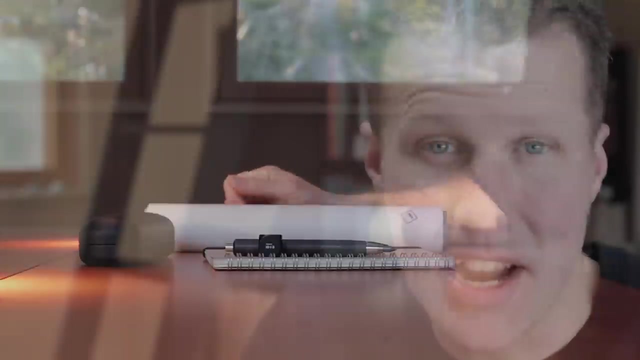 It's the questions we ask that will determine which problems our architecture will solve. Developing a concept allows us to frame the questions we're asking and it guides the design process. Choosing a starting point for your design can be intimidating and an early stumbling block for designers of any skill level, but it doesn't have to be Your concept. 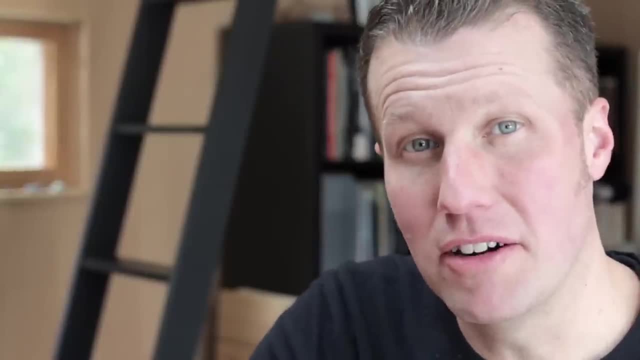 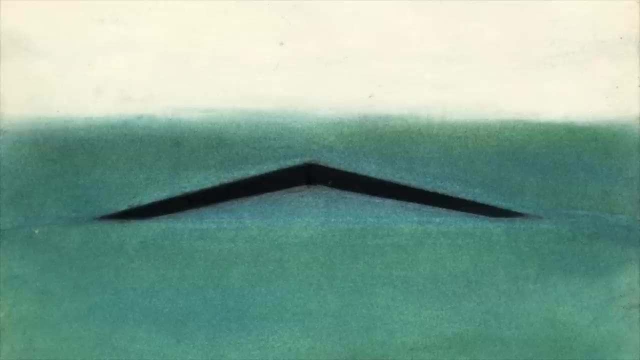 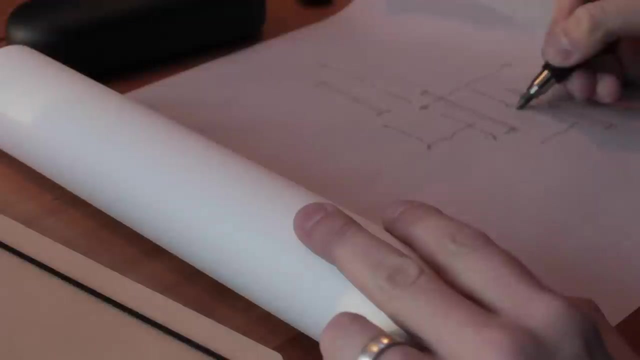 shouldn't be rigorous. The more malleable it is, the better. In fact, most architecture can't be reduced to one singular concept diagram. Rather, it's informed by many concepts working in concert. There may be organizational concepts, material concepts, functional or structural, or 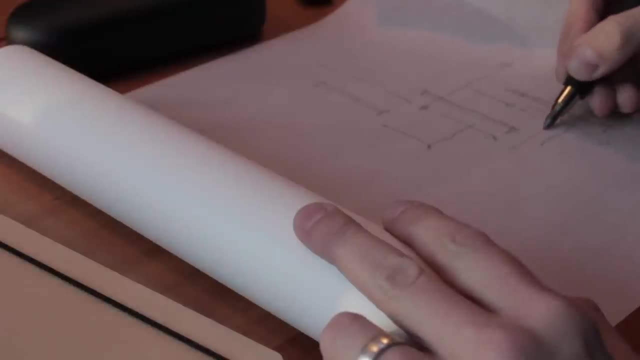 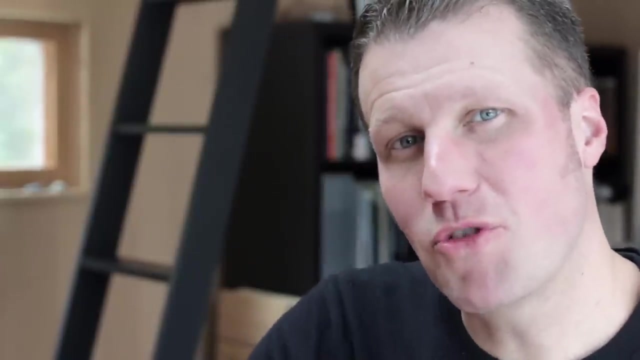 formal concepts. Don't fret if your idea isn't reducible to a single elegant black stroke on a page. It's best to illustrate concept development with a real project. As I said, we'll use our Squid Cove residence as an example. Before we can develop the concept, we first have to understand. 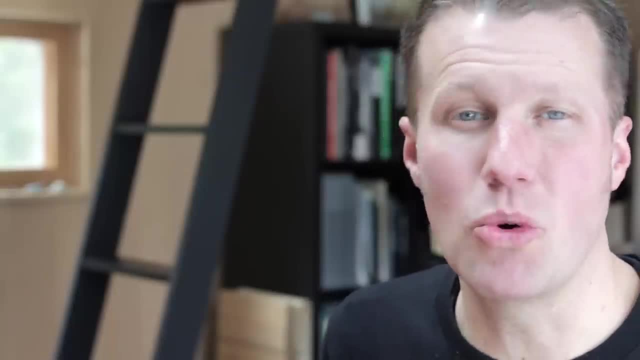 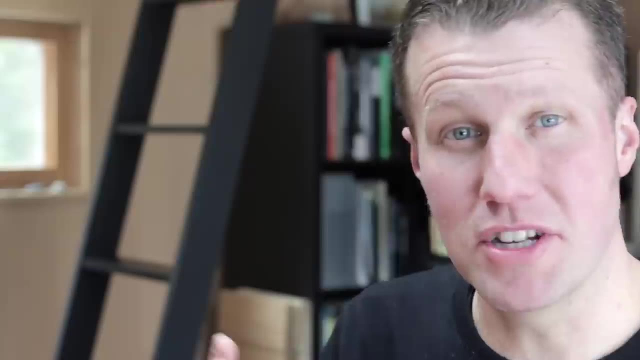 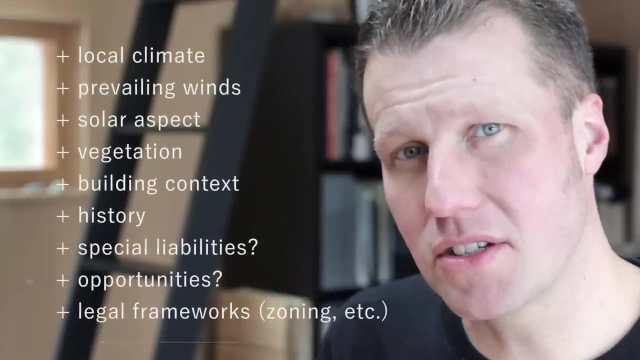 the practical constraints. My design process begins only after gathering and assessing all the given parameters for a project. This primarily consists of three types of information. There's information derived from the site: things like the local climate, the prevailing winds, the solar aspect, vegetation, neighboring structures, the site's history and any unique 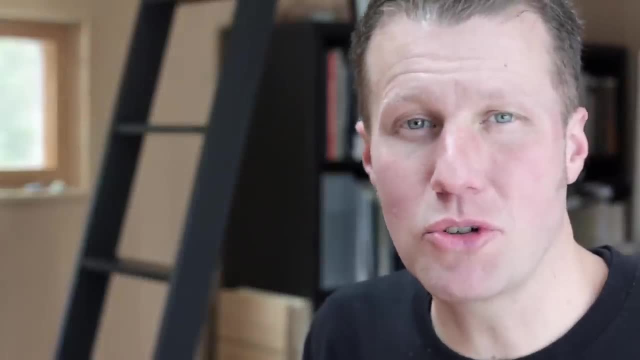 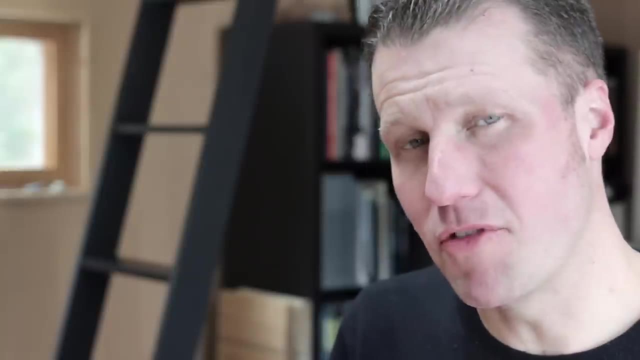 liabilities or opportunities. The site, of course, also comes along with legal frameworks for development which describe where and what we can and can't build. The second type of information we'll gather is from the client. Now, every client has a set of cultural beliefs and preconceptions. 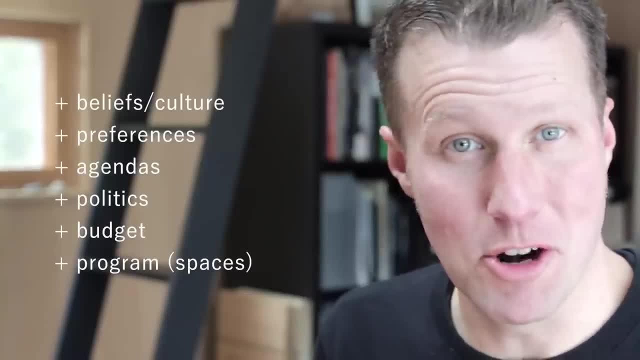 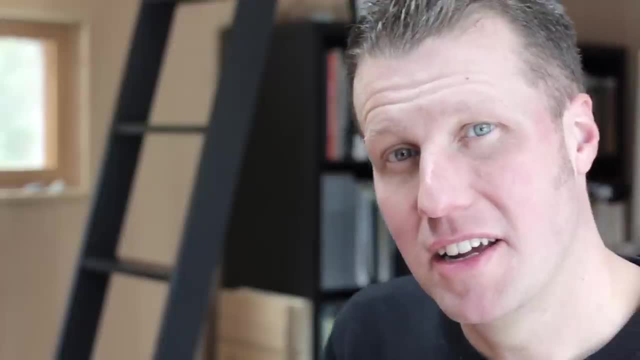 preferences and expectations. Each client has a set of cultural beliefs and preconceptions, preferences and agendas. Of course, we'll want to determine their budget and understand the personality, traits and organizational politics which might also shape the design, The client and the building type. 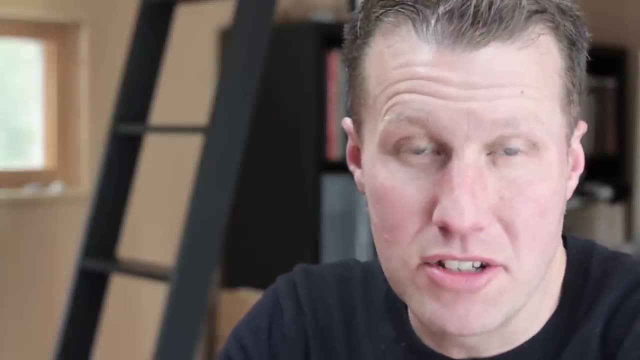 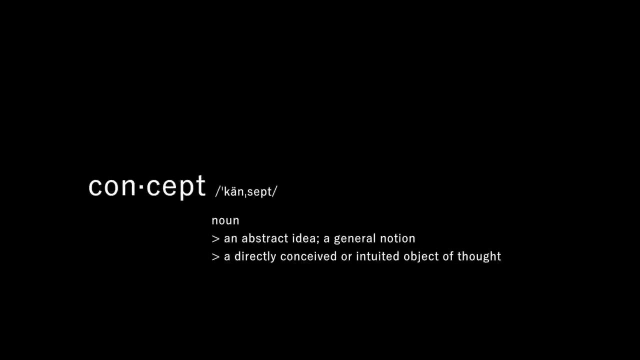 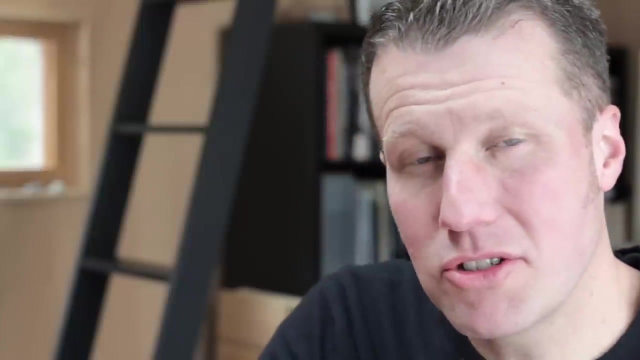 concepts, all illustrated with one of my residential projects. Very simply stated, a concept is an idea that underpins your project. To an architect, the concept is what distinguishes a work of architecture from a mere building. At its core, architecture seeks to solve problems. 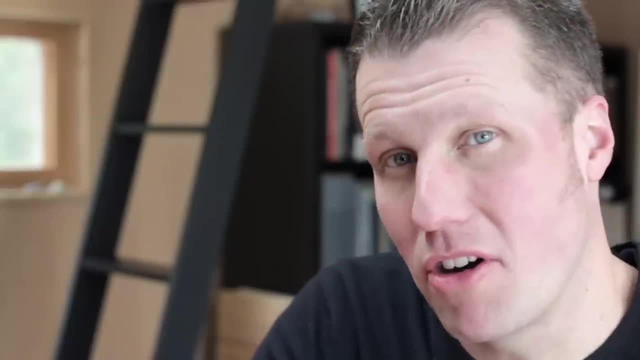 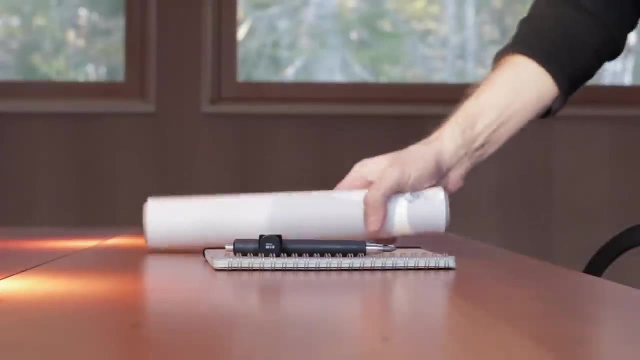 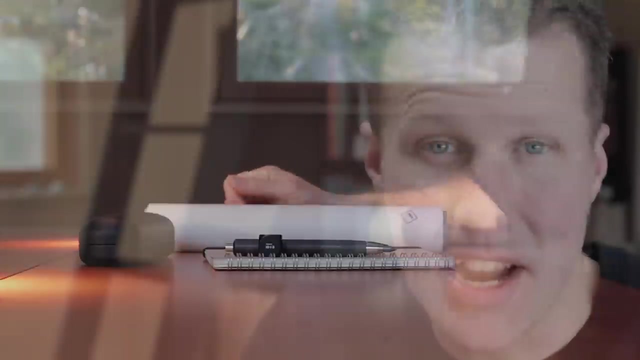 It's the questions we ask that will determine which problems our architecture will solve. Developing a concept allows us to frame the questions we're asking and it guides the design process. Choosing a starting point for your design can be intimidating and an early stumbling block for designers of any skill level, but it doesn't have to be Your concept. 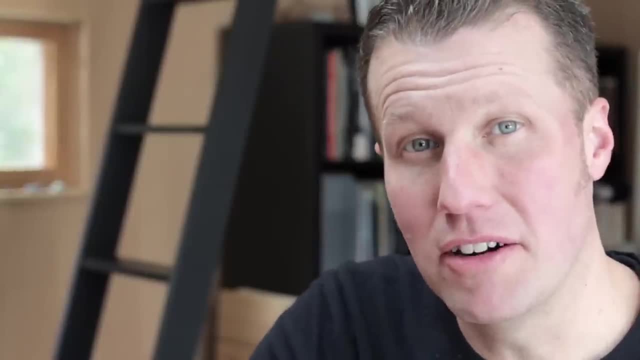 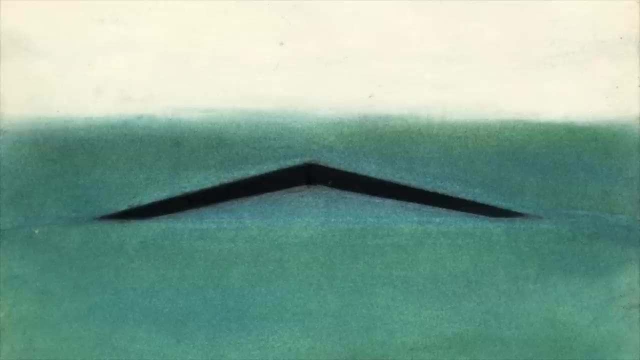 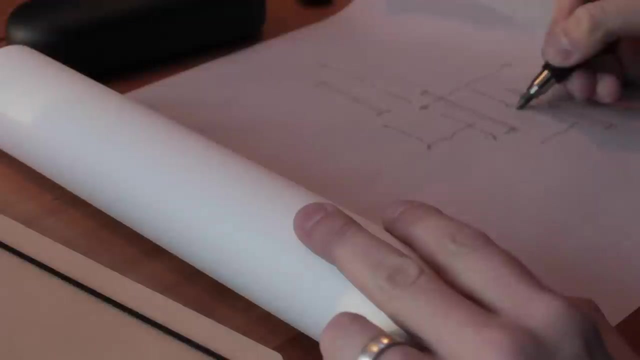 shouldn't be rigorous. The more malleable it is, the better. In fact, most architecture can't be reduced to one singular concept diagram. Rather, it's informed by many concepts working in concert. There may be organizational concepts, material concepts, functional or structural, or 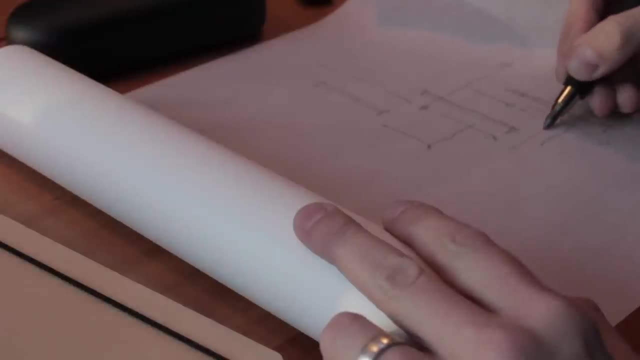 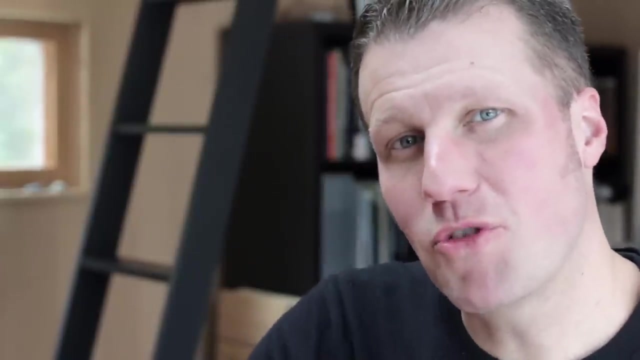 formal concepts. Don't fret if your idea isn't reducible to a single elegant black stroke on a page. It's best to illustrate concept development with a real project. As I said, we'll use our Squid Cove residence as an example. Before we can develop the concept, we first have to understand. 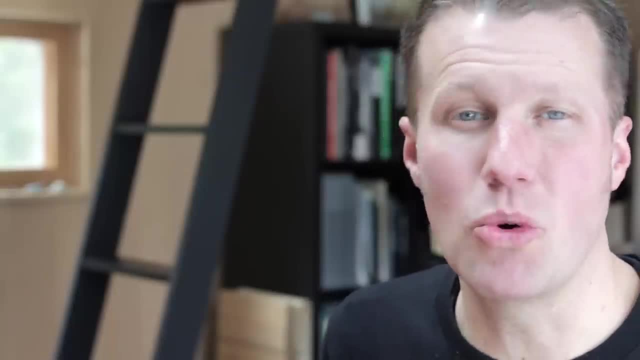 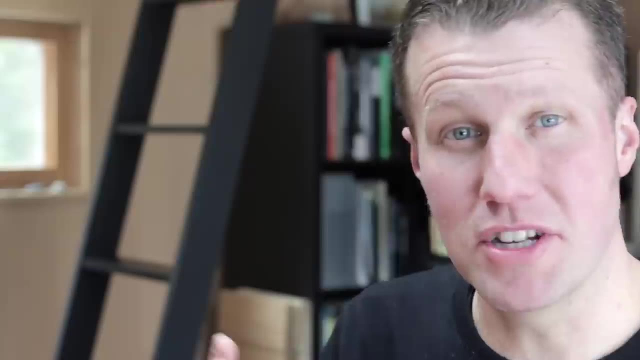 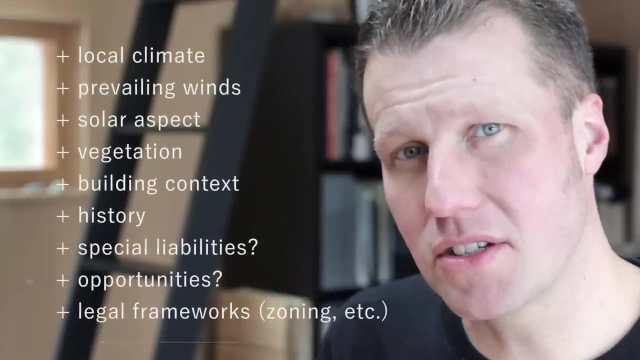 the practical constraints. My design process begins only after gathering and assessing all the given parameters for a project. This primarily consists of three types of information. There's information derived from the site: things like the local climate, the prevailing winds, the solar aspect, vegetation, neighboring structures, the site's history and any unique 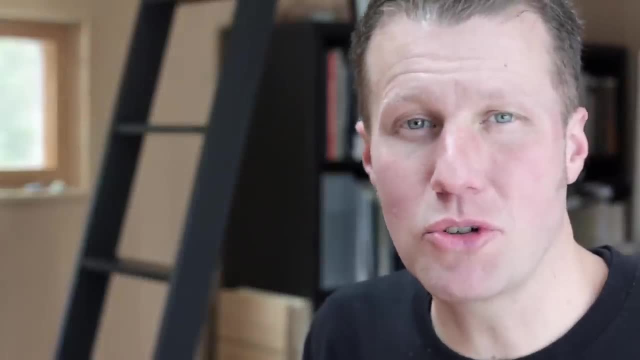 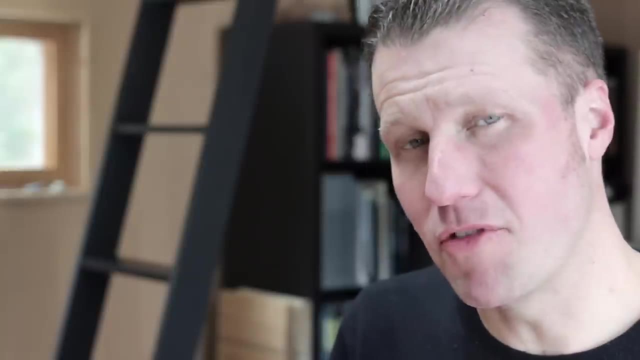 liabilities or opportunities. The site, of course, also comes along with legal frameworks for development which describe where and what we can and can't build. The second type of information we'll gather is from the client. Now, every client has a set of cultural beliefs and preconceptions. 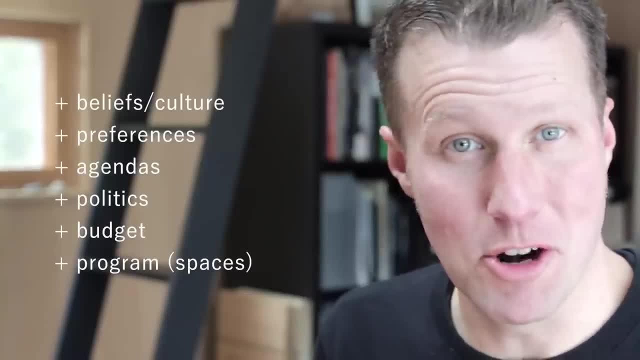 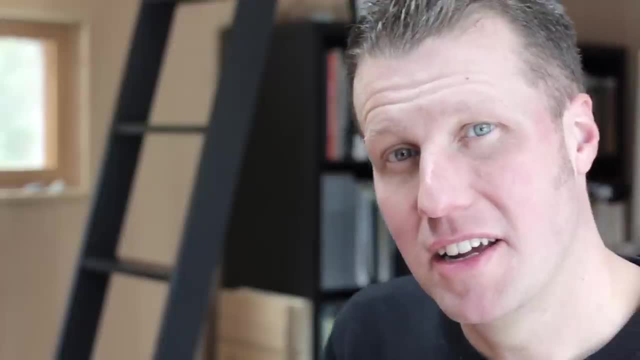 preferences and expectations. Each client has a set of cultural beliefs and preconceptions, preferences and agendas. Of course, we'll want to determine their budget and understand the personality, traits and organizational politics which might also shape the design, The client and the building type. 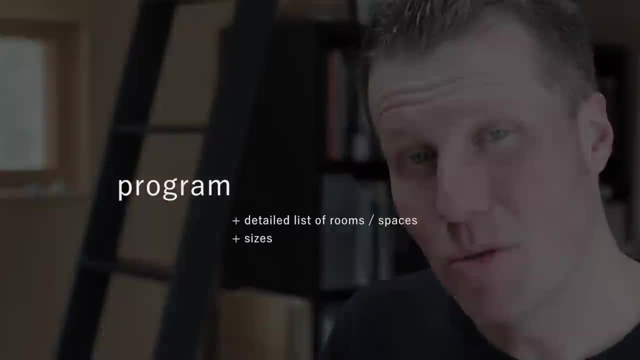 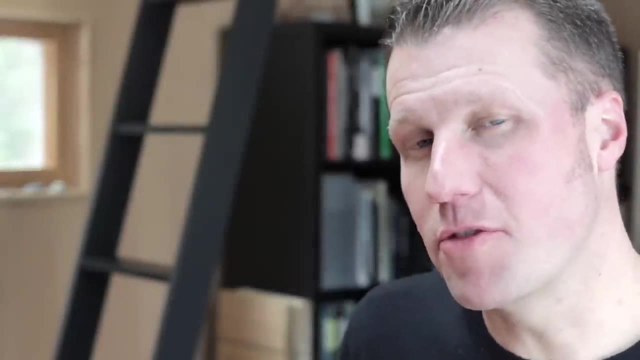 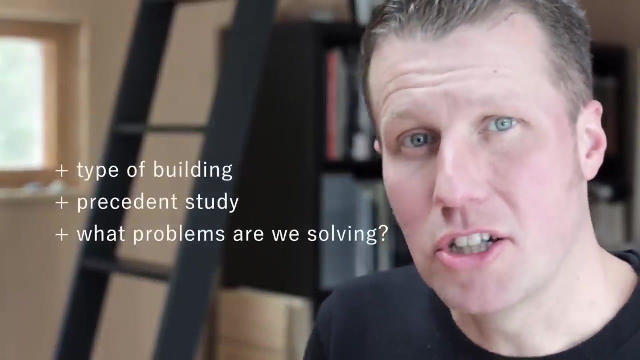 together determine what architects call the program, which is essentially a detailed accounting of all the spaces the building will contain. And the third type of information I gather is related to the building typology: Is it a museum, a home or a school To learn about a building type? 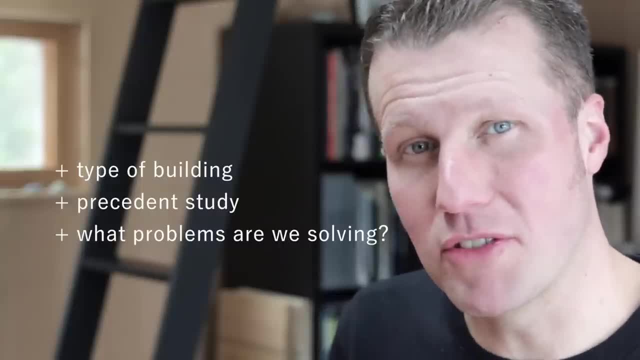 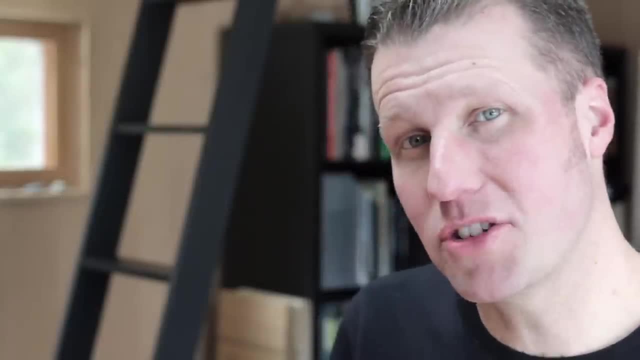 typology. we often conduct an analysis of notable or relevant historical precedents. We want to know the essential problems these type of structures grapple with. Understanding the history of the archetype allows us to approach a problem from a fresh perspective. Now, all of this necessary. 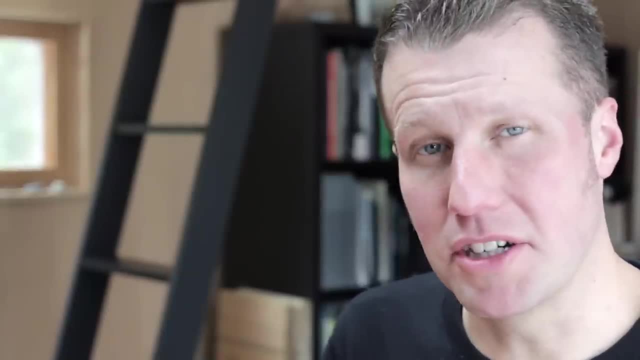 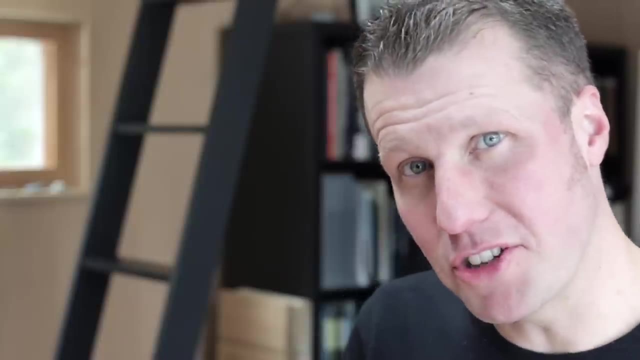 information. it's something that we collect for every single project. This inventory can also serve as the progenitor for the design concept, our seed idea. And, rather than shunting creativity, these constraints often incite the client to think about what they want to build and what they want to build. 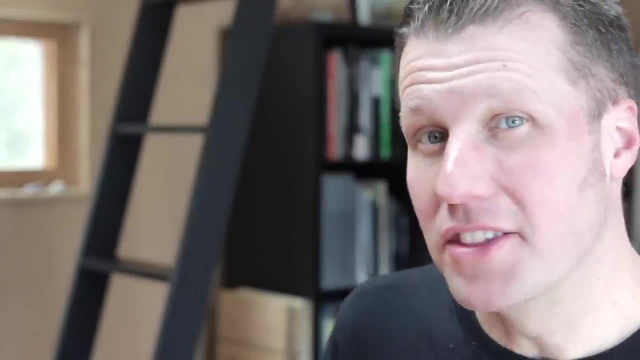 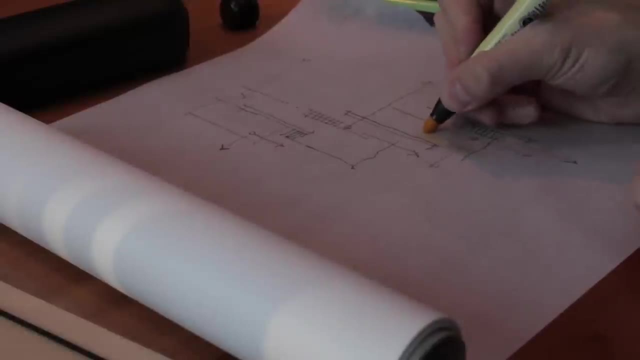 As with a good film, the setting, the characters, the cinematography and the plot all conspire to make it what it is. It's the experience, you'll recall, rather than the concept per se. Sure, the concept sets the film in motion and it's the starting point for all that follows. But this concept 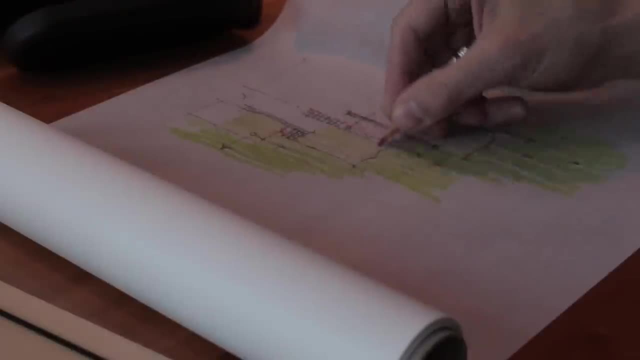 the one or two line description can't possibly capture the richness and depth of the finished film or, in our case, the architecture. Yet without it, the work is unfulfilling, and so it should be clear that the work is unfulfilling, and so it should be clear that the work is unfulfilling. 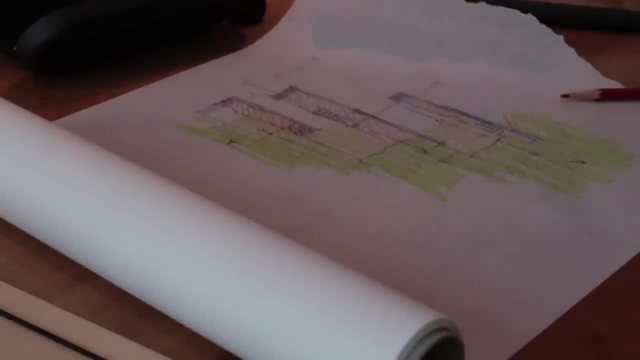 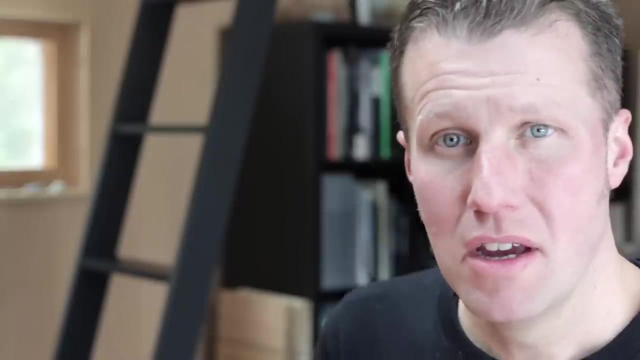 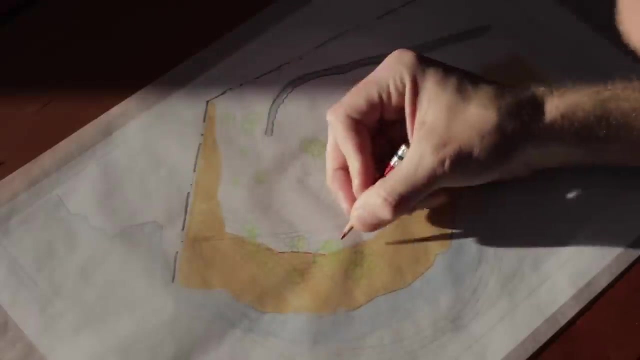 That the concept is necessary for all of our work as architects. Once we've gathered this information, it's now time to begin processing it into a usable form. Of the three, the site inventory is the most readily translated to a physical diagram For our Squid Cove project. you can see I've transcribed the zoning, the deed. 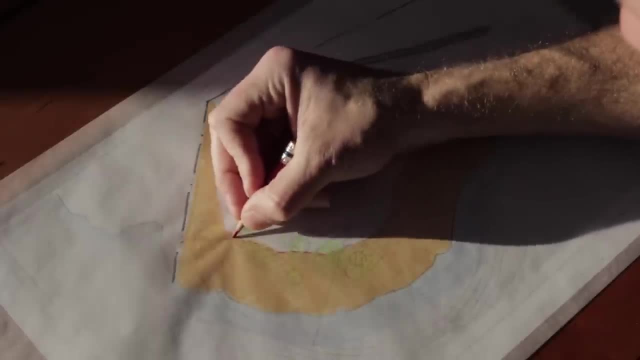 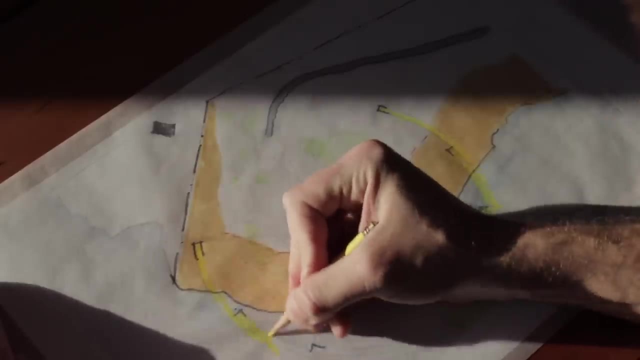 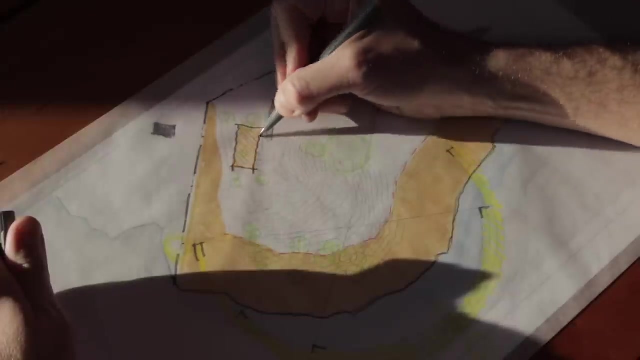 and setback information onto the site plan. This diagram sets the real boundaries of our project. We have property line setbacks, a setback from the ocean and an unstable bluff we need to avoid and this is shown on the topographical plan. There are a number of trees on the site and one significant ash that we're trying to avoid. 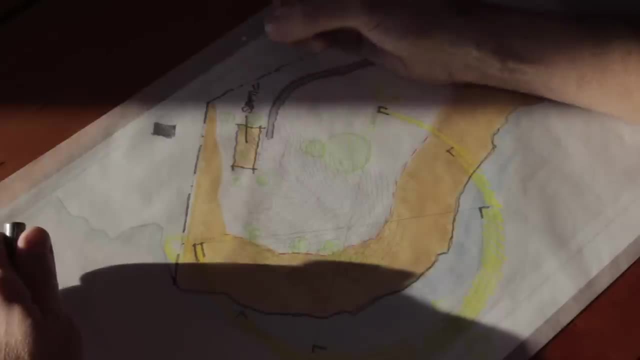 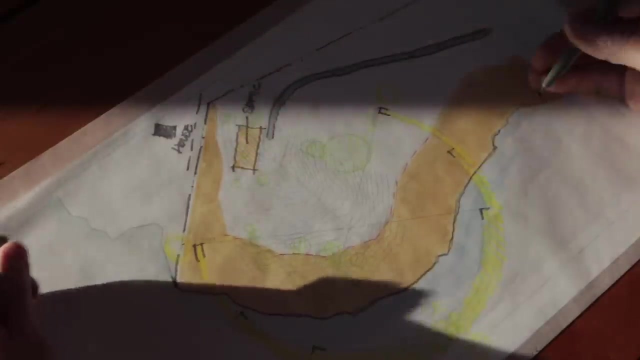 but for the most part the trees and vegetation here were just unremarkable. Next, I add to this the solar path, the prevailing wind direction and this amazing view. There are site utilities and an existing logging road, and because there's no public sewer here, I worked with a soil scientist to define the best spot for the septic field and consequently the well, which needs to be a certain distance away from the field. Now, this can often be a stringent limitation to the buildable area because there's so much. 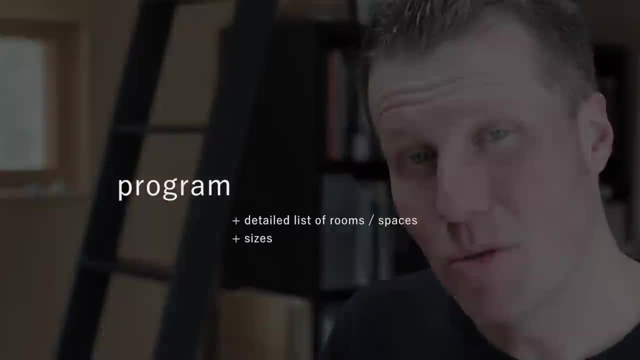 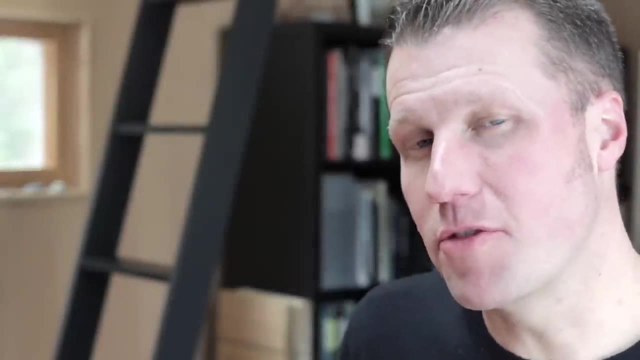 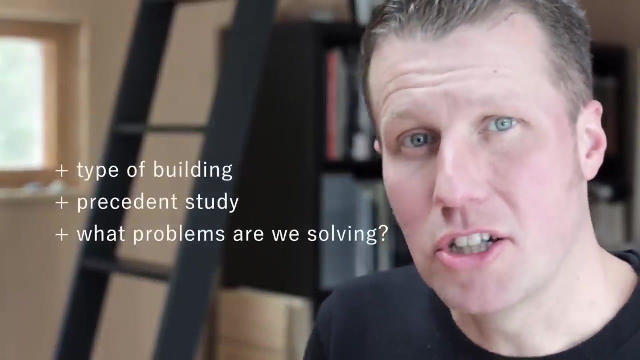 together determine what architects call the program, which is essentially a detailed accounting of all the spaces the building will contain. And the third type of information I gather is related to the building typology: Is it a museum, a home or a school To learn about a building type? 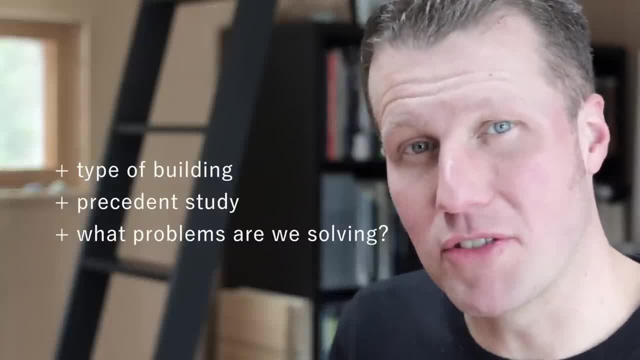 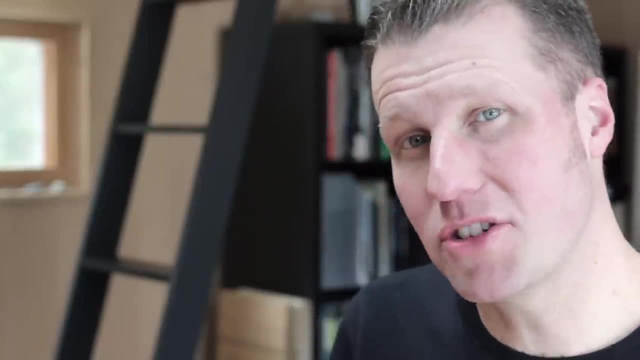 or a building typology. we often conduct an analysis of notable or relevant historical precedents. We want to know the essential problems these type of structures grapple with. Understanding the history of the archetype allows us to approach a problem from a fresh perspective. Now, all of this necessary. 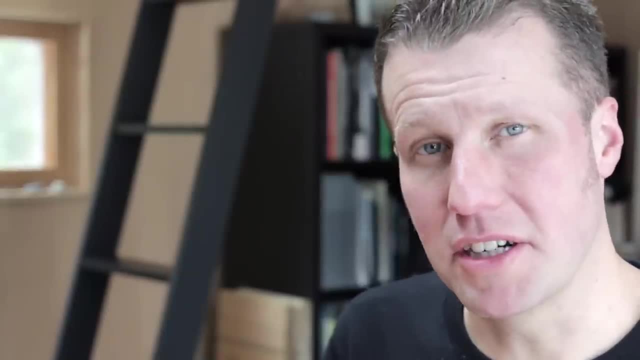 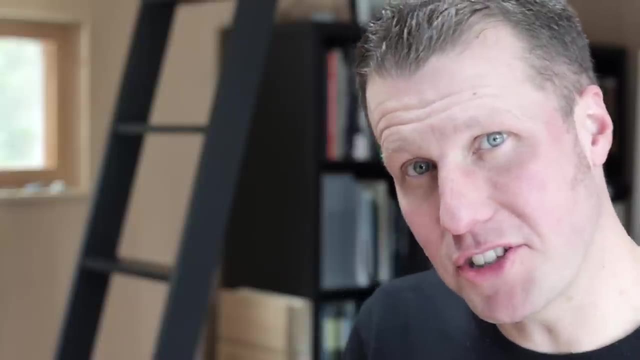 information. it's something that we collect for every single project. This inventory can also serve as the progenitor for the design concept, our seed idea. And, rather than shunting creativity, these constraints often incite the project. and this is what we're trying to do. We're trying to create a 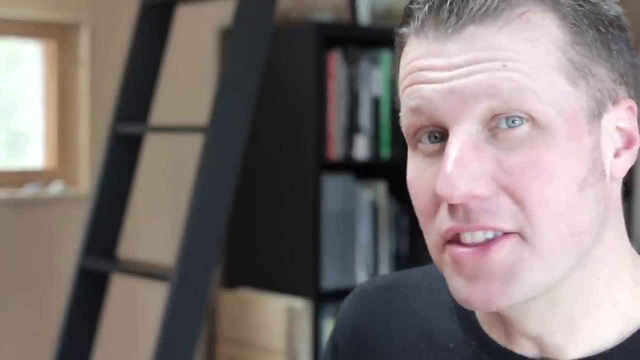 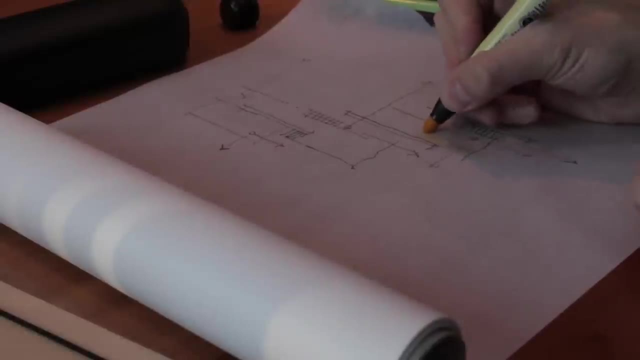 insight, the creative process- As with a good film, the setting, the characters, the cinematography and the plot all conspire to make it what it is. It's the experience you'll recall, rather than the concept per se. Sure, the concept sets the film in motion and it's the starting point for all. 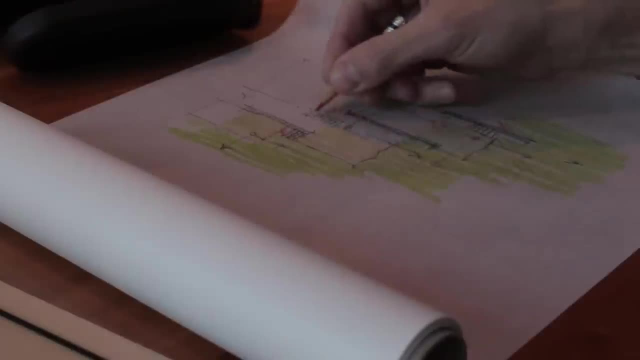 that follows. but this concept, the one or two line description, can't possibly capture the richness and depth of the finished film, or, in our case, the architecture. Yet without it the work is unfulfilling, and so it should be clear that the concept is necessary for all of our work, as 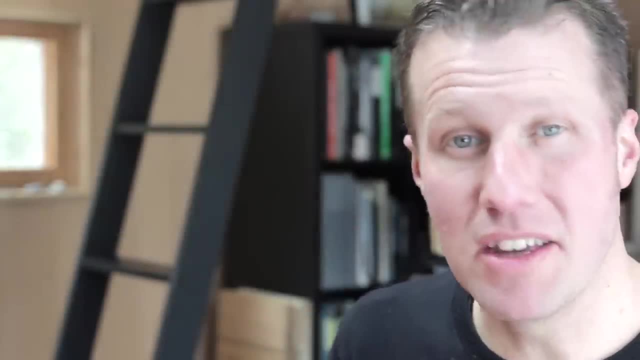 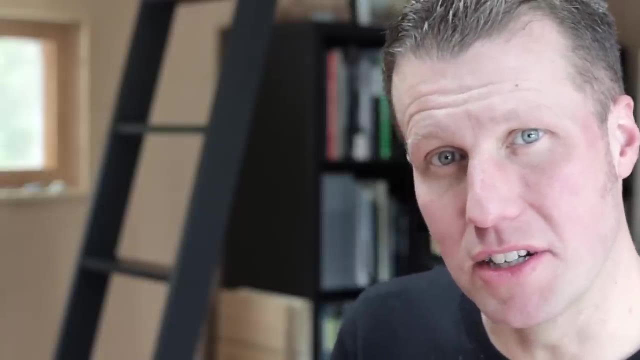 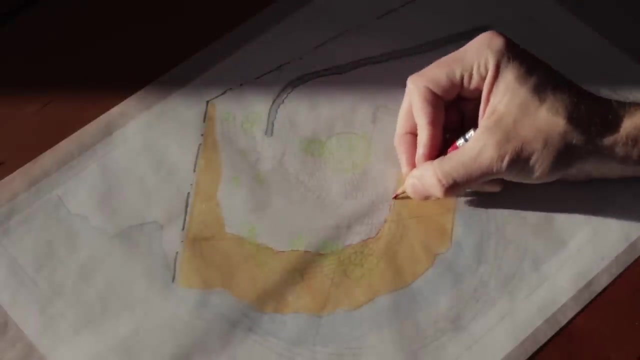 architects. Once we've gathered this information, it's now time to begin processing it into a usable form. Of the three, the site inventory is the most readily translated to a physical diagram. For our Squid Cove project. you can see I've transcribed the zoning, the deed and setback. 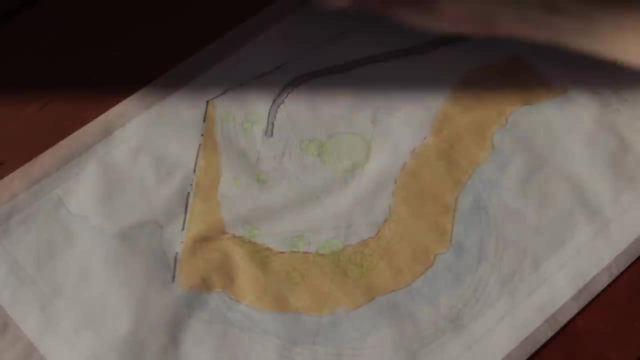 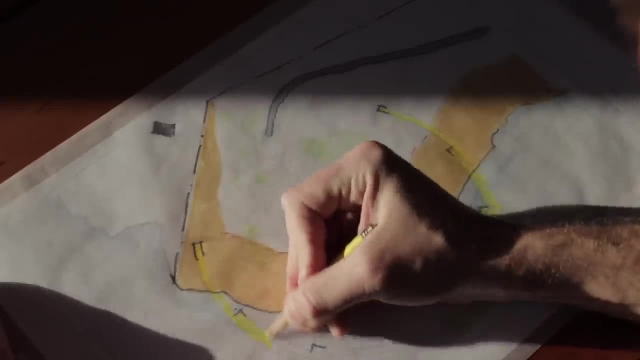 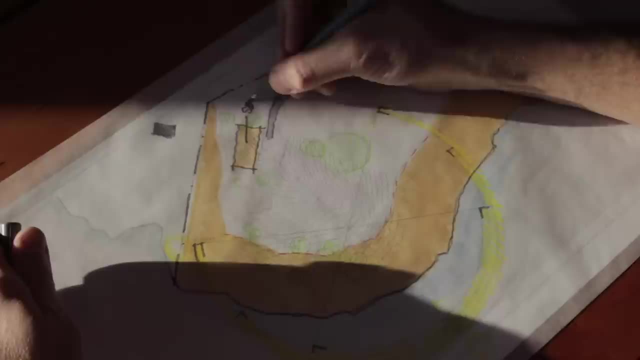 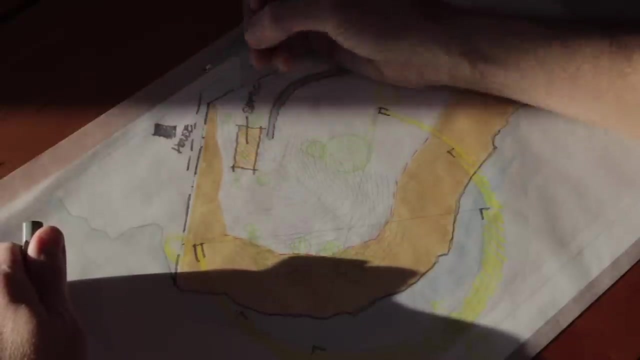 ash that we're trying to avoid, but for the most part, the trees and vegetation here were just unremarkable. Next, I add to this the solar path, the prevailing wind direction and this amazing view. There are site utilities and an existing logging road. 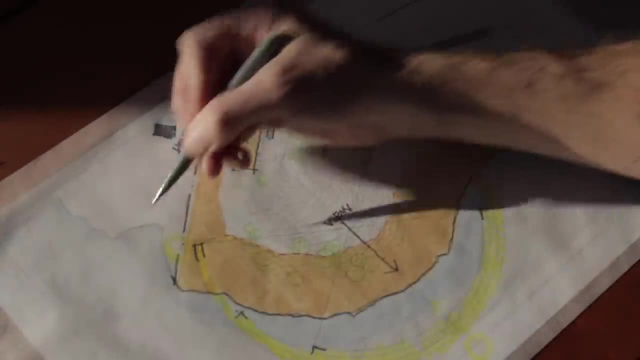 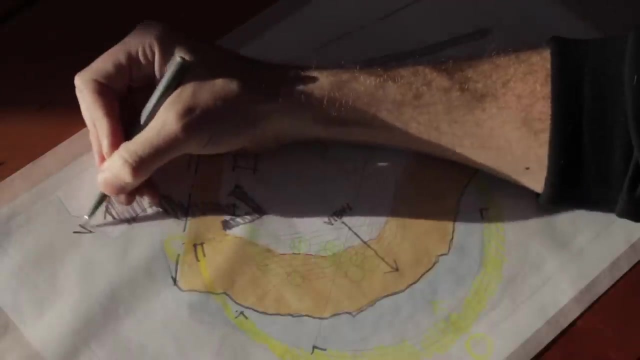 and because there's no public sewer here, I worked with a soil scientist to define the best spot for the septic field and consequently the well, which needs to be a certain distance away from the field. Now, this can often be a stringent limitation to the buildable area. 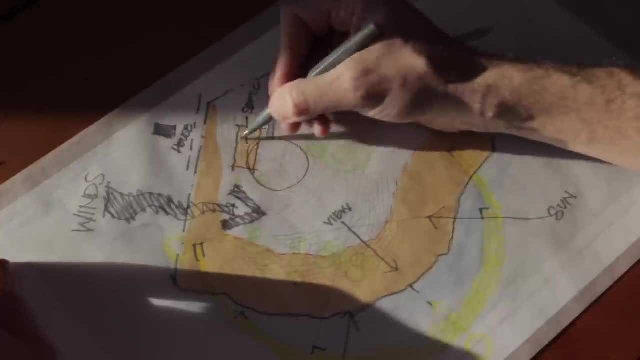 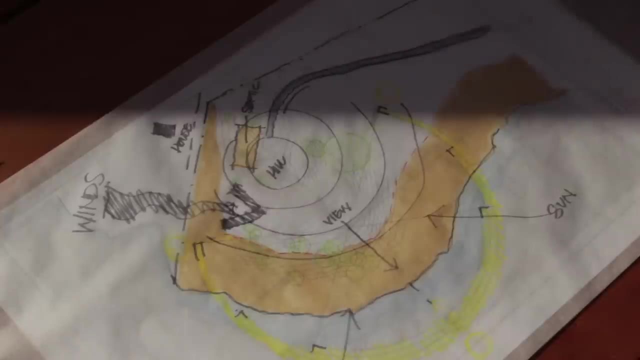 because there's so much granite locally, so it's important for me to define it early, and the one last piece of information is that there's a neighboring house here that we want to avoid looking at. Now I like to diagram these constraints on the site plan before I visit the 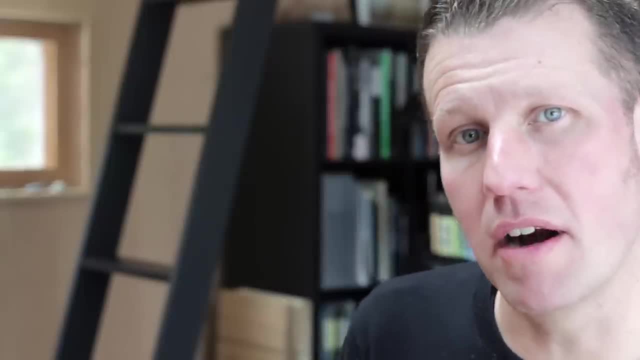 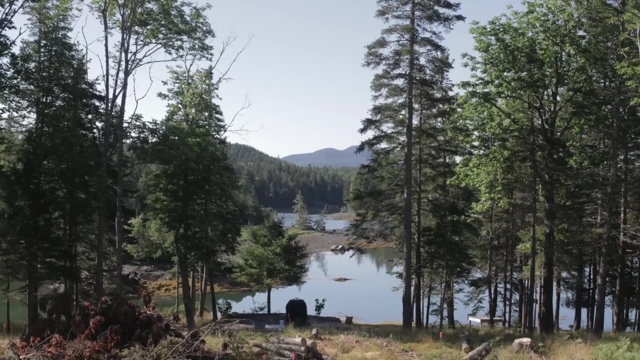 site, so the information becomes a part of how I see things when I'm there. Visiting the site, of course, will leave a different impression, and I find mapping things out first allows me to overlay the two in a way that selects for opportunity. Now that we have this diagram, 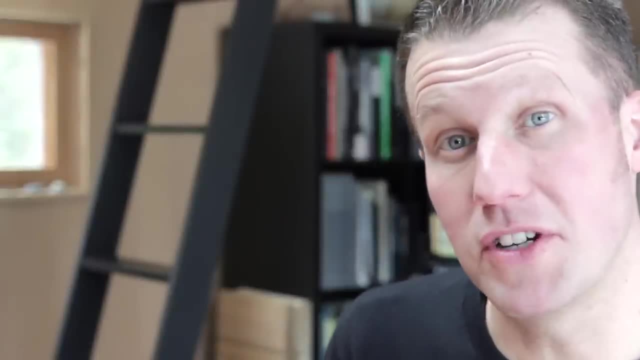 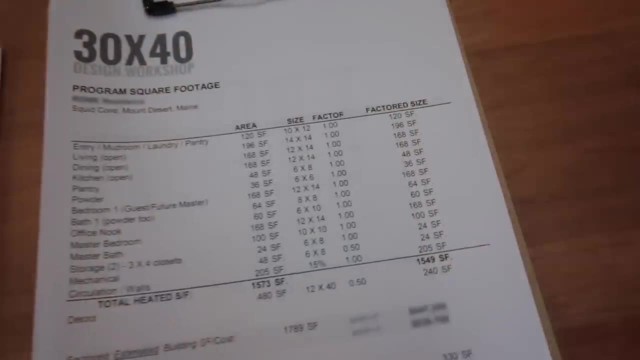 we can start to see the buildable site. Still quite a bit of territory. This video won't cover the programming phase. we'll save that for another one, but prior to this I've worked with a client to define the size of the home and the budget, which are, as you'd imagine, strongly interrelated. 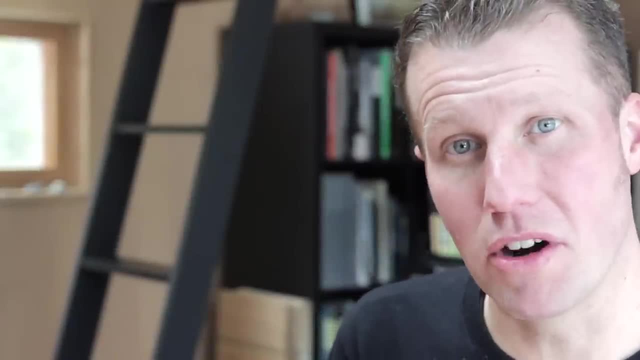 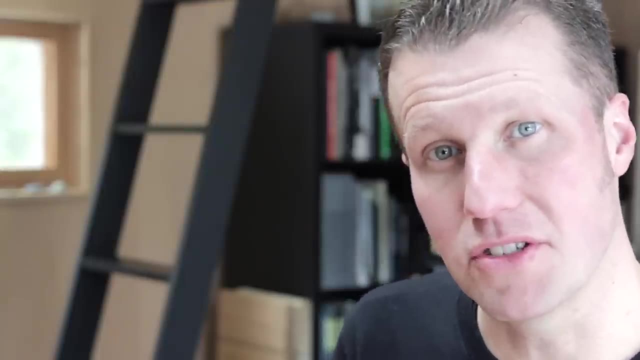 There's no sense in beginning any design work until you're done with the design work and, if you're done with the design work, until the client is aware of the rough cost of the work which, at this stage, is directly tied to their wish list of spaces and the sizes of those spaces. So, having completed, 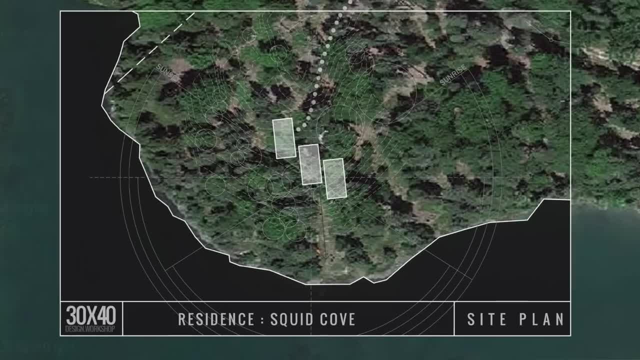 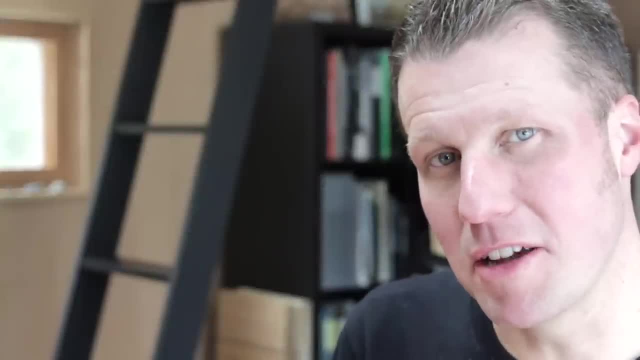 the programming exercise, I can now diagram the relative size of the home and overlay that on the site when the time is right. Because I work solely on residential projects, I'm quite familiar with the building type. so I'm not doing an exhaustive precedent study for each project, but knowing the 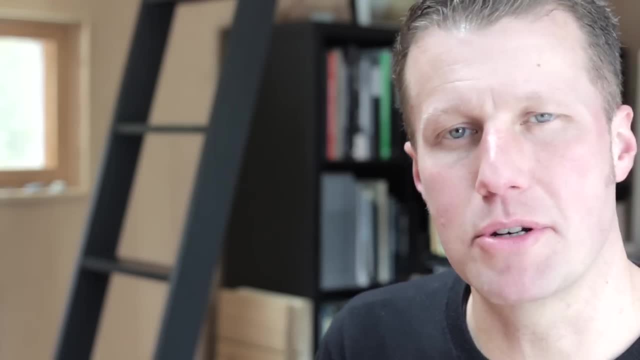 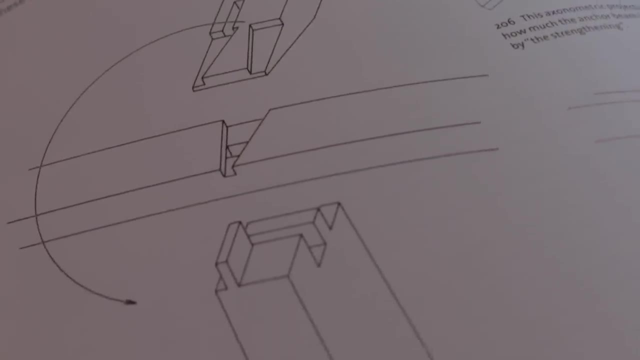 typology allows me to reinvent and rethink things that I'm not familiar with, So I'm going to start from where I was when I saw an opportunity. If I were working on a building typology I was unfamiliar with, I'd research the building precedence and use that information as an underlying framework for 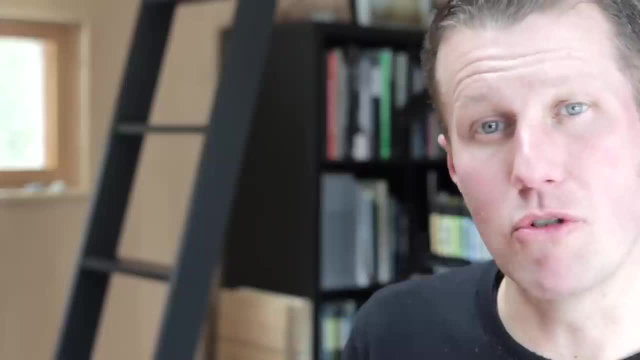 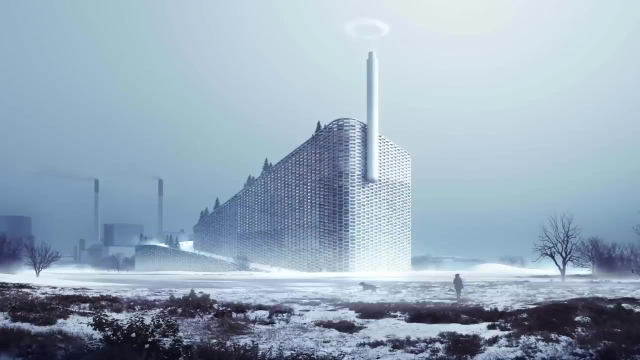 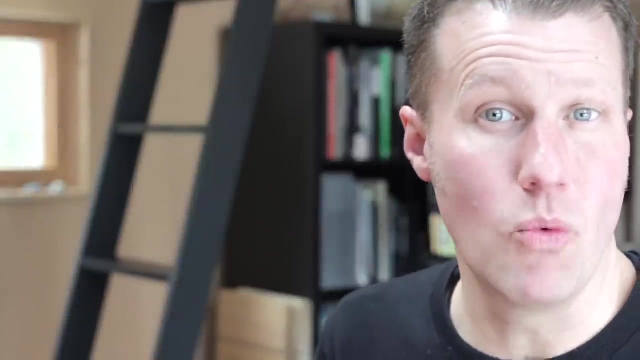 developing the program and possibly as a launching point for my concept. Now you should look at the work of Bjarki Ingels as a contemporary example of someone who uses typological reinvention to inspire his building concepts. So we visited the site and we know what and where we can. 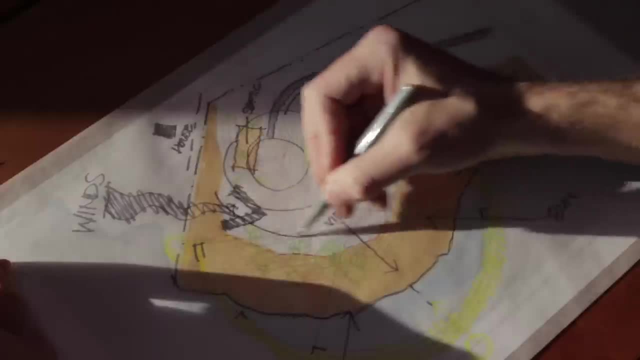 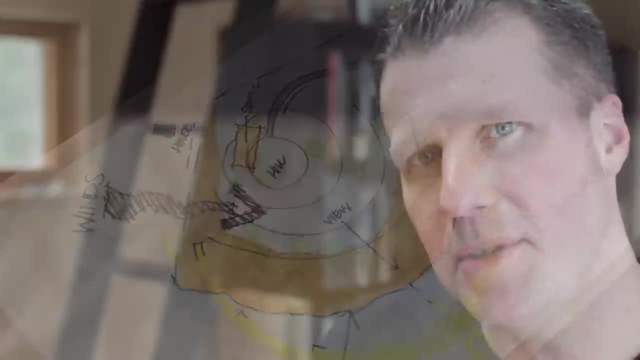 granite locally, so it's important for me to define it early. And the one last piece of information is that there's a neighboring house here that we want to avoid looking at. Now I like to diagram these constraints on the site plan before I visit the site. 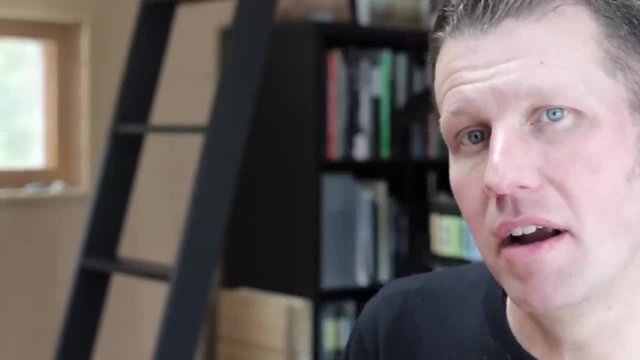 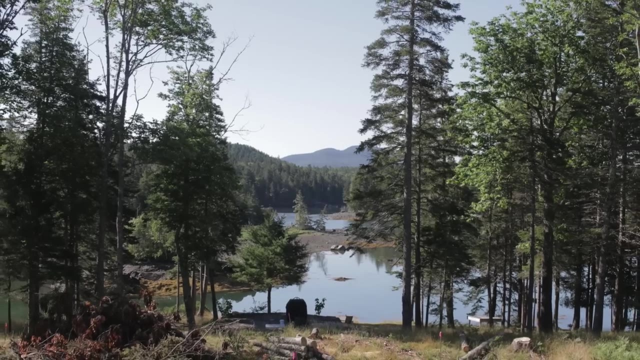 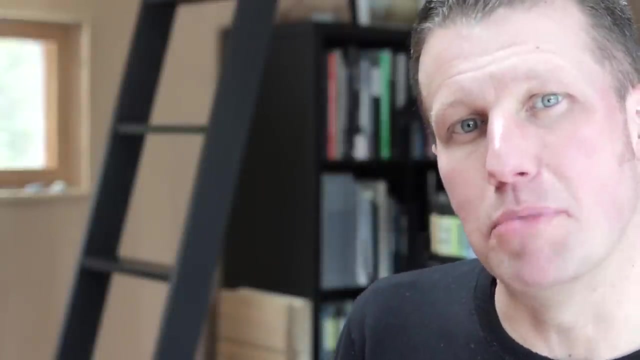 so the information becomes a part of how I see things when I'm there. Visiting the site, of course, will leave a different impression, but I find mapping things out first allows me to overlay the two in a way that selects for opportunity. Now that we have this diagram, we can start to see the buildable site Still. 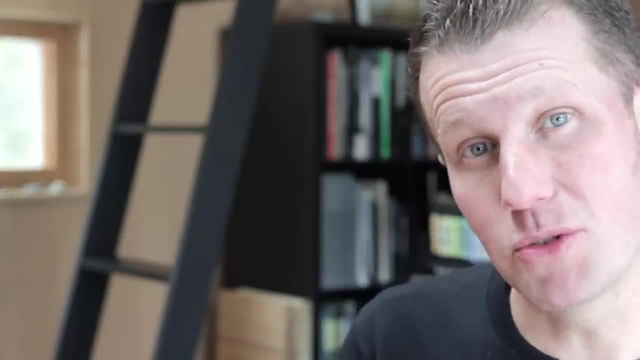 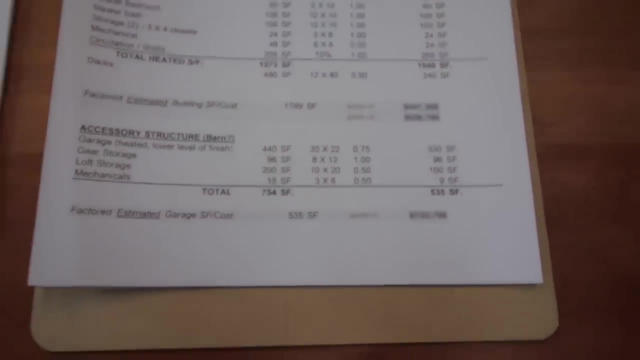 quite a bit of territory. This video won't cover the programming phase. we'll save that for another one. but prior to this I've worked with a client to define the size of the home and the budget, which are, as you'd imagine, strongly interrelated. There's no sense in beginning any design work. 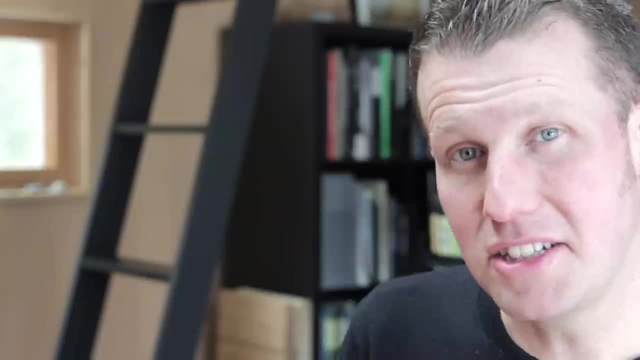 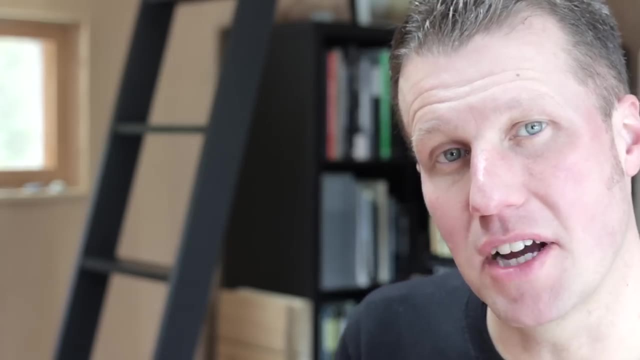 until the client is aware of the rough cost of the work, which, at this stage, is directly tied to their wish list of spaces and the sizes of those spaces. So, having completed the programming exercise, I can now diagram the relative size of the home. 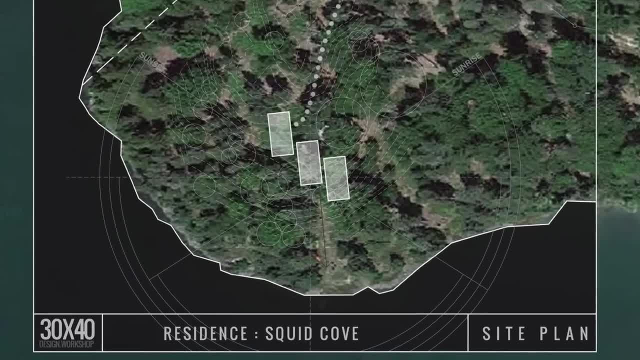 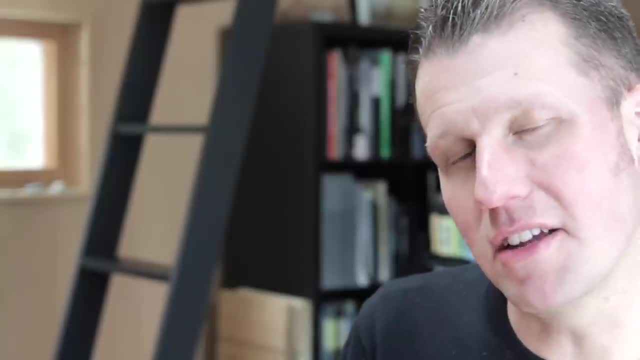 and overlay that on the site when the time is right. Because I work solely on residential projects, I'm quite familiar with the building type. so I'm not doing an exhaustive precedent study for each project, But knowing the typology allows me to reinvent and rethink things when I 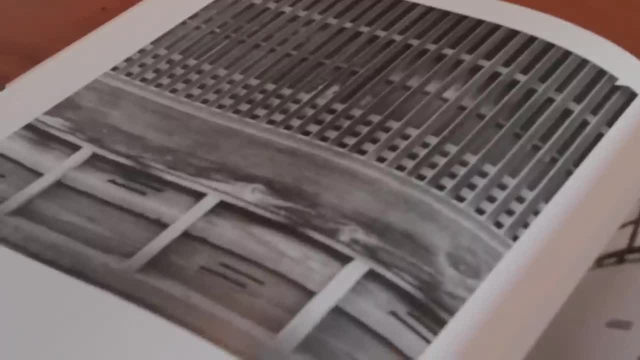 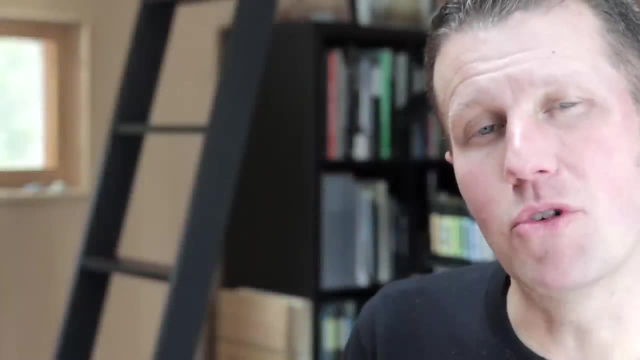 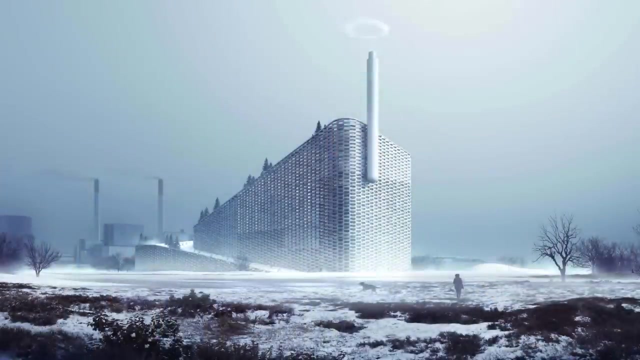 see an opportunity If I were working on a building typology I was unfamiliar with. I'd research the building precedents and use that information as an underlying framework for developing the program and possibly as a launching point for my concept. Now you should look at the work of Bjarki Ingles. 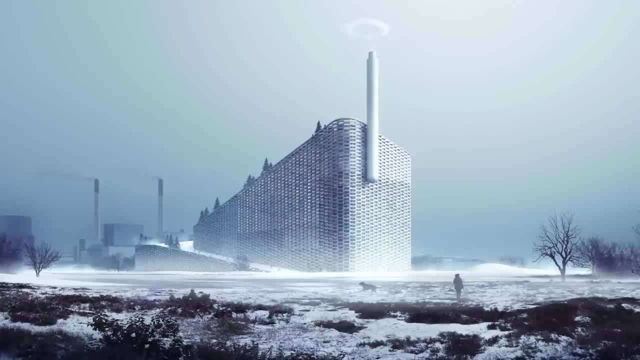 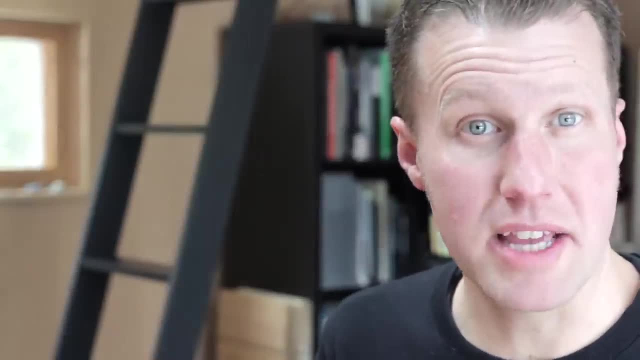 as a contemporary example of someone who uses typological reinvention to inspire his building concepts. So we've visited the site and we know what and where we can and can't build, we know type and we know our client has budgeted for the design we're about to undertake. 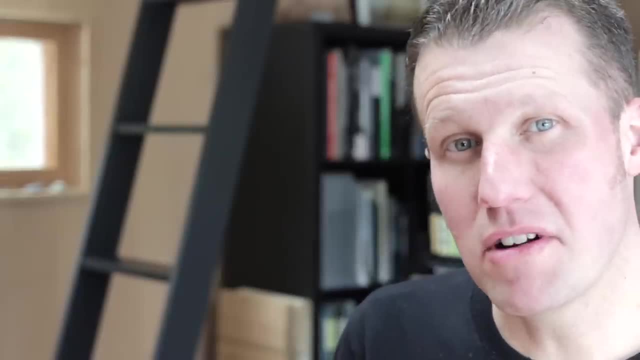 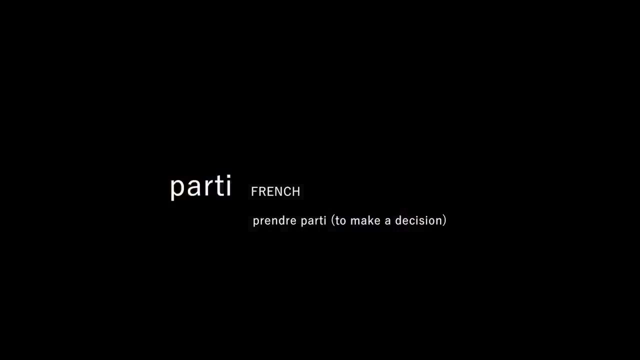 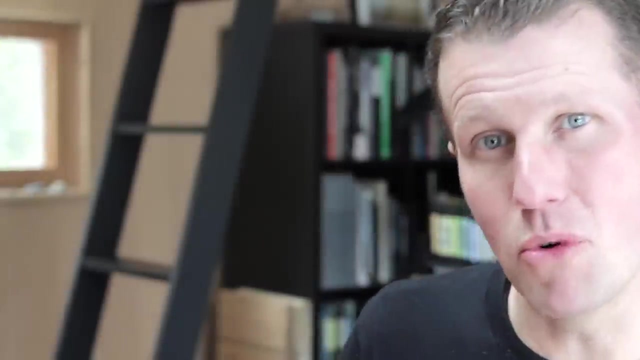 What's next? Well, this is where the building concept, or parti, comes in. Parti is sort of architect lingo for concept, and it actually comes from the French prendre parti, which means to make a decision. It's the organizing principle we use as a starting point for the design. Now I've come up with a few of. 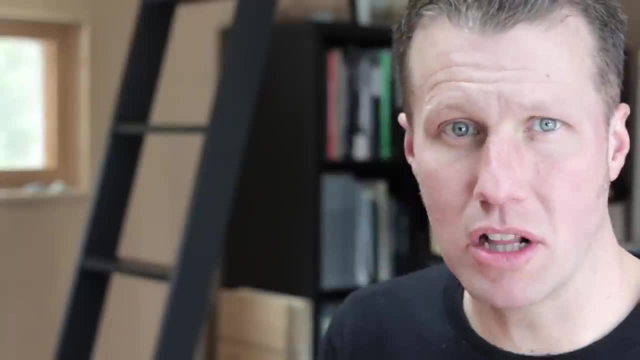 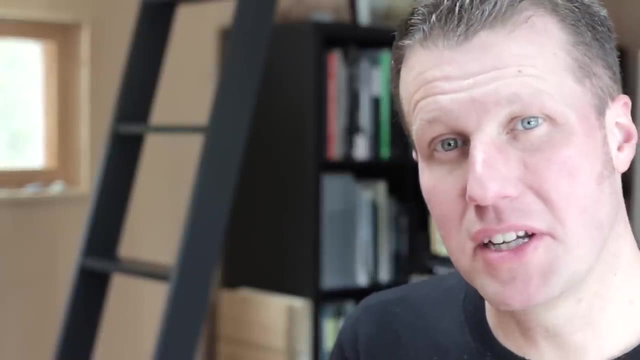 can and can't build. We know something about the building type and we know our client has budgeted for the design we're about to undertake. What's next? Well, this is where the building concept, or parti, comes in. Parti is sort of architect lingo for concept, and it actually 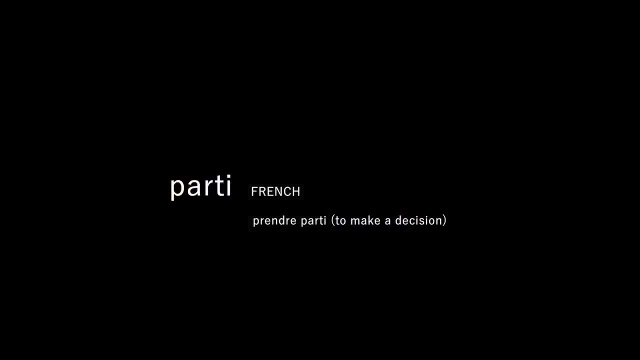 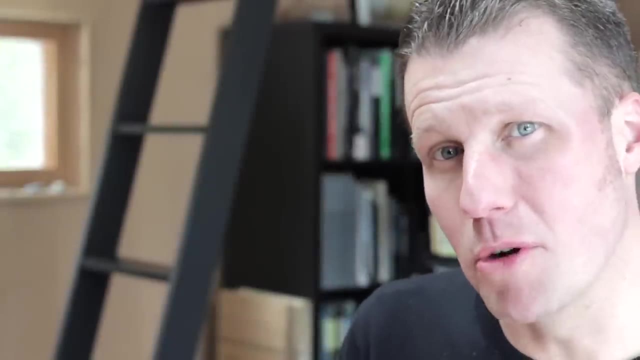 comes from the French prendre parti, which means to make a decision. It's the organizing principle we use as a starting point for the design. Now I've come up with a few of the most common ones I rely on to spark ideas, but there are an infinite number available to you. We'll start. 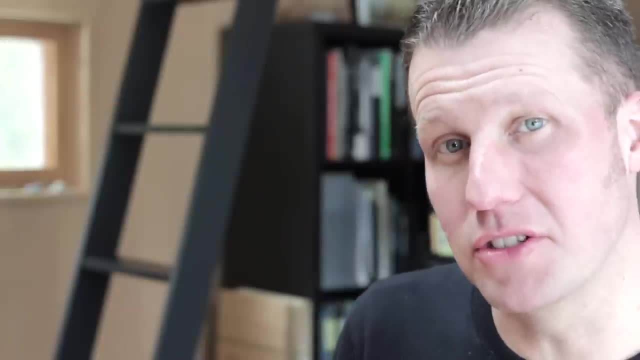 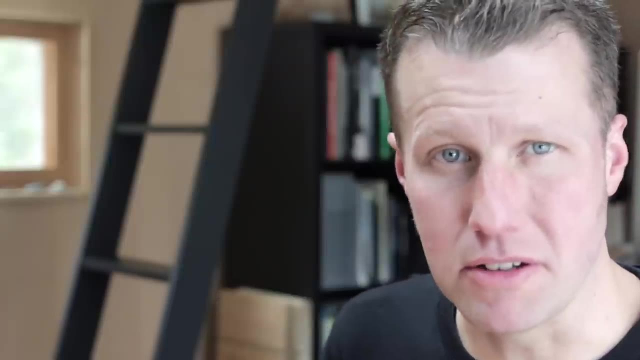 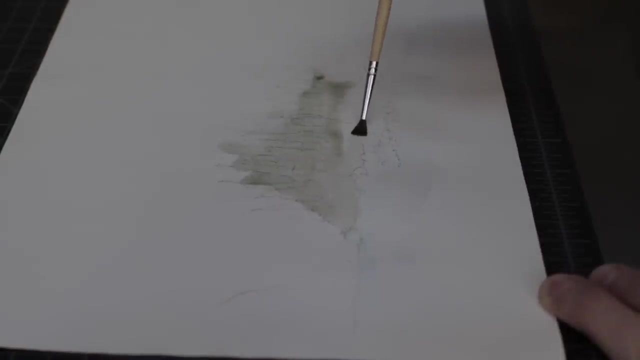 with the simplest, and it's one we've already touched on in our initial information gathering phase. Buildings interpret their surroundings and reformulate them in a way that can be experienced. The site demands specificity from our architecture. It must react to it. so, using the site to inspire. 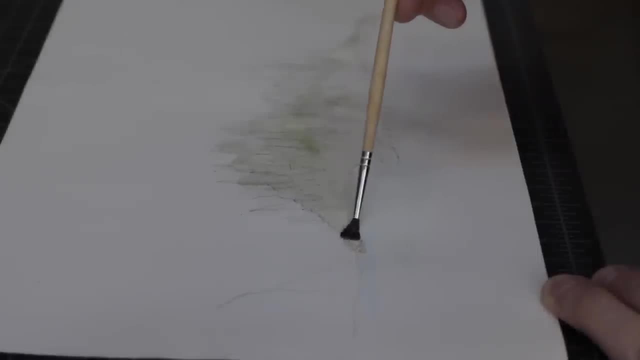 the building concept is as genuine a place to start as any. We can react to views, light, topography, history and the like. We can react to the site's design and we can react to the design. We can react to the site's design and we can react to the site's design. We can react to the 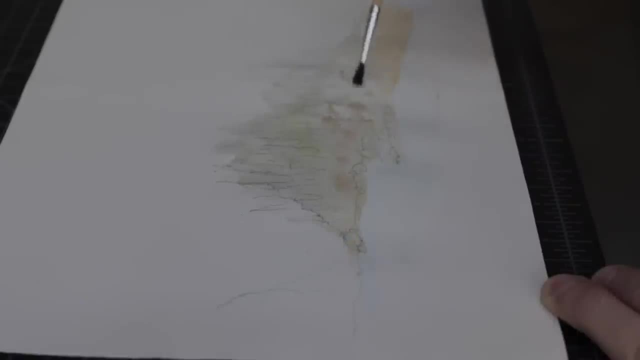 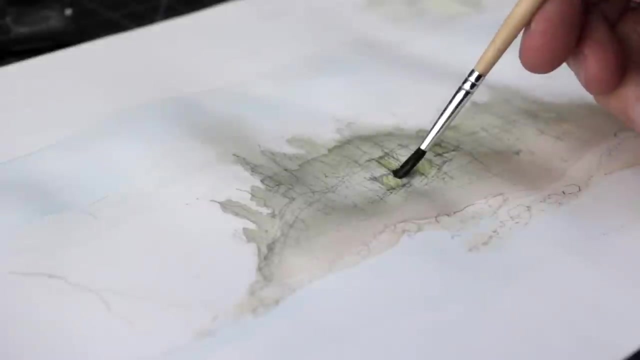 historical features, vegetation and other structures. When a building concept references a site in a rural setting, it establishes a dialogue between natural and man-made In urban and suburban contexts, a boundary between what you can design and control and what you can't. 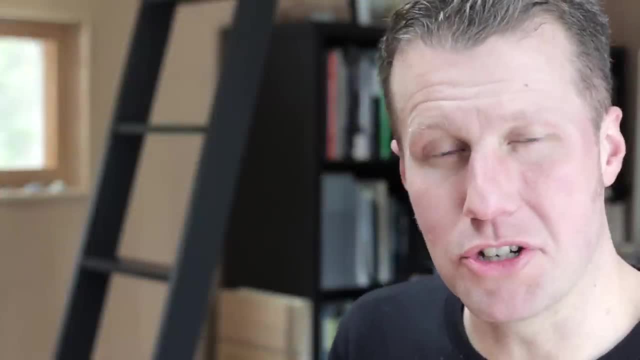 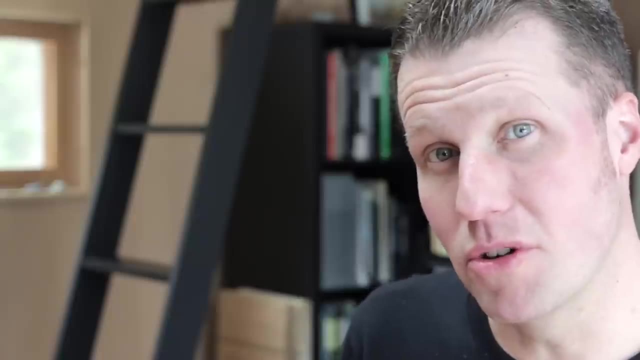 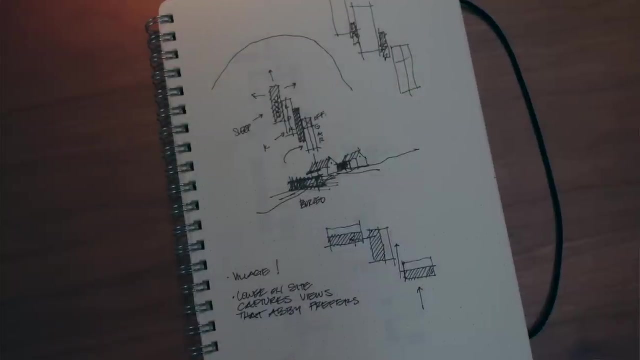 Your design inspiration can editorialize this relationship. Will it oppose nature or the local surroundings or complement it? Will it disregard it or adapt to it? Will it impose order on it Or will it assume a different order? For our project, the site was an important progenitor of 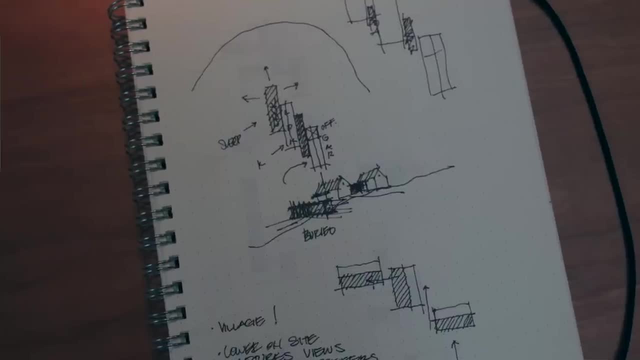 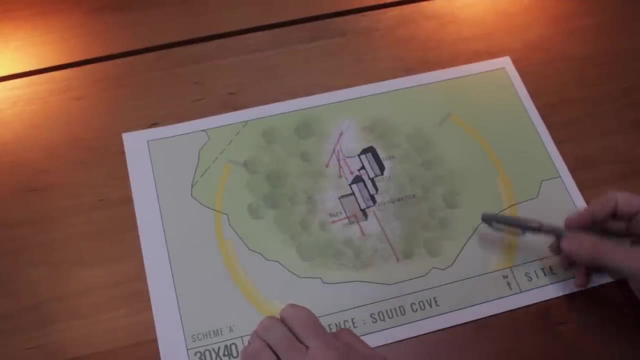 the design concept, It was important for me to work with the landform and exploit the natural slope. Of equal importance were the view to the water and the solar aspect, each of which became strong organizing forces that shaped our early building massings. I imagined one arriving to: 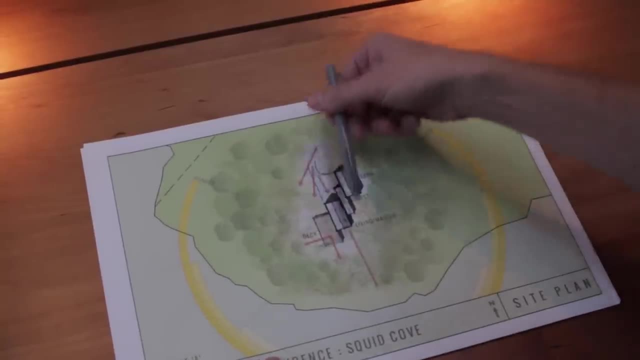 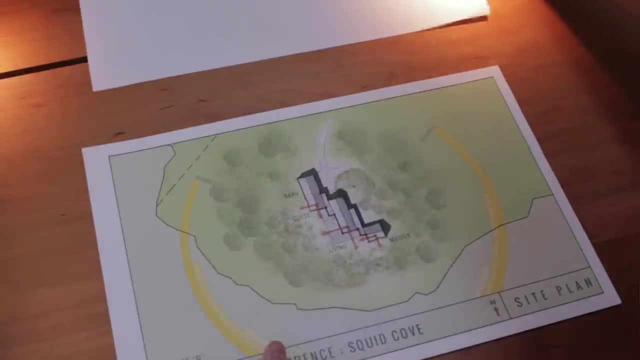 the site and being presented with the view beyond rather than the building. So I knew I wanted to work on the hillside rather than on the crest of the hill. The sloping landform presented an opportunity to mimic that with the form of the house, and I began thinking of ways to zone the 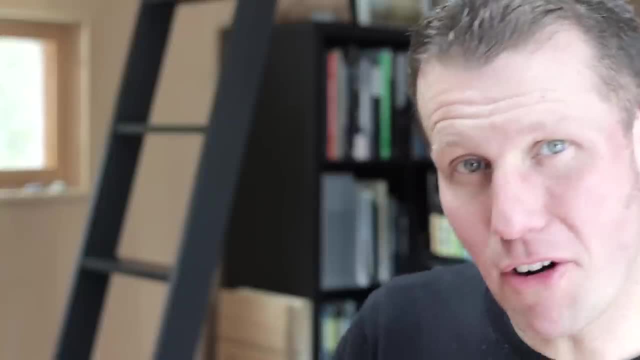 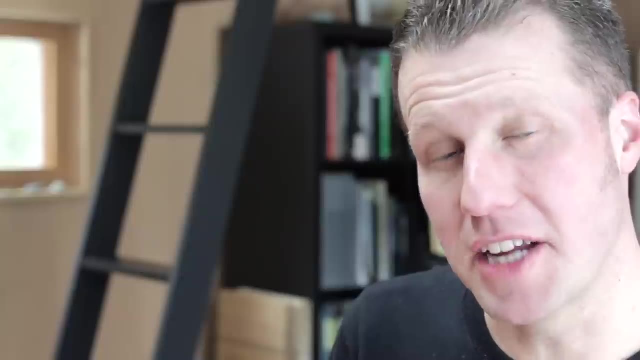 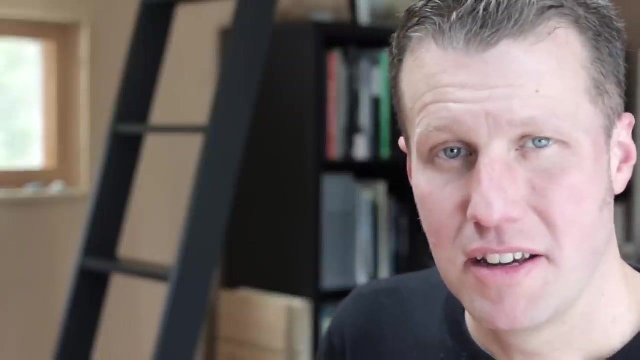 the most common ones I rely on to spark ideas, but there are an infinite number available to you. We'll start with the simplest, and it's one we've already touched on in our initial information gathering phase. Buildings interpret their surroundings and reformulate them in a way that can be experienced. The 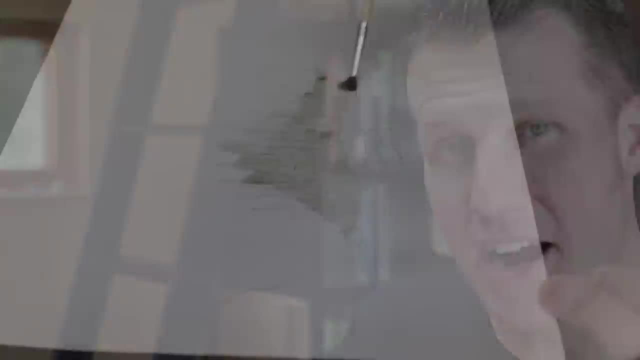 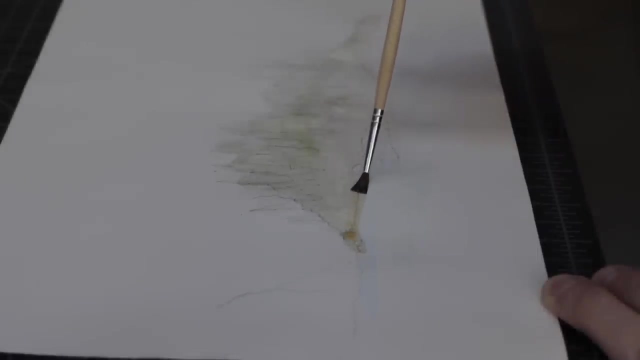 site demands specificity from our architecture. It must react to it. so using the site to inspire the building concept is as genuine a place to start as any. We can react to views, light, topography, historical features, vegetation and other structures. When a building concept references a site in a rural setting, it establishes a 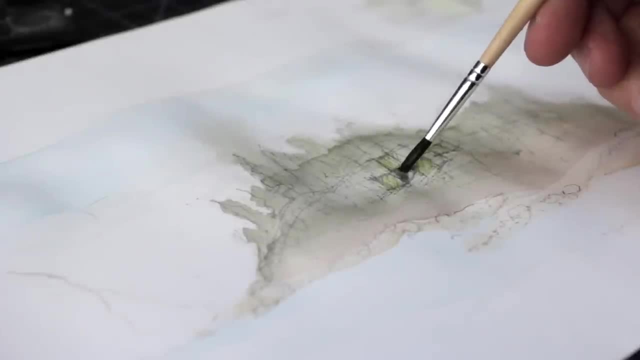 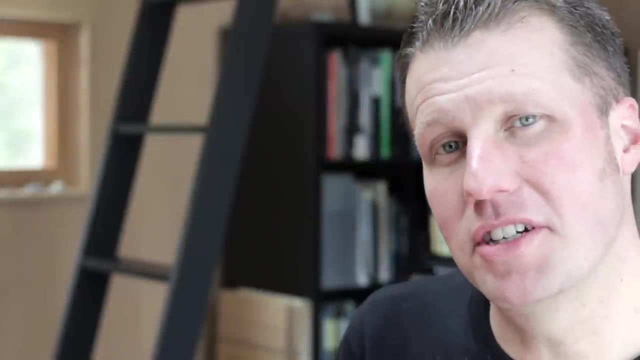 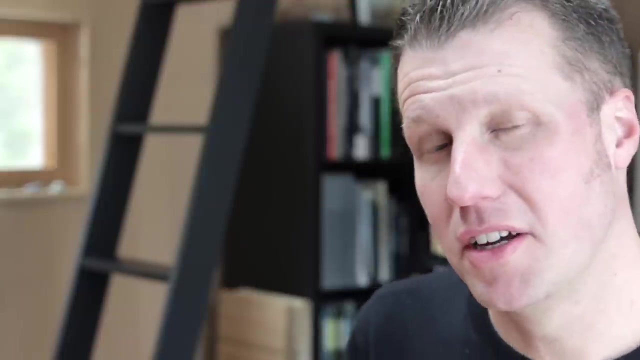 dialogue between natural and man-made In urban and suburban contexts, a boundary between what you can design and control and what you can't. Your design inspiration can editorialize this relationship. Will it oppose nature or the local surroundings or complement it? Will it disregard it or adapt to it? Will it? 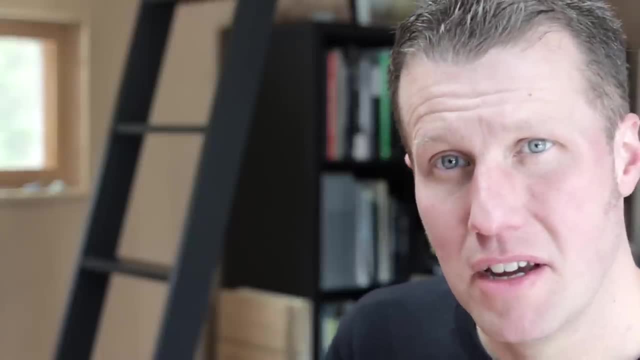 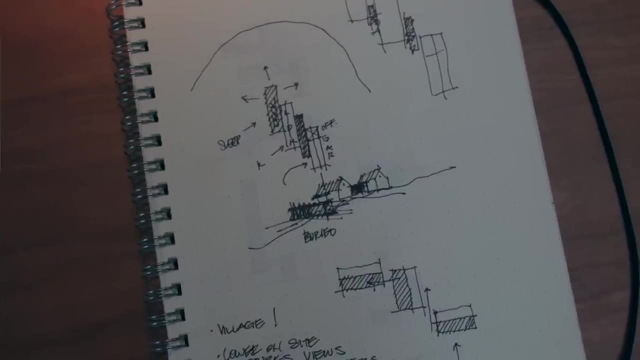 impose order on it, or will it assume a different order? For our project, the site was an important progenitor of the design concept. It was important for me to work with the landform and exploit the natural slope. Of equal importance were the view to the water and the solar aspect, each of which 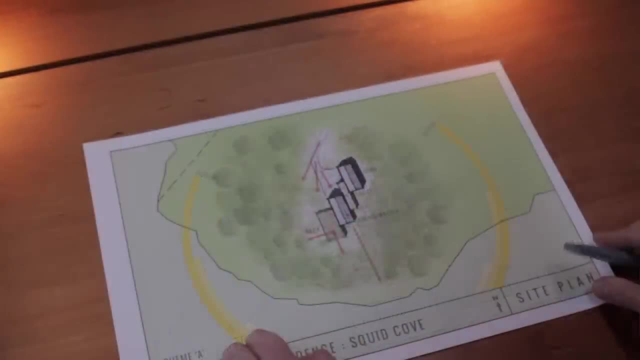 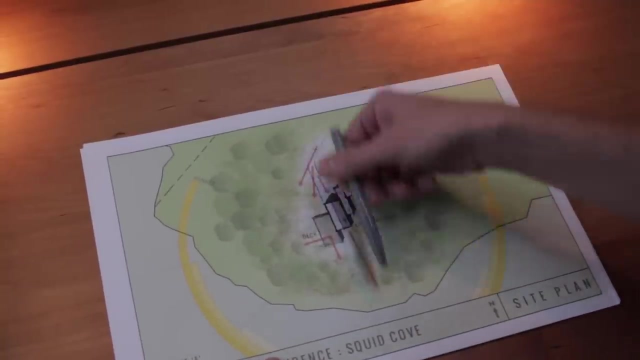 became strong organizing forces that shaped our early building massings. I imagined one arriving to the site and being presented with the view beyond rather than the buildings, So I knew I wanted to cite the home to the south, splayed out along the hillside rather than on the crest of the hill, The 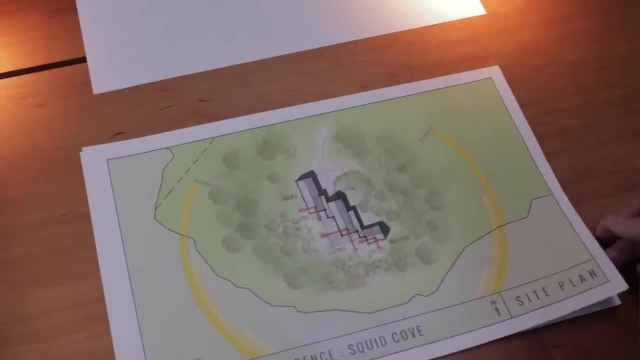 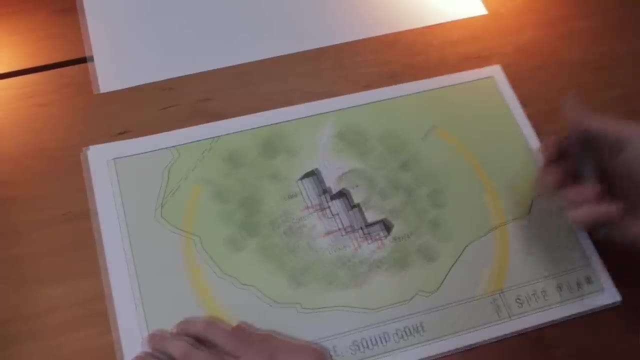 sloping landform presented an opportunity to mimic that with the form of the house, and I began thinking of ways to zone the organization of the building to complement the site features too. I used the view to the cove as well as the solar aspect to select the most desirable site for the home. Now, often, 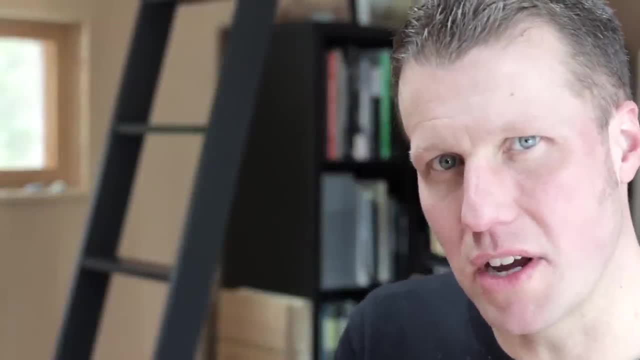 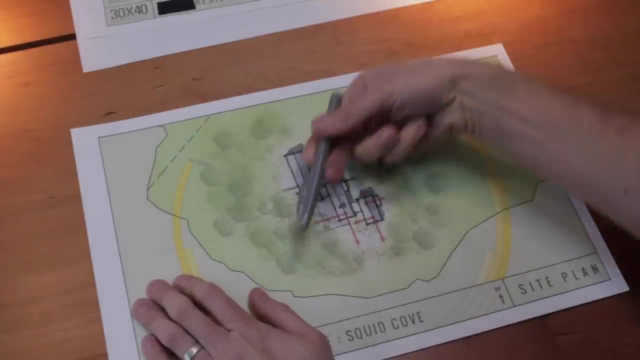 competing site factors will force you to choose one site force as more dominant. For example, the prevailing wind direction is in the direct competition with the idea I had about arrival to the site. If we were to look at the home instead of the view to the coast, I would choose to go to the south bend. For example, the prevailing wind direction is in the direct competition with the idea I had about arrival to the site. If we were to compare the site to the north bend, the 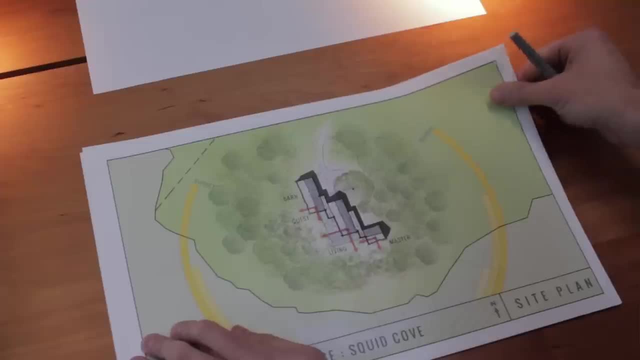 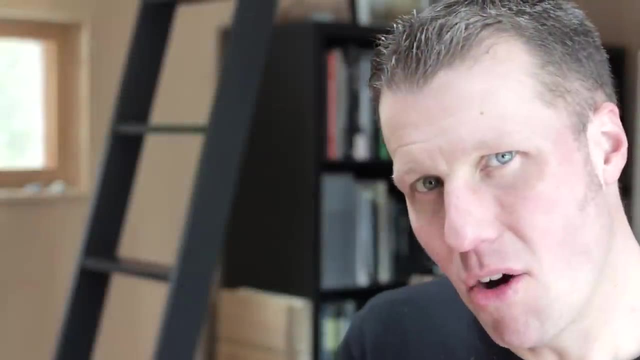 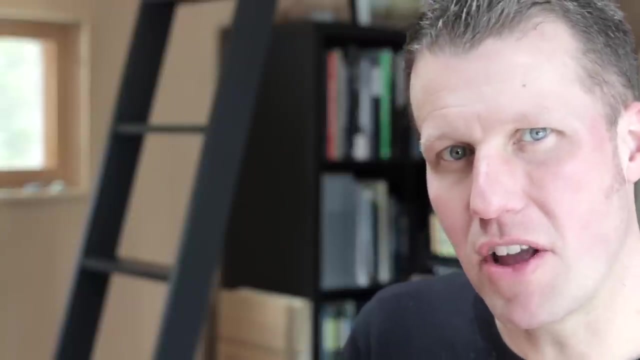 organization of the building to complement the site features too. I used the view to the cove, as well as the solar aspect, to select the most desirable site for the home. Now, often, competing site factors will force you to choose one site force as more dominant, For example the prevailing 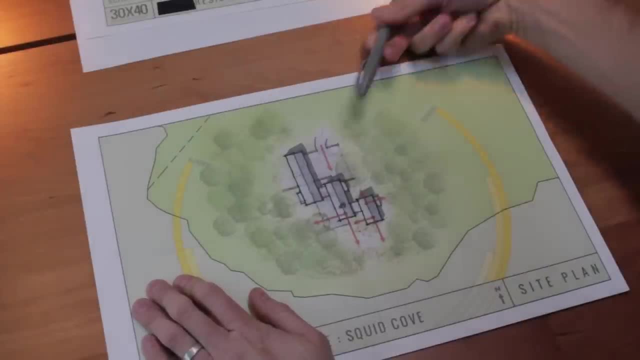 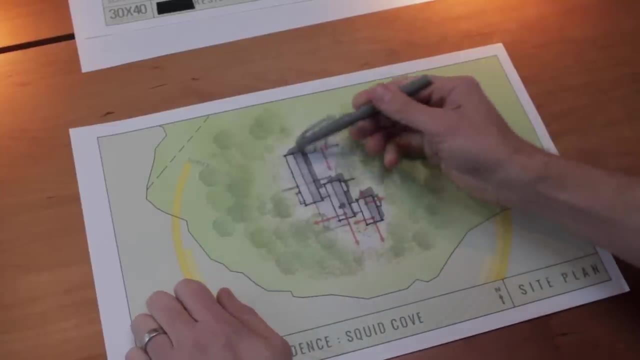 wind direction is in the direct competition with the idea that the wind direction is more dominant. If we were to position a taller mass to the northwest to act as a natural windscreen, it would impact our afternoon sun and prevent an arrival sequence which presented the view. 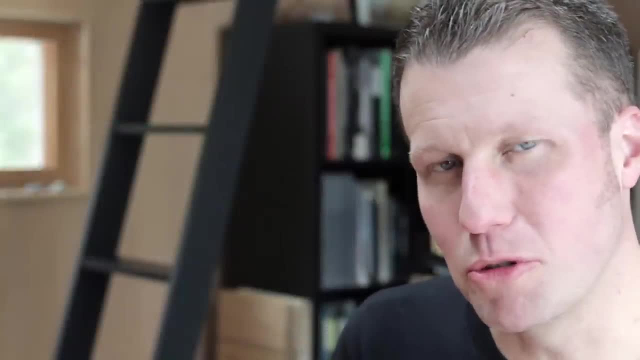 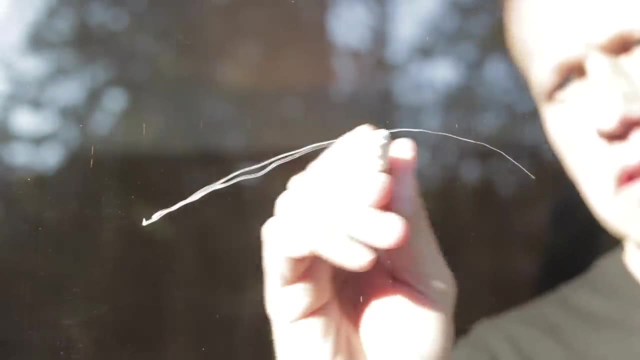 rather than the building. Not all problems will be solved by assuming a singular attitude toward the site. What was most important was the idea that the building, conformed to the topography Unfolding along the hillside, allowed the building to create a series of terraced plains. 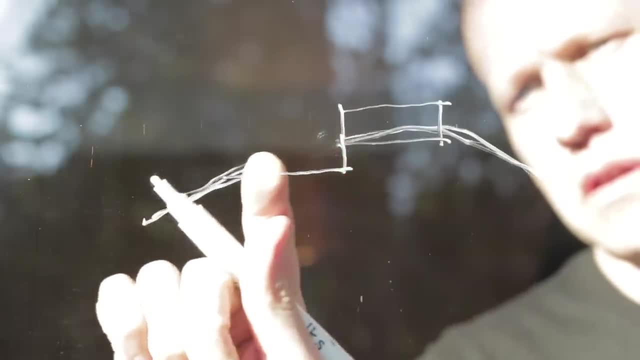 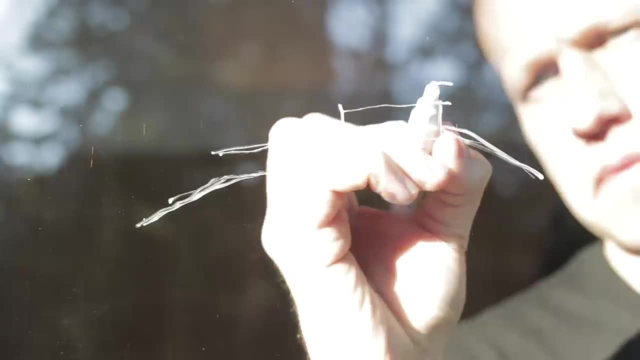 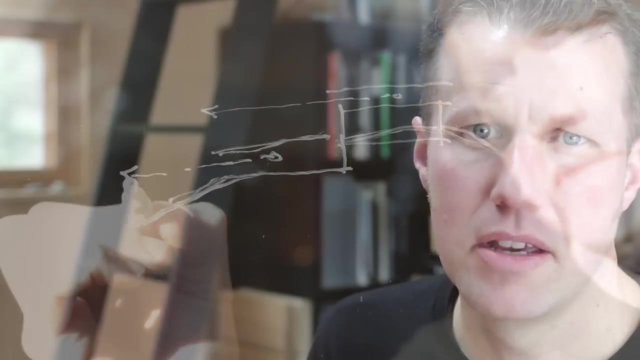 and transition spaces mediating inside and out. We could then use these to establish intermediate zones between architecture and nature. Using the hard edge- site retaining walls and decks- would give us the chance to highlight and contrast the soft edges of the site. Equally, I could have positioned the home at the top of the site and used it as a light. 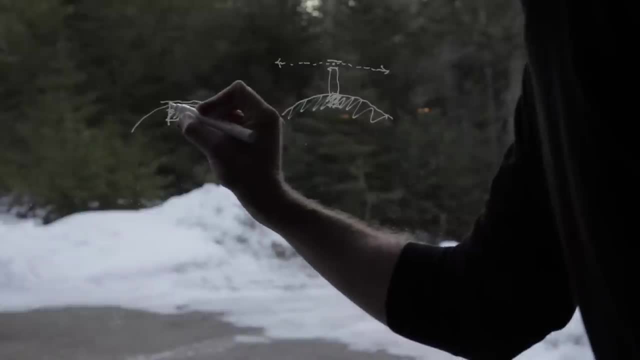 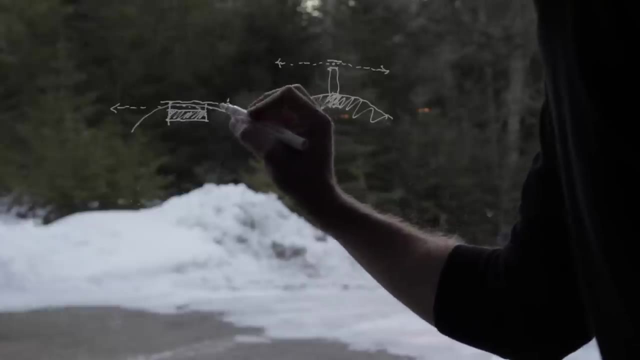 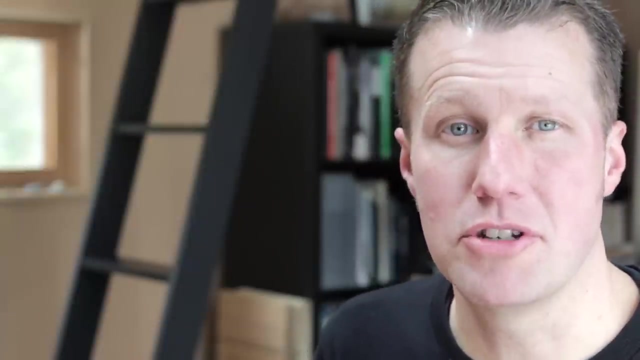 monitor or a viewing tower, or I could have completely excavated the terraces, placed a green roof on top and concealed the home. Although these were ideas I explored along the way, they were abandoned. as my client helped shape the decision making, The site helps to shape other dimensions of our concept too. 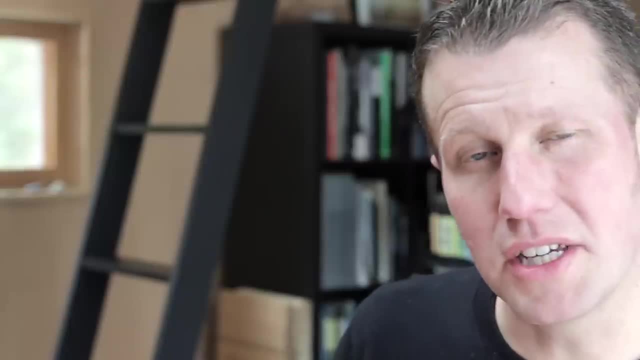 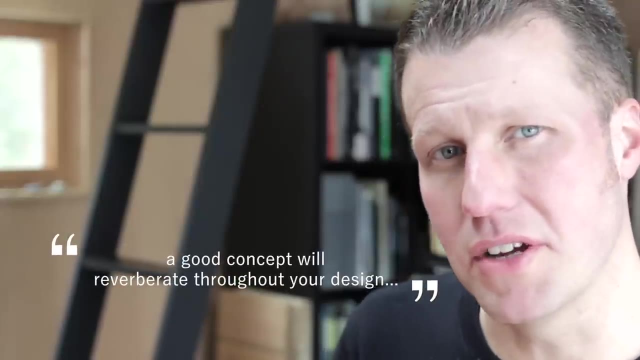 things like the material and structural concept and we'll get into those in future videos. But you'll begin to see- and it's worth noting- how the concept reverberates throughout the design. You'll always be referring back to it as you iterate and look to it when you're stuck on a 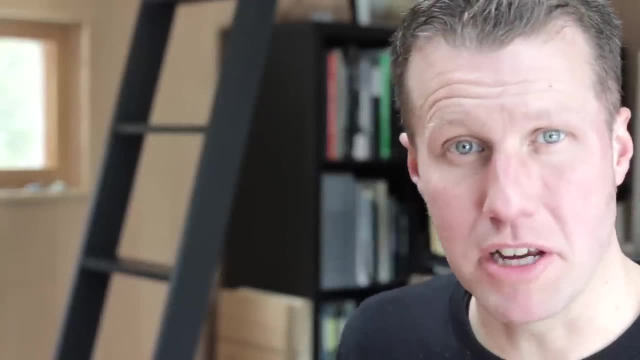 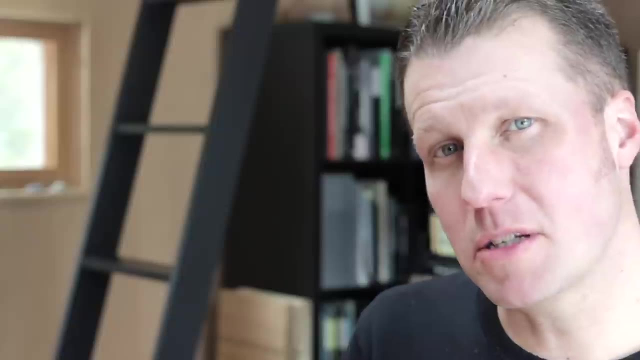 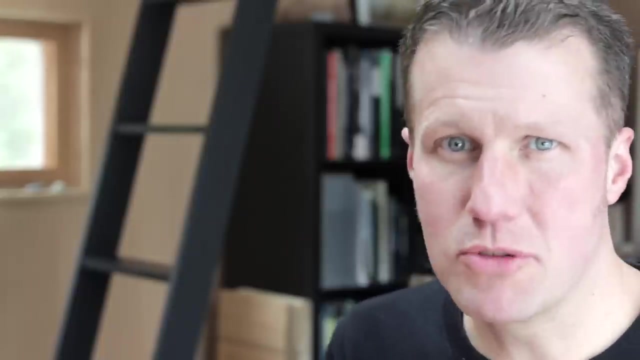 design problem. The site will obviously inform the organization of public and private spaces too, How one arrives and moves from the public gathering spaces to the more private sleeping spaces. It shapes where we locate windows, which would be to the views and to capture the sun. and the site informs the formal concepts too. 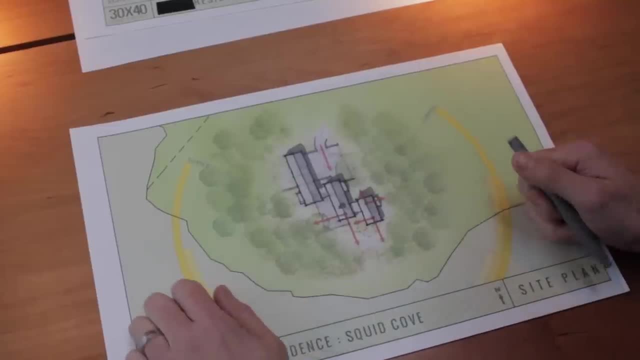 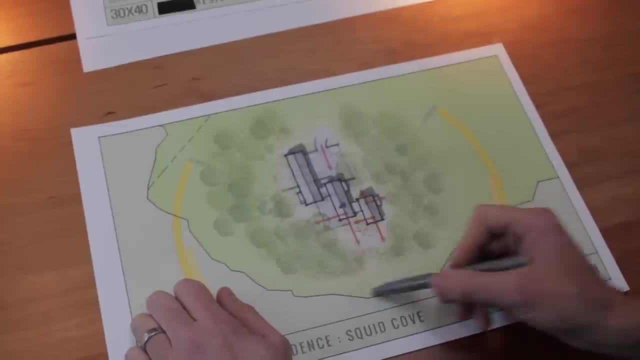 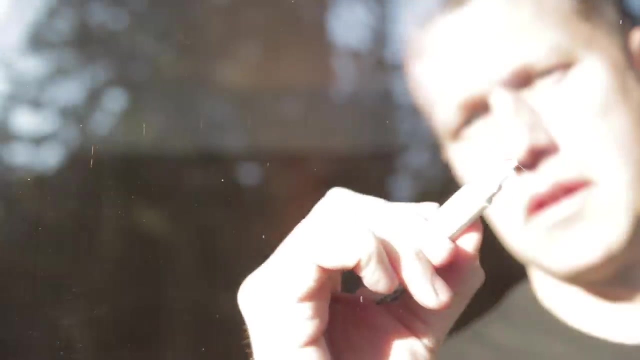 to position a taller mass to the northwest to act as a natural windscreen. it would impact our afternoon sun and prevent an arrival sequence which presented the view rather than the building. Not all problems will be solved by assuming a singular attitude toward the site. 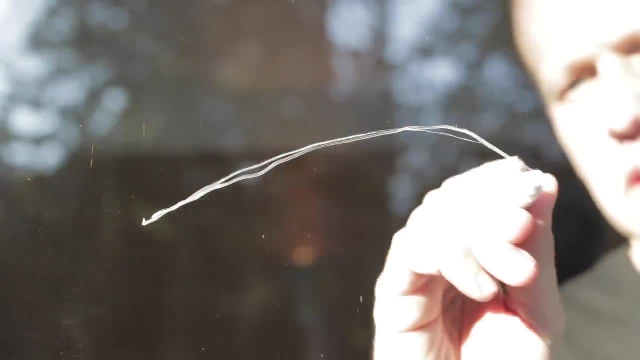 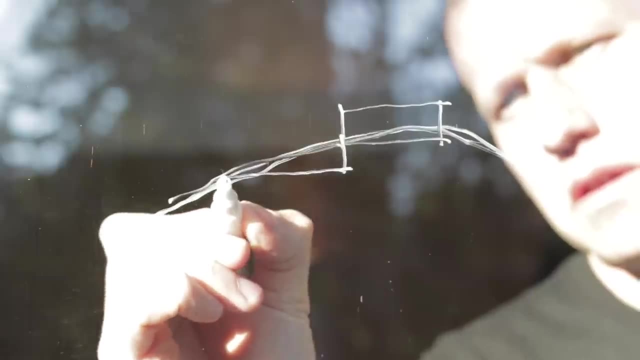 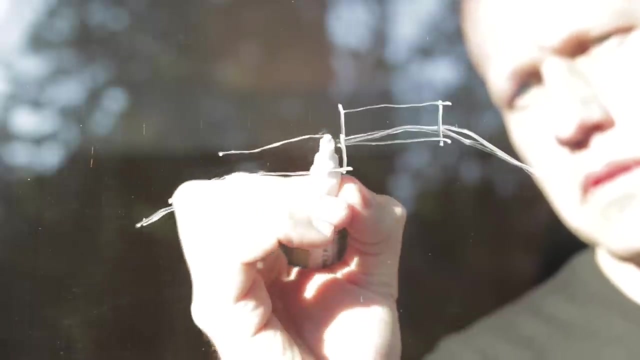 What was most important was the idea that the building, conformed to the topography Unfolding along the hillside, allowed the building to create a series of terraced plains and transition spaces mediating inside and out. We could then use these to establish intermediate zones between architecture and nature. 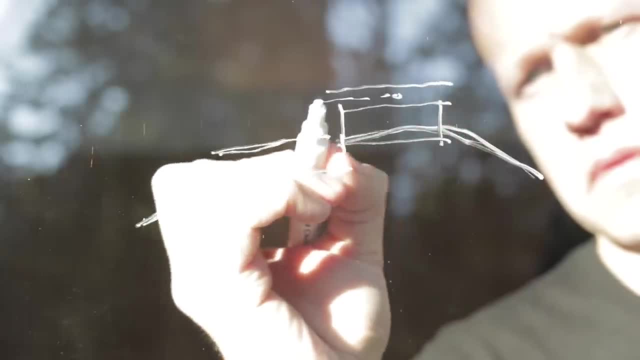 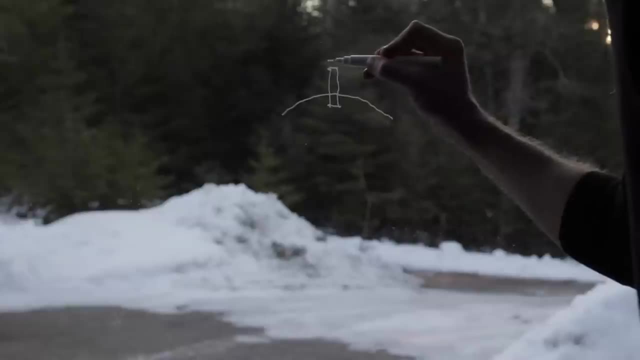 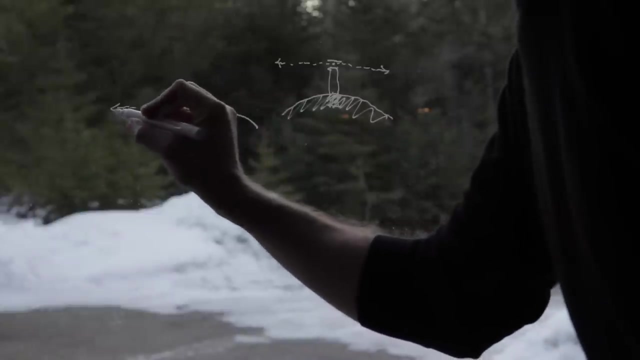 Using the hard-edged site retaining walls and decks would give us the chance to highlight and contrast the soft edges of the site. Equally, I could have positioned the home at the top of the site and used it as a light monitor or a viewing tower, or I could have completely excavated the terraces placed. 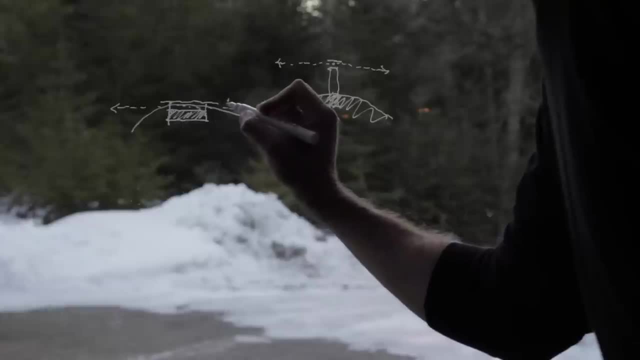 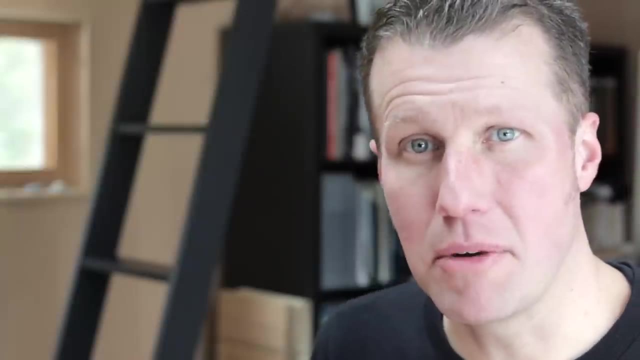 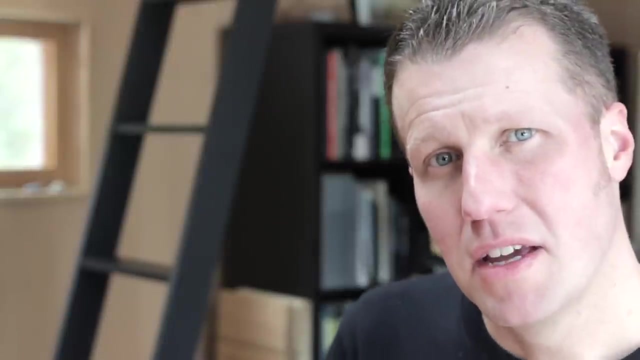 a green roof on top and concealed the home, And Although these were ideas I explored along the way, they were abandoned, as my client helped shape the decision making. The site helps to shape other dimensions of our concept too, things like the material and structural concept, and we'll get into those in future videos. 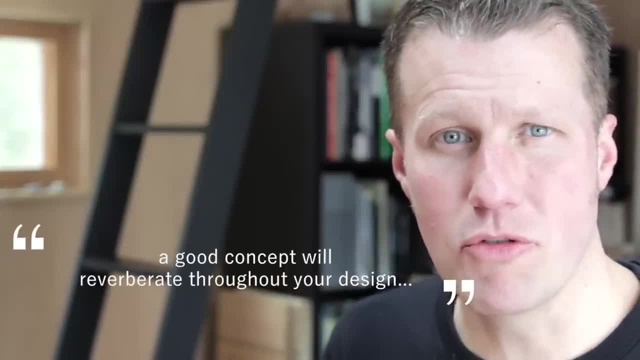 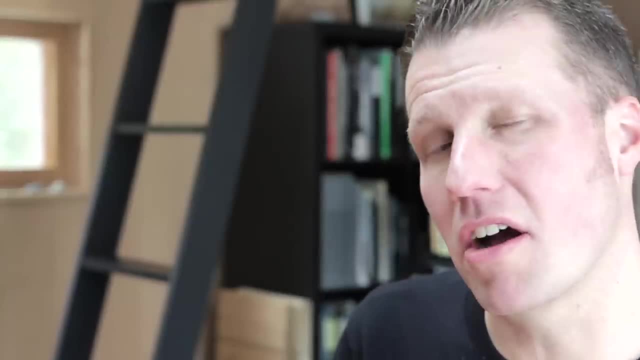 But you'll begin to see- and it's worth noting- how the concept reverberates throughout the design. You'll always be referring back to it as you iterate and look to it when you're stuck on a design problem. The site will obviously inform the organization of public. 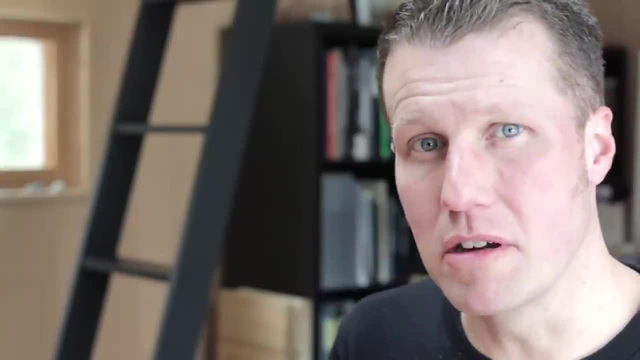 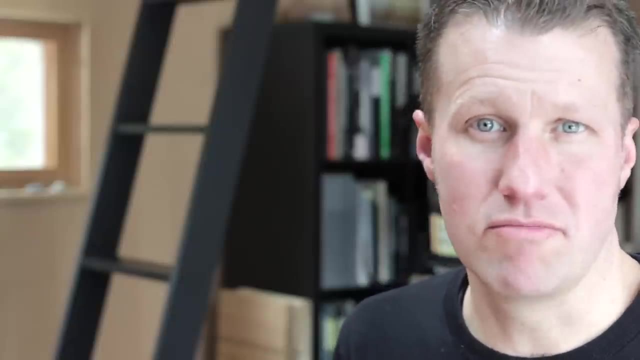 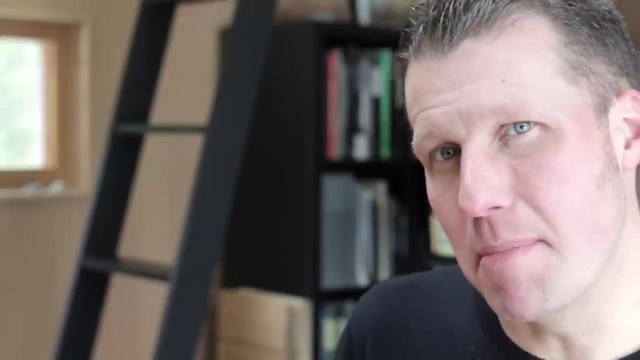 and private spaces too, How one arrives and moves from the public gathering spaces to the more private sleeping spaces. It shapes where we locate windows, which would be to the views and to capture the sun, And the site informs the formal concepts too. This site concept is like a marriage. 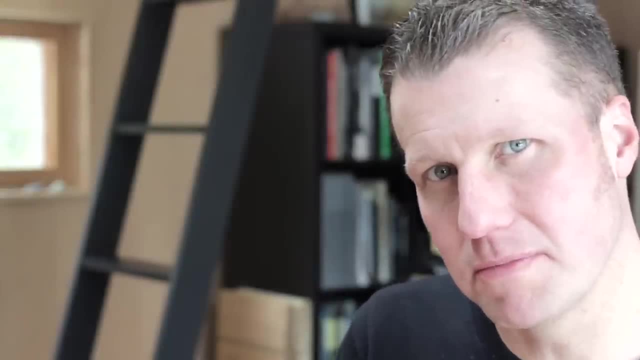 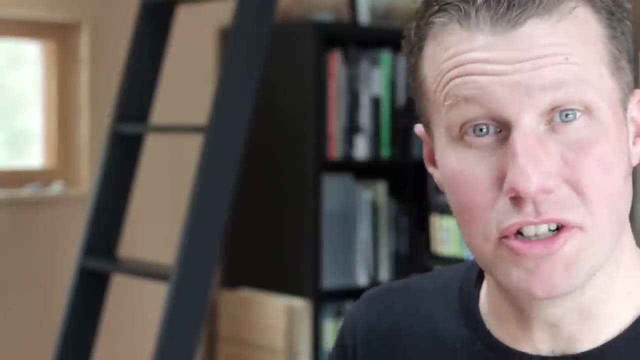 The architecture shapes the site and the site shapes our architecture. So this is not enough, you say. Well, I agree, There's more meaning to extract and more layers to the concept we should explore. So inspiration number two: the client concept. Every work of architecture requires a. 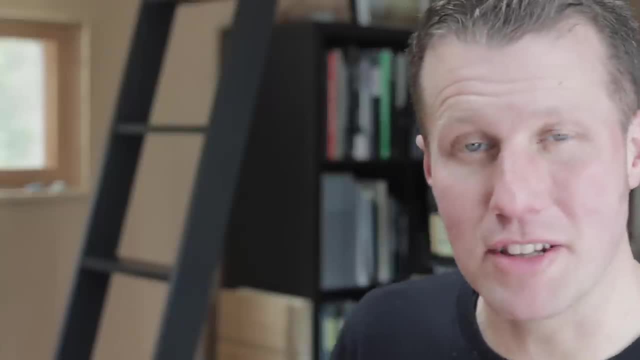 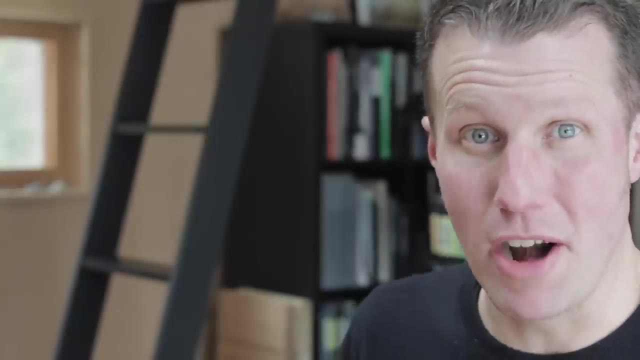 client For residential architecture. the client is a major force driving the design concept, not only from an aesthetic point of view but also programmatically. The client determines the program and which spaces are most important in that program, And they obviously provide the 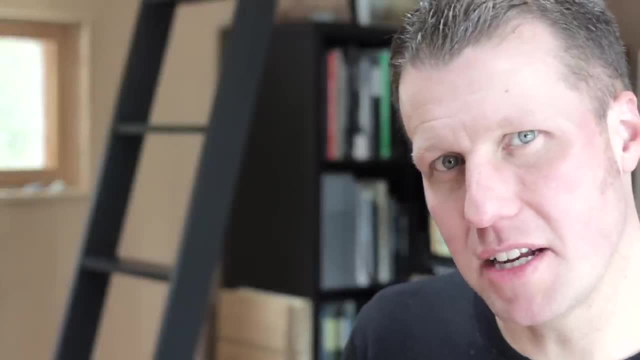 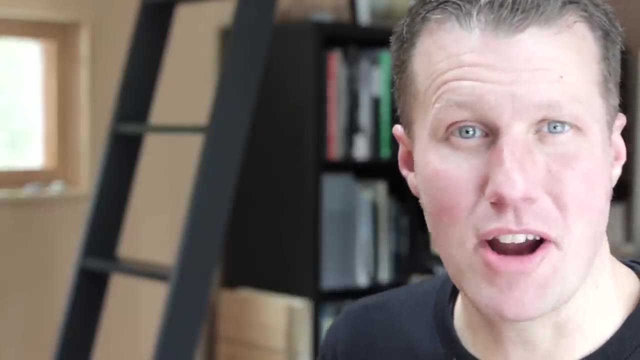 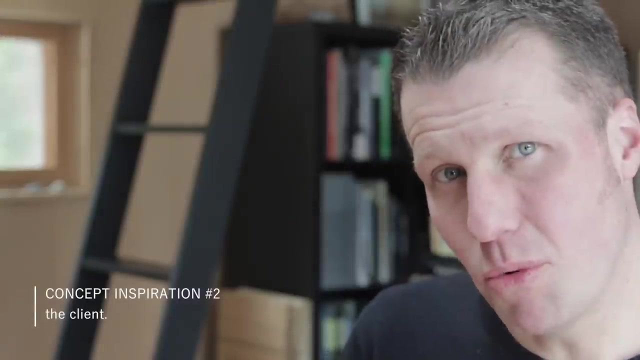 This site concept is like a marriage: the architecture shapes the site and the site shapes our architecture. So this is not enough, you say. Well, I agree, there's more meaning to extract and more layers to the concept we should explore. So, inspiration number two, the client concept. 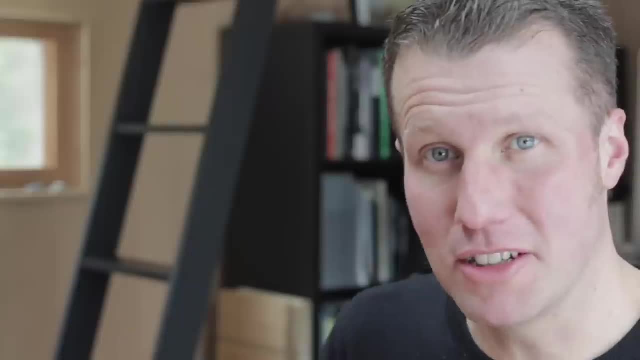 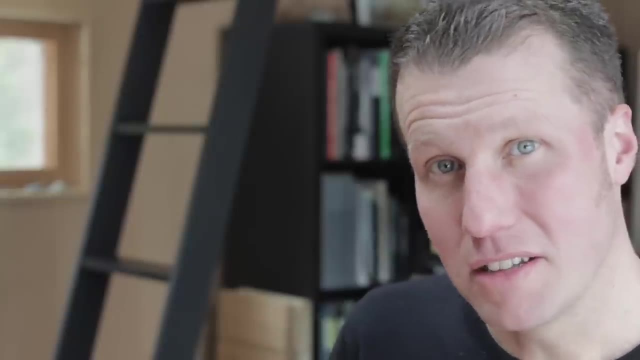 Every work of architecture requires a client. For residential architecture, the client is a major force driving the design concept, not only from an aesthetic point of view, but also programmatically. The client determines the program and which spaces are most important in that program. 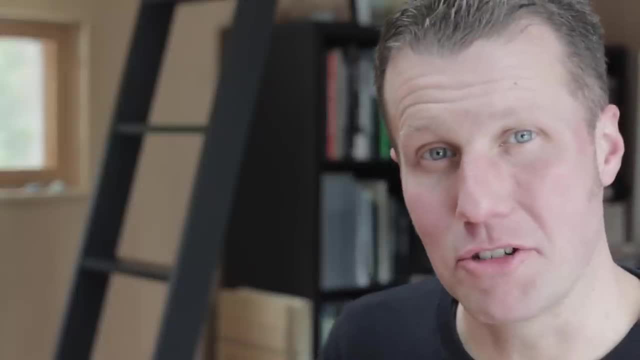 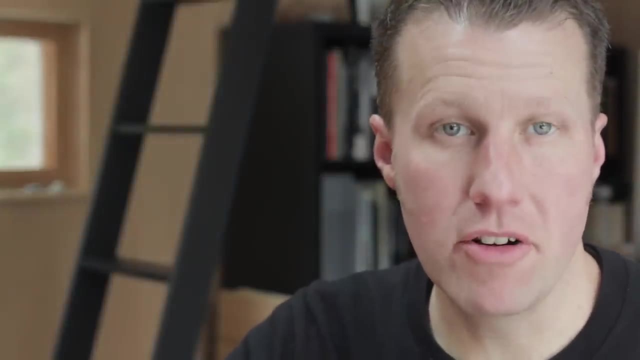 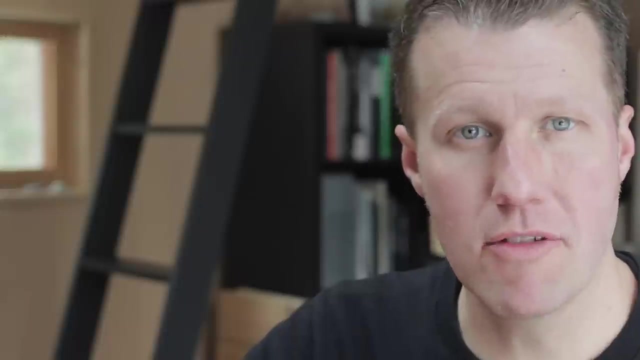 And they obviously provide the financial framework for realizing the architecture. Successful architecture artfully addresses a client's needs. Now, client-driven concepts can take the form of narratives or lifestyle peculiarities, or they can be purely functional, For example, a request for all living to be on one level or an open plan. 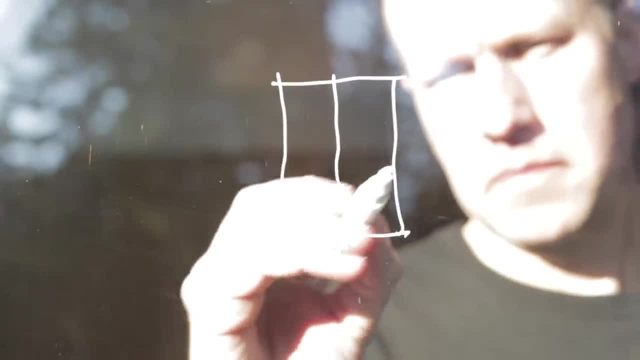 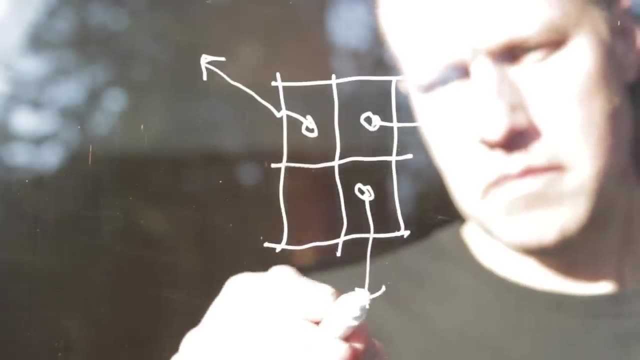 For this project. our client expressed a desire for the house to act as a gathering place for friends and family, but also that it accommodates seclusion and the need for retreat from others. Because we live in a seasonal community, the summer here often sees a massive influx of guests and visitors. So those who live here are likely to have a lot of fun and they're likely to have a lot of fun. So those who live here are likely to have a lot of fun and they're likely to have a lot of fun, and they're likely to have a lot of fun and they're likely to have a lot of fun. 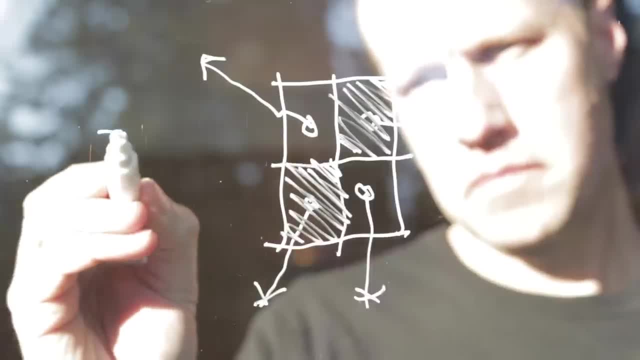 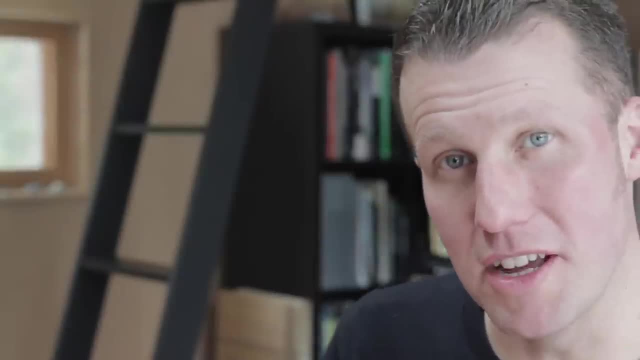 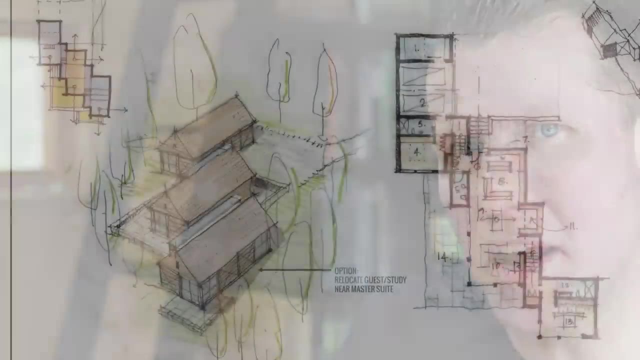 And, because we live here year round, are accustomed to welcoming house guests in the summer months. this inspired the division of spaces into separate living and sleeping pods, Each afforded a unique aspect or view to the site. As we begin to organize the spaces of the client-driven program, a simple way to develop. 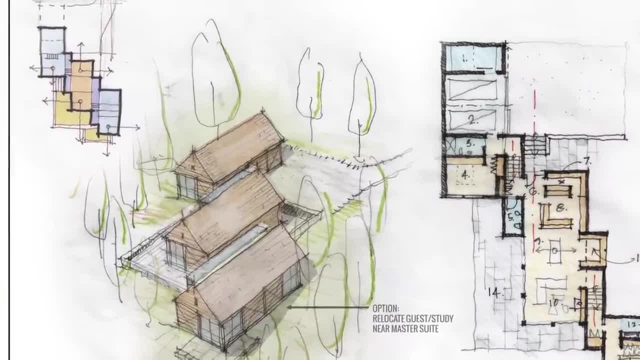 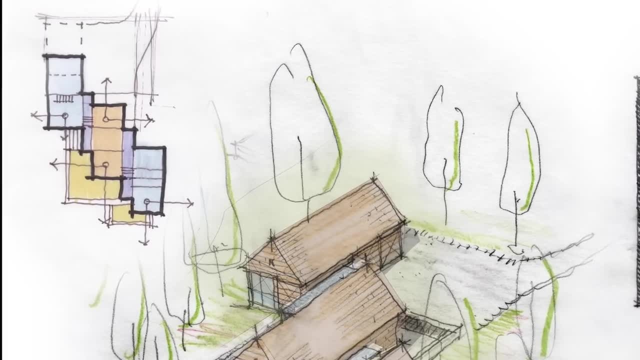 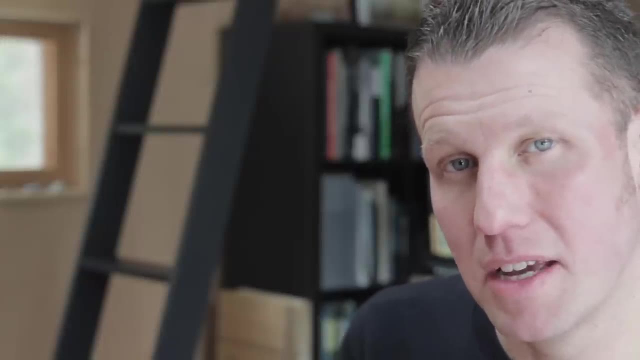 a concept is to divide public and private spaces and then take a position on their relationship. Perhaps you overlap them, perhaps they're in separate pods or nested, Perhaps their relationship is inverted. From here, begin to diagram your concept and iterate For our project. we continued on by layering our client's interest in the outdoors and 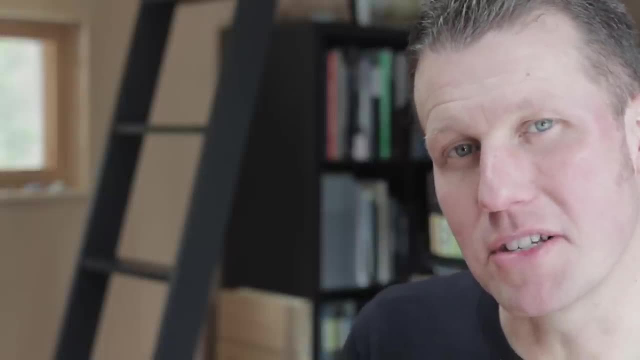 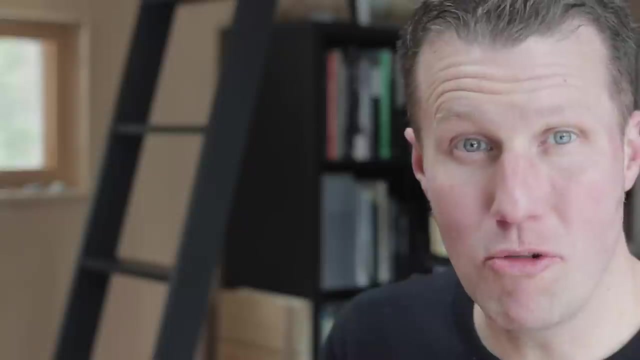 a near constant schedule of expeditions to faraway places. This lifestyle helped fuel a story about what the house could be, how it might function and when they were home and when they were traveling, and where we might position the spaces in relation to each other. 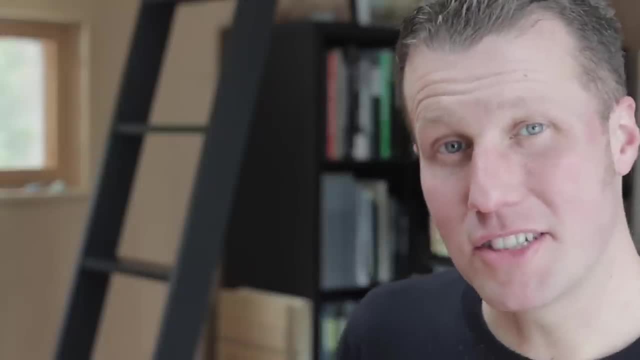 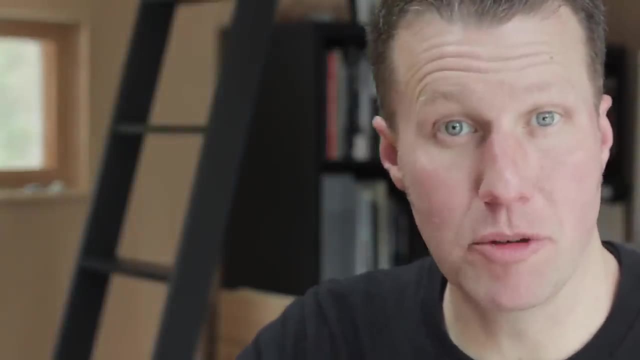 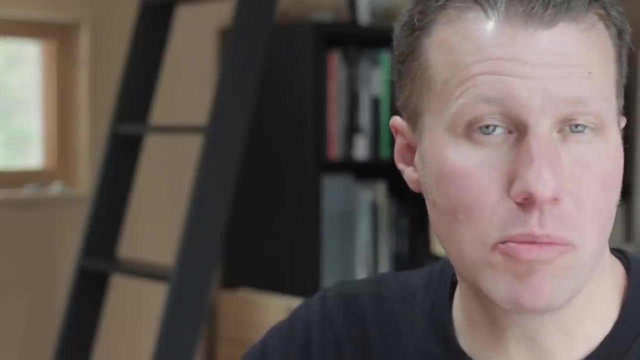 financial framework for realizing the architecture. Successful architecture artfully addresses a client's needs. Now, client-driven concepts can take the form of narratives or lifestyle peculiarities, or they can be purely functional, For example, a request for all living to be on one level or an open plan For this. 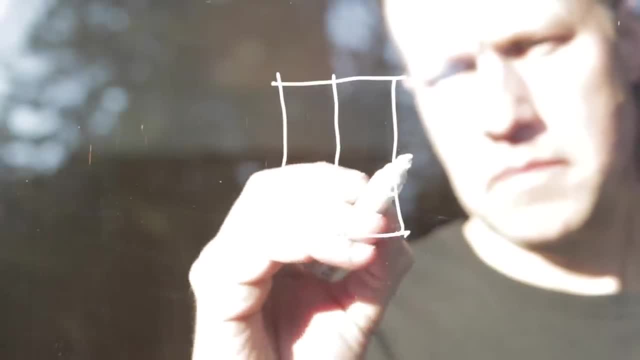 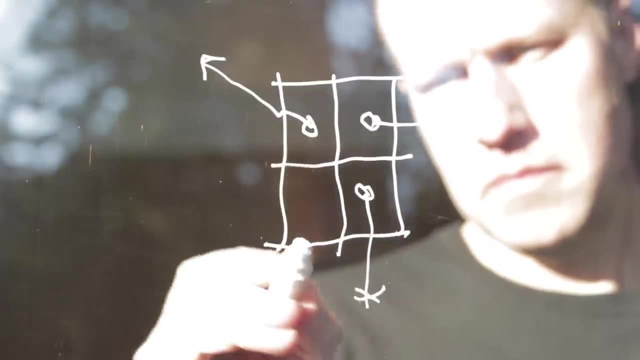 project. our client expressed a desire for the house to act as a gathering place for friends and family, but also that it accommodates seclusion and the need for retreat from others. Because we live in a seasonal community, the summer here often sees a massive influx of guests and visitors. 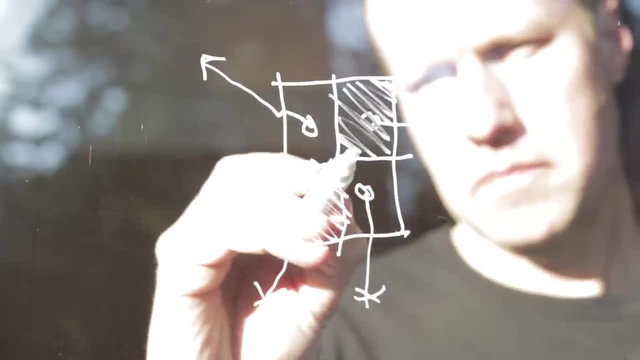 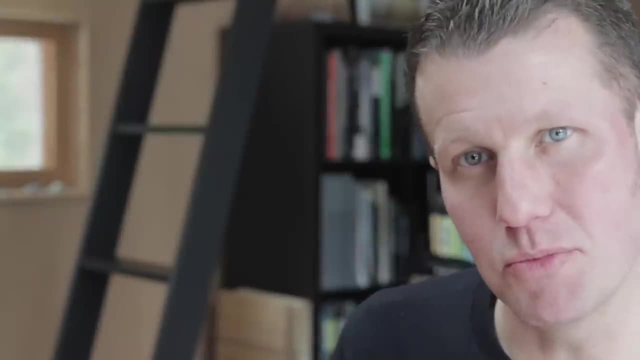 So those who live here around are accustomed to welcoming house guests in the summer months. This inspired the division of spaces into separate living and sleeping pods, Each afforded a unique aspect or view to the site. As we begin to organize the spaces of the client-driven program, 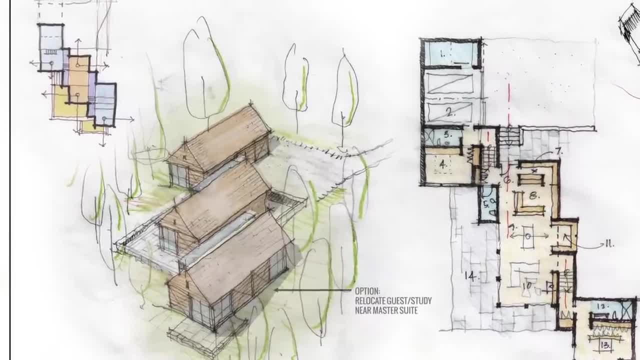 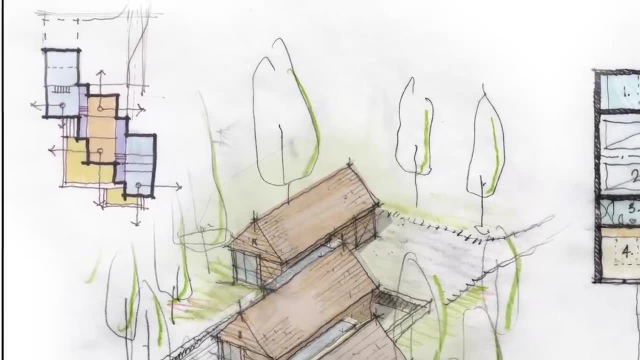 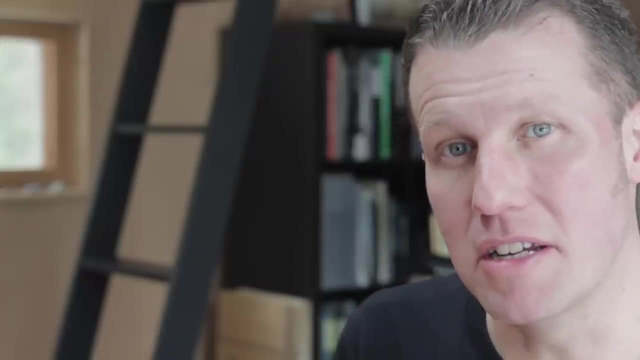 a simple way to develop a concept is to divide public and private spaces and then take a position on their relationship. Now, perhaps you overlap them, perhaps they're in separate pods or nested, perhaps their relationship is inverted. From here, begin to diagram your concept and iterate For our project. we continued on by 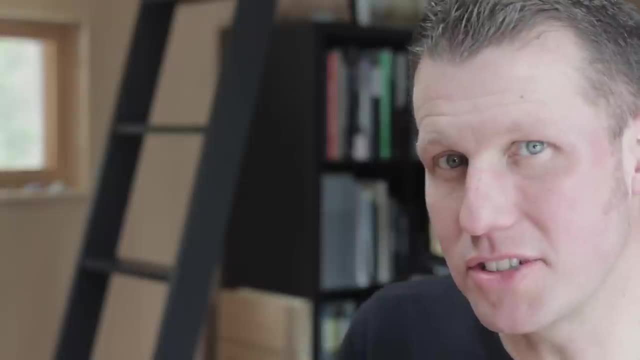 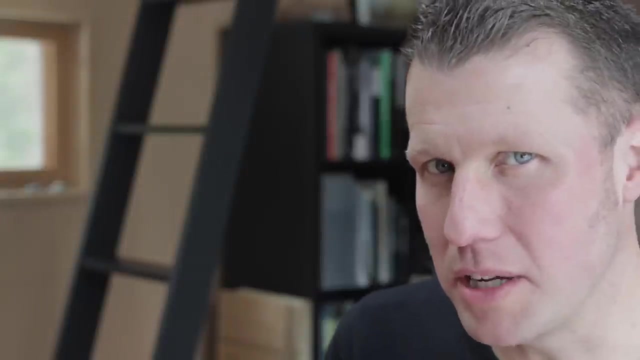 layering our client's interest in the outdoors and a near constant schedule of expeditions to faraway places. This lifestyle helped fuel a story about what the house could be, how it might function and when they were home and when they were traveling, and where we might position the. 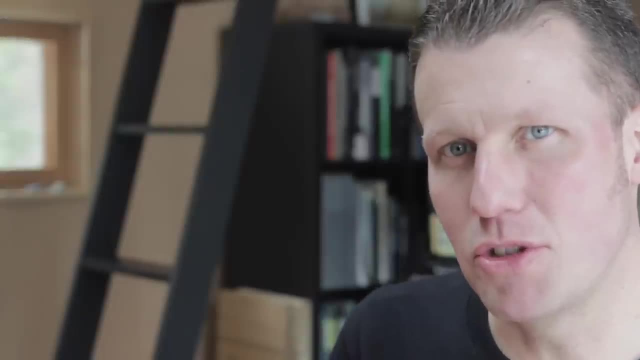 spaces in relation to each other, And this brings us to inspiration number three, the narrative concept, Inspired by an attitude about how our client might live in the home and welcome guests, and how they plan to move in and out of the spaces and mobilize gear. this all suggested to me the 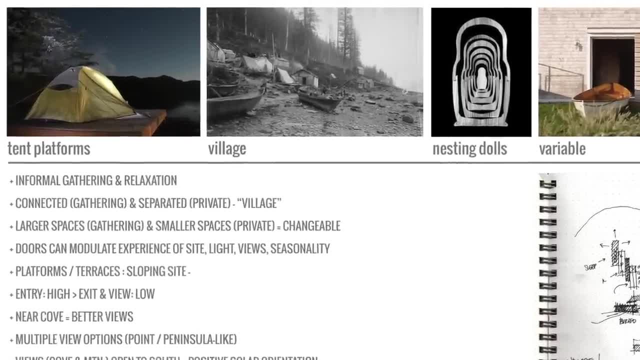 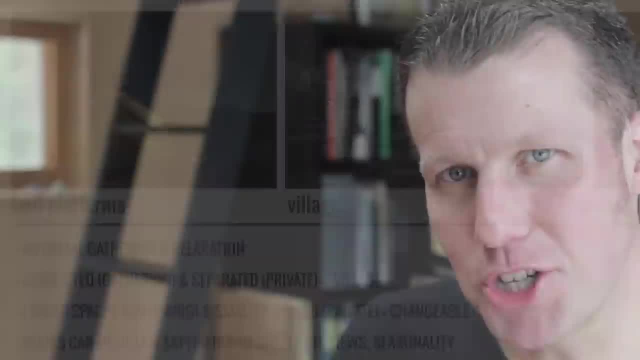 imagery of an encampment by the sea. I envisaged the home as a place for family and friends to gather, and sort of camp, together Uniting in the evenings around the campfire to share a meal, but retreating to private comfort. 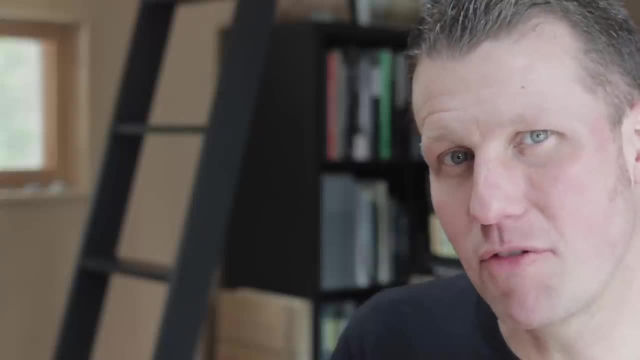 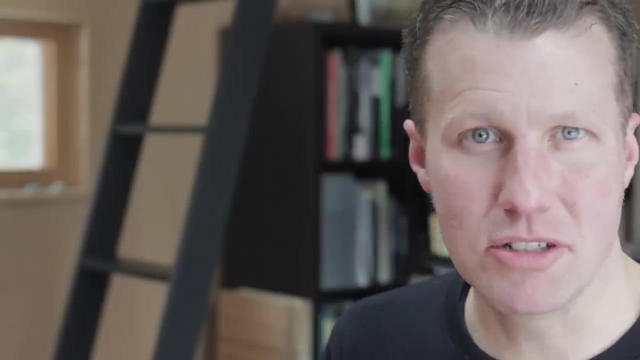 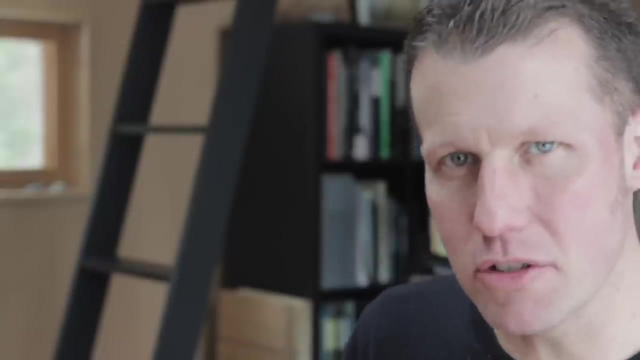 for sleeping. The village concept provided for both social gathering and private reflection as needed. Expedition travel allowed the house to expand and contract with the seasons and with ebbs and flows of visitors. And this story, as we'll see, begins to inform layers of meaning. 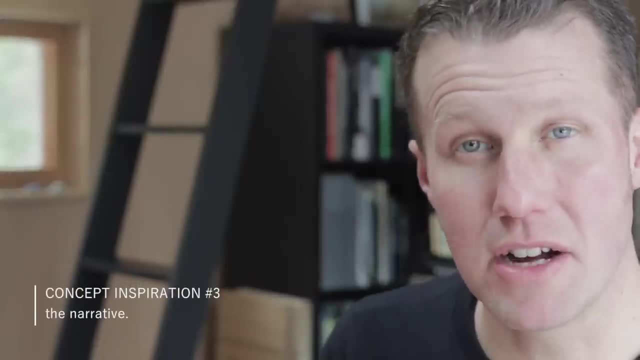 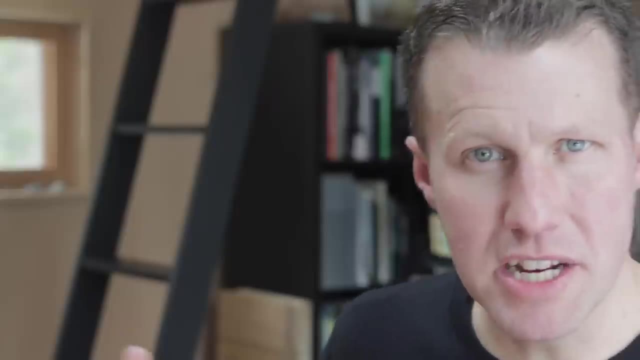 And this brings us to inspiration number three, the narrative concept Inspired by an attitude about how our client might live in the home and welcome guests, and how they plan to move in and out of the spaces and mobilize gear. this all suggested to me the imagery of an encampment by the sea. 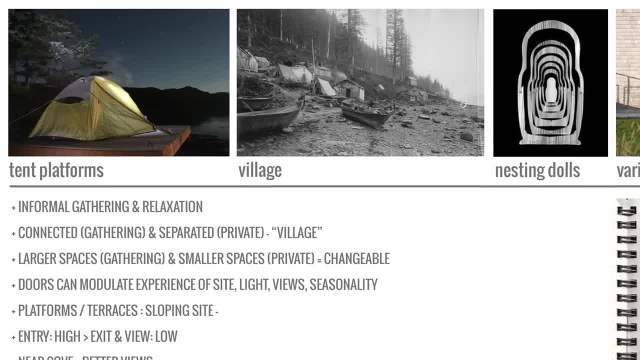 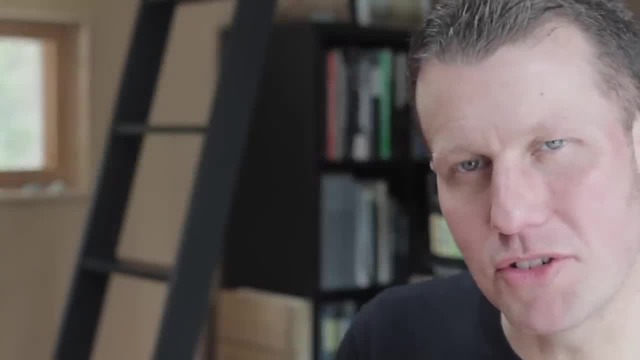 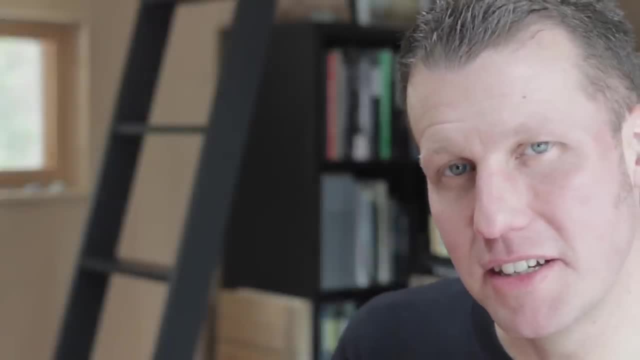 I envisaged the home as a place for family and friends to gather and sort of camp together Uniting in the evenings around the campfire to share a meal but retreating to private quarters for sleeping. The village concept provided for both social gathering and private reflection as needed. 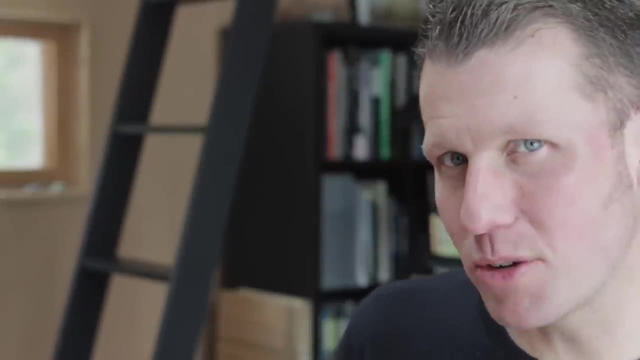 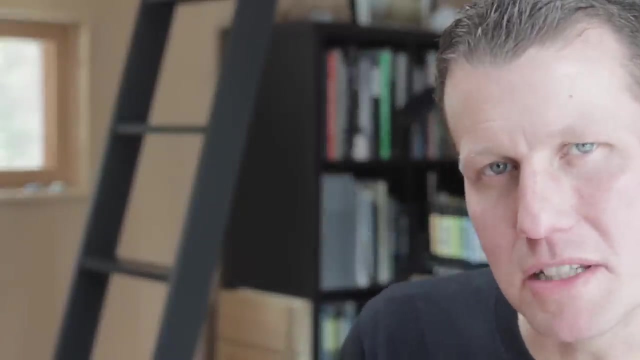 Expedition travel allowed the house to expand and contract with the seasons and with ebbs and flows of visitors, And this story, as we'll see, begins to inform layers of meaning as we develop the floor plans and exterior elevations. later, Nested pods provided for escape within the larger space of the home and a variety of 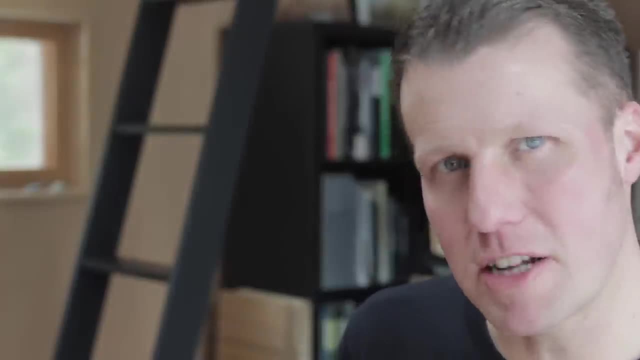 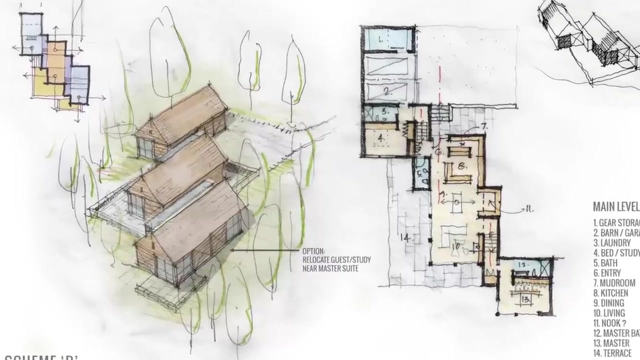 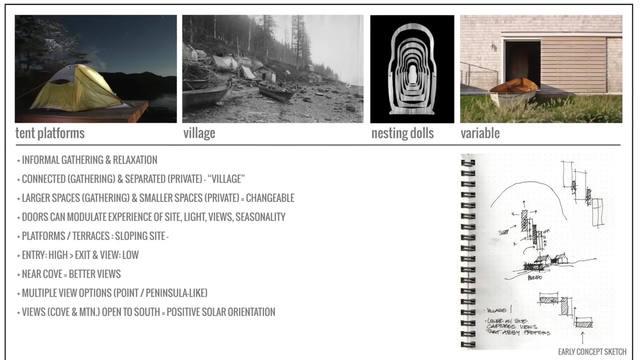 scales, mimicked the site beyond and my client's need for respite and seclusion. And this is where we begin. Each one of these ideas exists in various forms in the early design concepts presented Now. I created this cover sheet to describe the thinking behind the plans, but it may 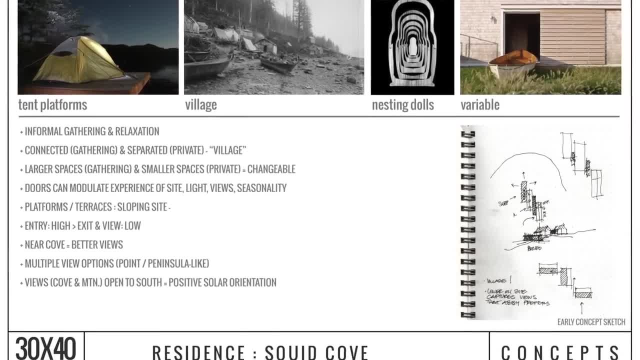 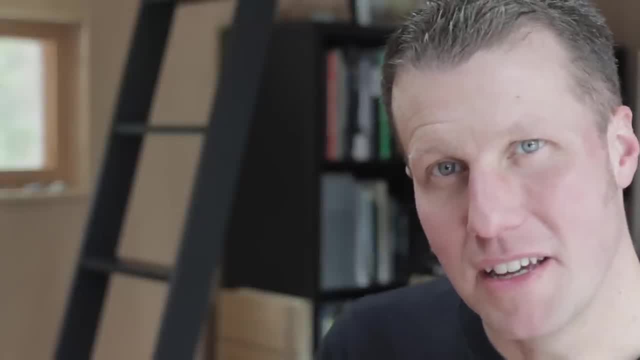 not be important for you to convey this to your client. It's sort of up to you. I think it adds a level of interest and a discussion point, but not every client will see the value. It's most important that it exists for you as you develop the design. 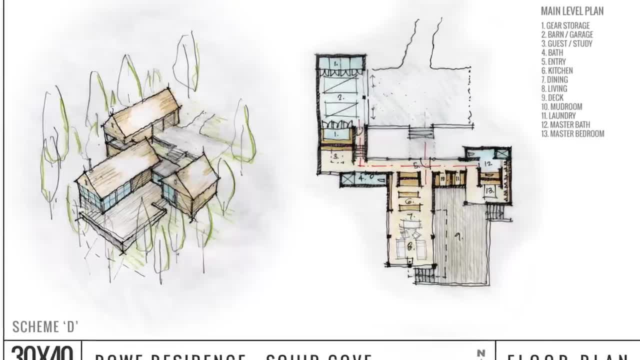 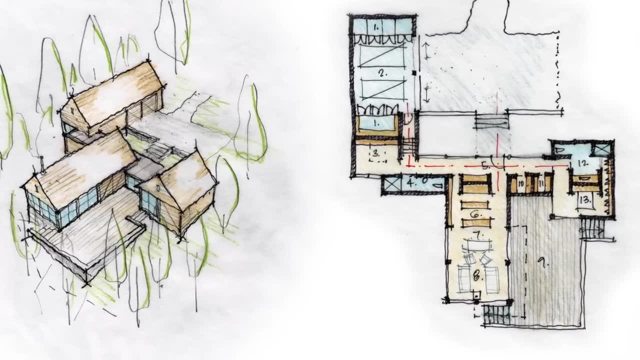 They will, of course, care most about the design. They will, of course, care most about what the design looks and feels like, And so, at this stage, I present very loose sketched plans to give an idea of how each concept deploys the program on the site and within the home. 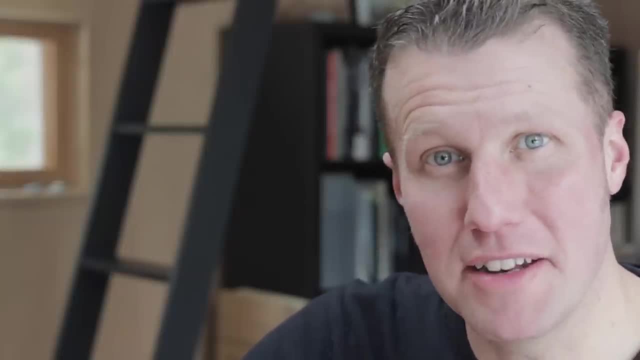 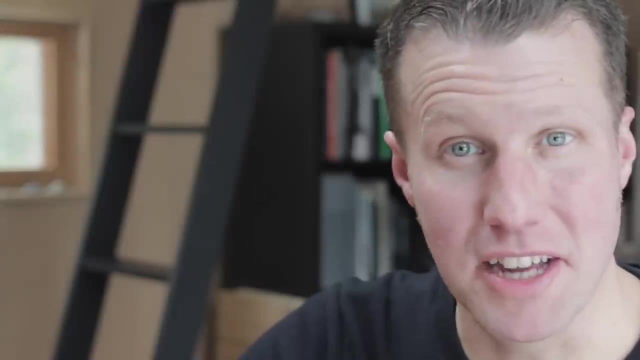 This process usually incites reactions, both positive and negative, and you'll use it to pivot moving forward. So, as you can see, it's not a singular concept. There's a narrative that ties it together and suggests a means for organizing the spaces. 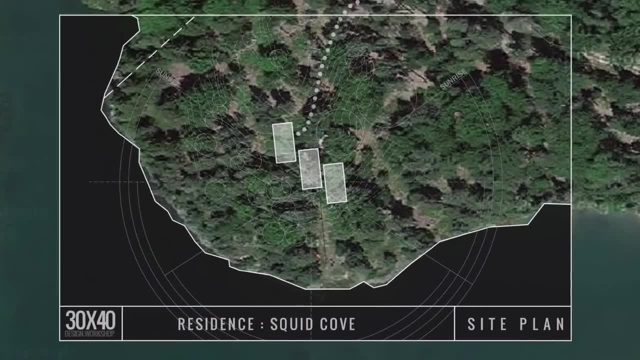 on the site. There's the site topography and natural features that suggest what's going on within the site. There's a narrative that ties it together and suggests a means for organizing the spaces on the site. There's the site topography and suggestions for organizing the spaces on the site. There's the site topography and suggestions for organizing the spaces on the site. There's the site topography and suggestions for organizing the spaces on the site, And so I talk a lot about where we want to locate the home, and there's our client's. 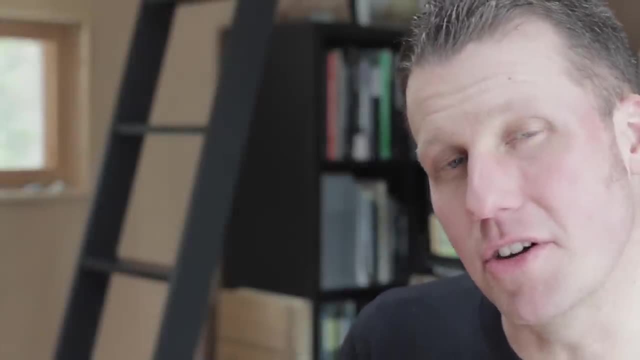 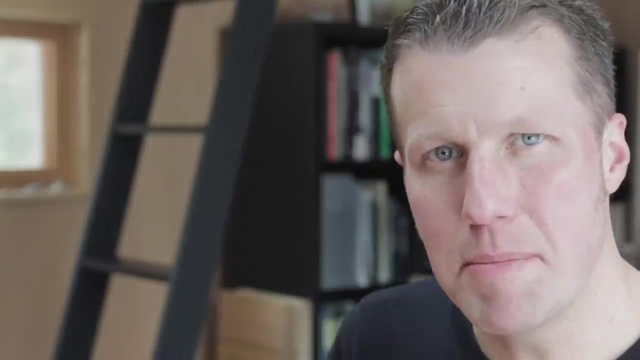 as we develop the floor plans and exterior elevations. later, Nested pods provided for escape within the larger space of the home and a variety of scales mimicked the site beyond. And this is where we see the client's need for respite and seclusion, even when surrounded by 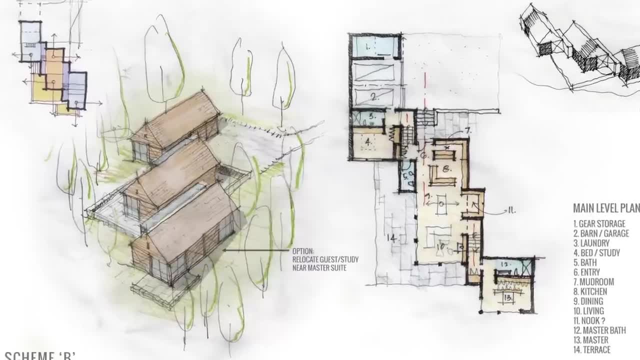 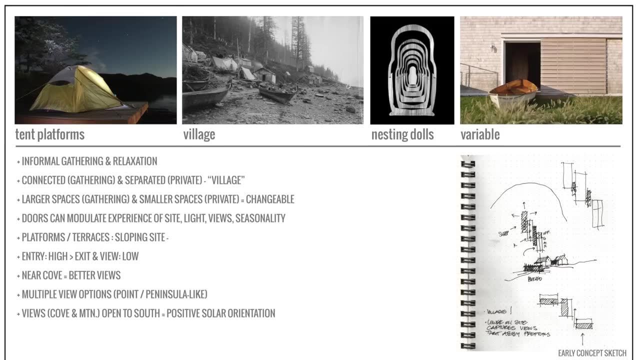 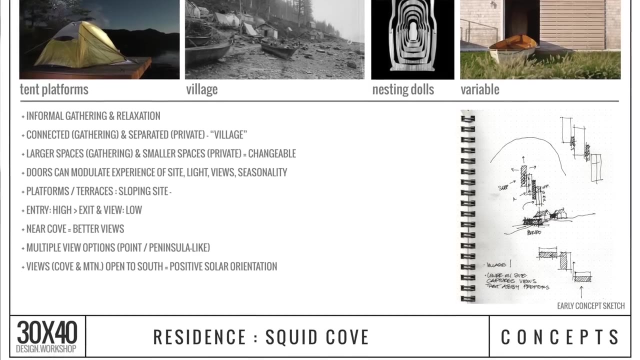 friends, Each one of these ideas exists in various forms in the earliest, early design concepts presented Now. I created this cover sheet to describe the thinking behind the plans, but it may not be important for you to convey this to your client. It's sort of up to you. I think it adds a 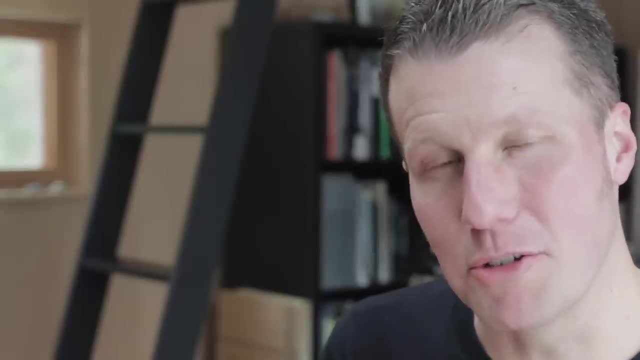 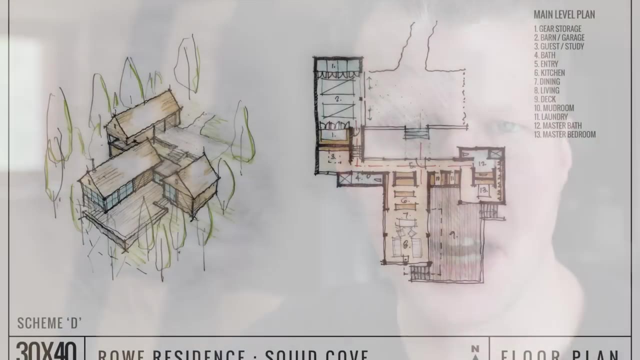 level of interest and a discussion point, but not every client will see the value. It's most important that it exists for you, The design. design is a very complex process. It requires a lot of time and effort to develop the design. They will, of course, care most about what the design looks and feels like, And so at this. 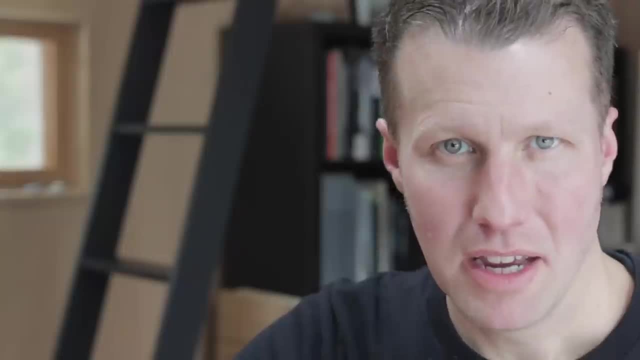 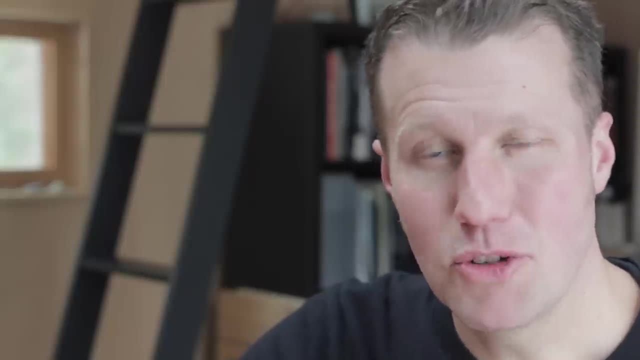 stage. I present very loose sketched plans to give an idea of how each concept deploys the program on the site and within the home. This process usually incites reactions, both positive and negative, and you'll use it to pivot moving forward. So, as you can see, it's not a singular concept. 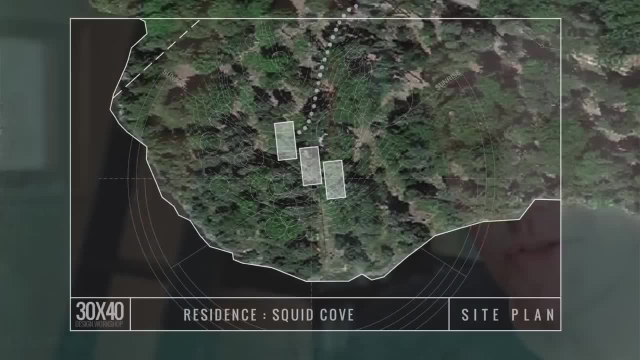 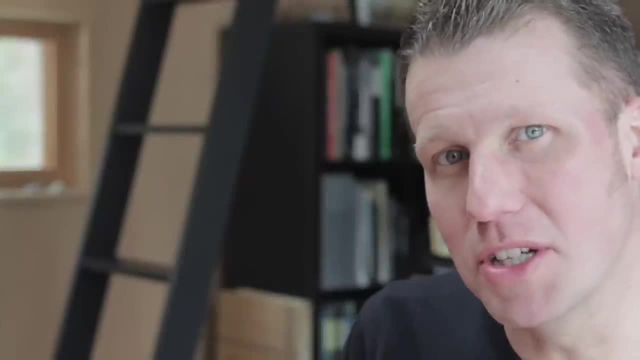 There's a narrative that ties it together and suggests a means for organizing the spaces on the site. There are natural features that suggest where we want to locate the home, And there's our client's life that tells us how the elements of their story can inform the architecture. 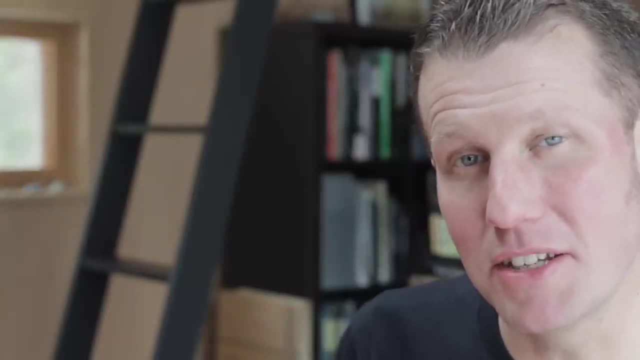 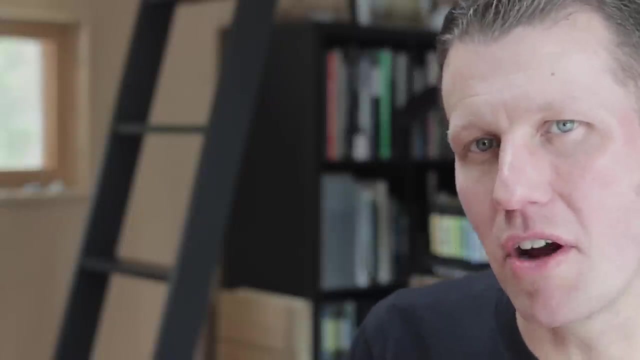 So I'd struggle to produce the diagram of this concept as gracefully as Maya Lin, but it's still a concept and it's informed every move I've made since. Sure, I revisited it and refined it, I've tweaked things based on client feedback and tastes, but it's still there and I continue to layer on. 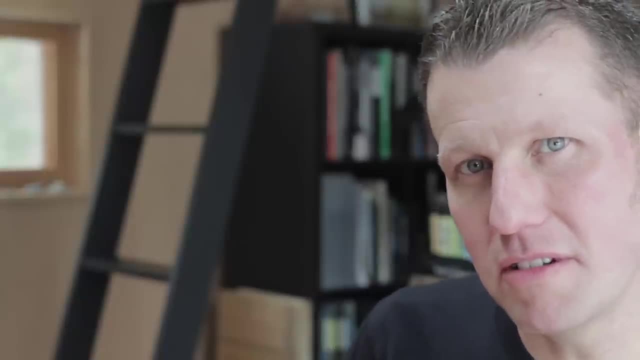 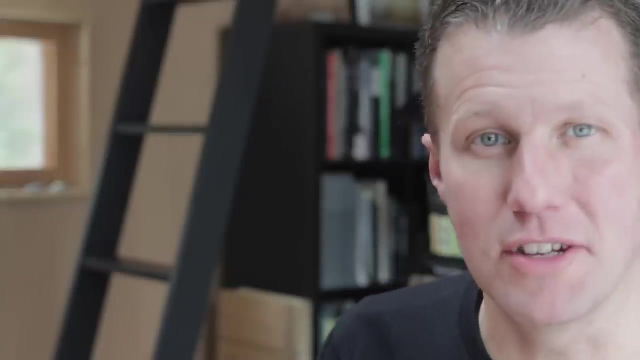 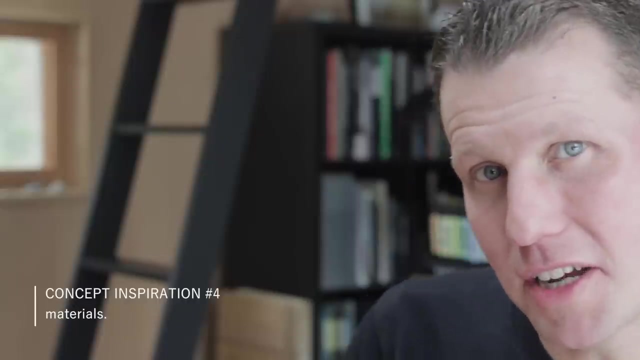 meaning as I develop the design. When there's a question, I know how to answer it because the conceptual framework is there to help. Now, there are, as I said, infinite other ways to develop concepts, So here's a few more if you're still stuck. Materials Architects like Peter Zumthor, Herzog & de Meurne and Peter 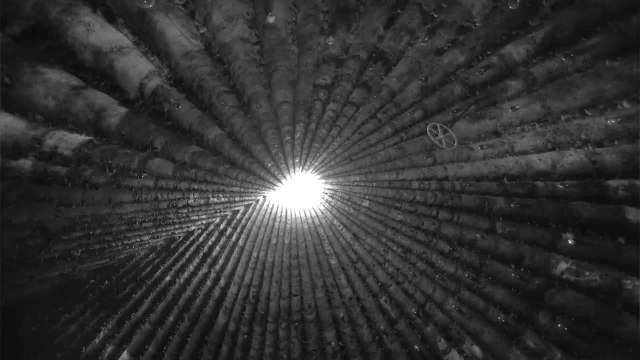 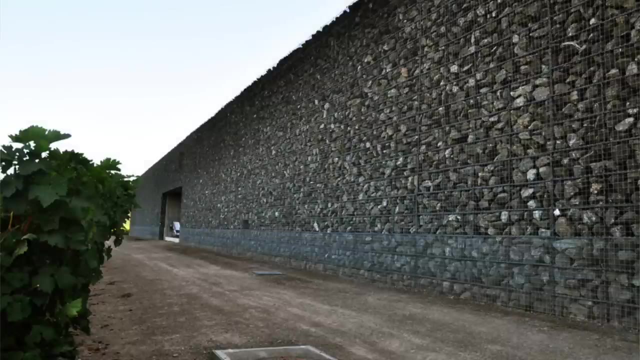 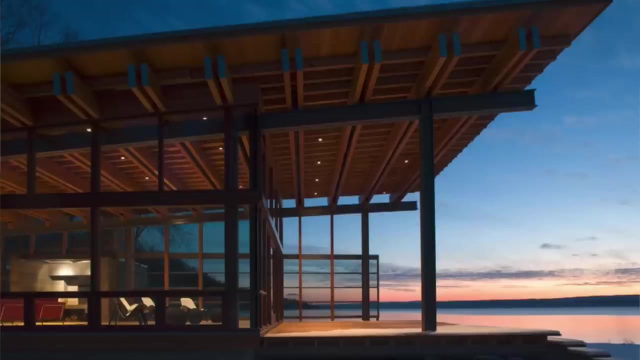 Bohlen often use the raw materials of building as the starting point for their work. Every line we trace on the page represents real physical materials coming together to make our architecture. Instead of rendering our work in pure white as we so often do, why not seek meaning from the materials we'll use to 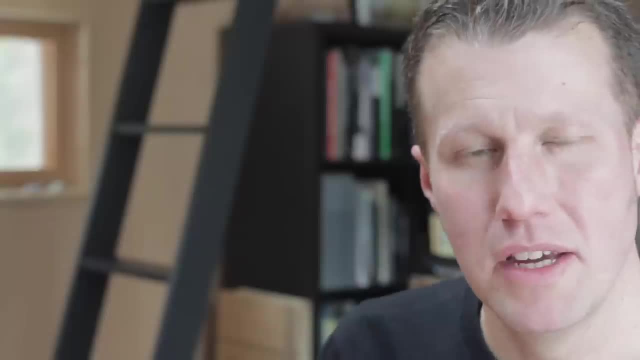 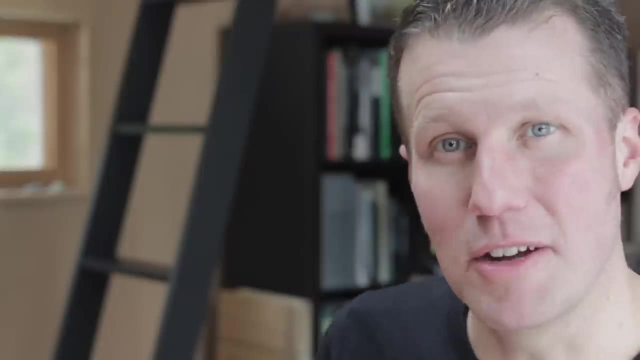 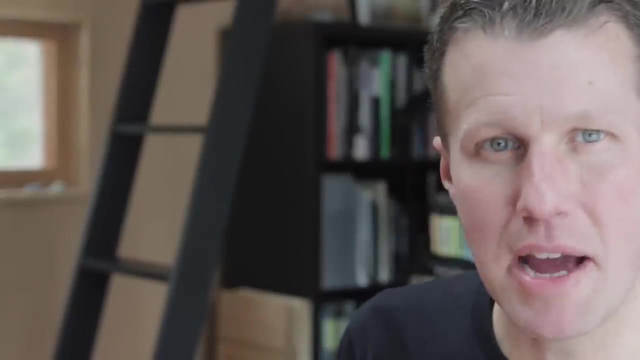 life that tells us how the elements of their story can inform the architecture. So I'd struggle to produce the diagram of this concept as gracefully as Maya Lin, but it's still a concept and it's informed. every move I've made since Sure, I revisited it and refined it. I've tweaked things based on client feedback and 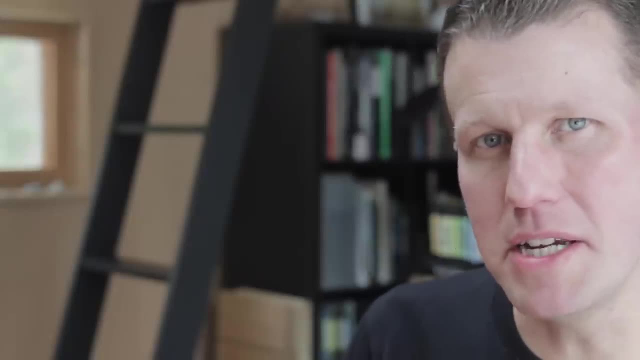 tastes, but it's still there and I continue to layer on meaning as I develop the design. When there's a question, I know how to answer it. I know how to answer it because the conceptual framework is there to help. Now there are, as I said, infinite other ways. 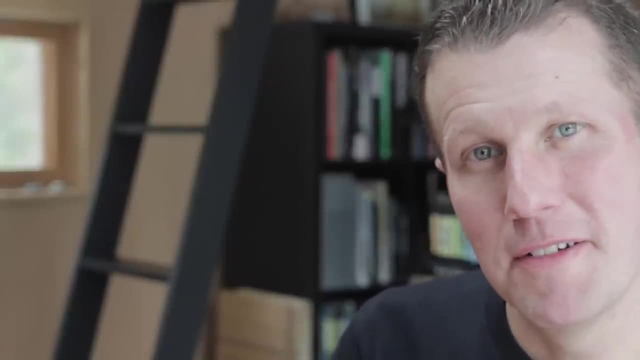 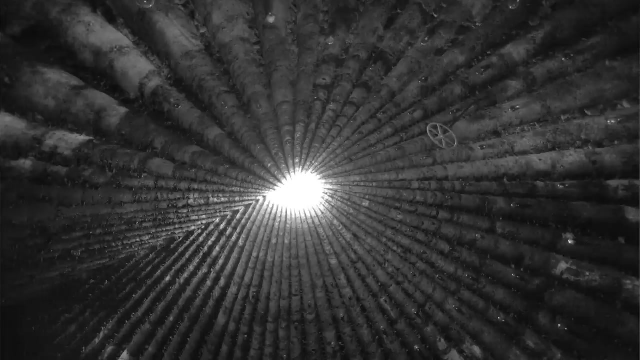 to develop concepts, So here's a few more if you're still stuck: Materials Architects like Peter Zumthor, Herzog and de Meurne and Peter Bohlen often use the raw materials of building as the starting point for their work. 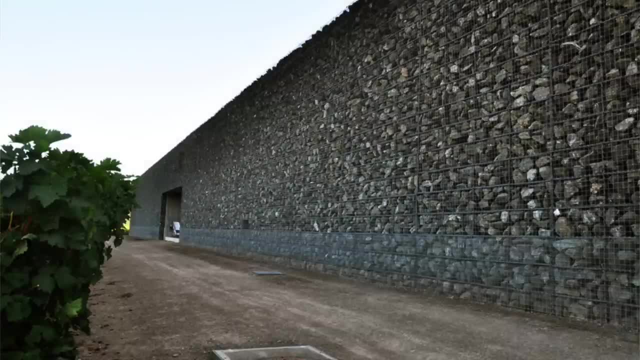 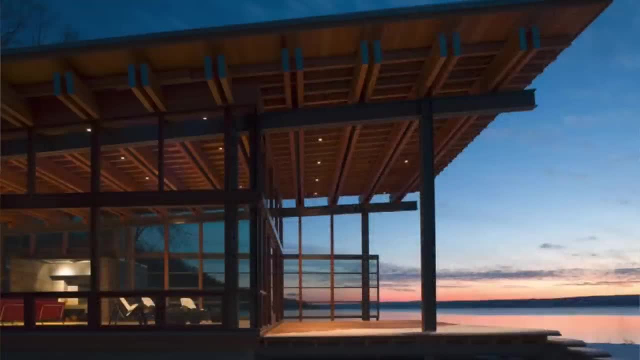 Every line we trace on the page represents real physical materials coming together to make our architecture. Instead of rendering our work in pure white, as we so often do, why not seek meaning from the materials we'll use to construct it: Local stone or wood, aggregates, tradespeople. 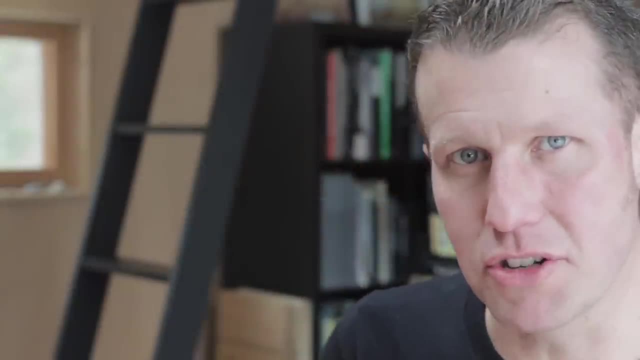 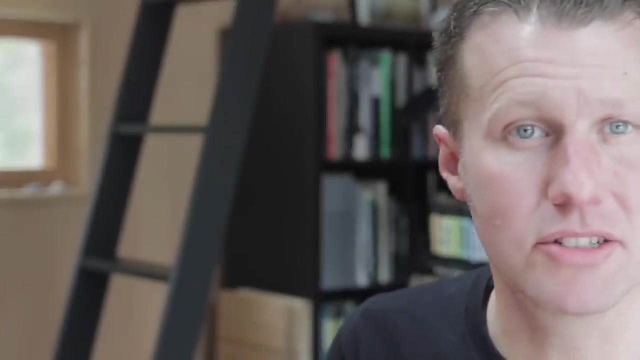 or special techniques. these can all be called into service of the architecture, and the spaces can be enriched with meaning. Materials have very specific properties by which they're bound. Steel conducts, It's strong and bending. It can be welded. Stone is heavy and thick and imposing. 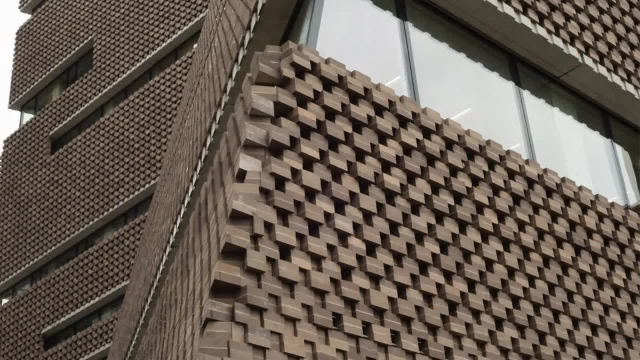 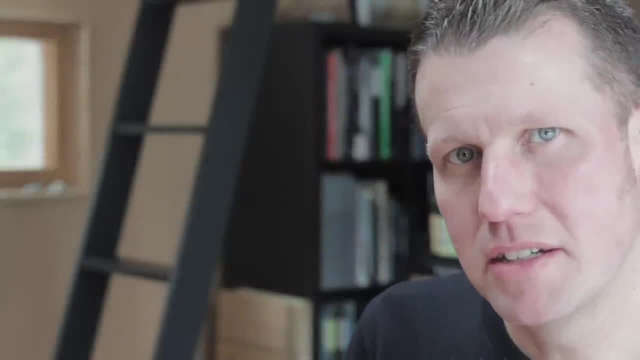 Glass is light and ethereal. Bricks are the size of the human hand and lend texture and scale and warmth to a space. Ask yourself how these materials, or combinations of them, tell a more interesting story. For my work, I'll always use the underlying narrative concept. 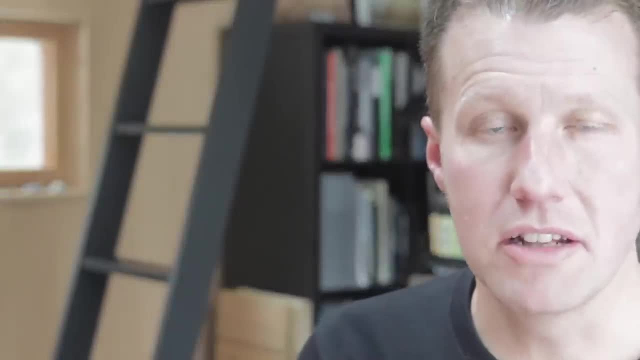 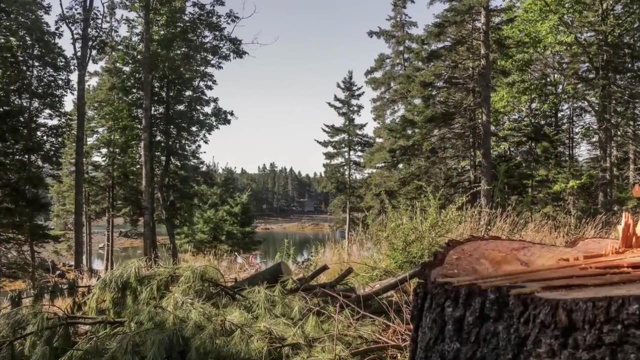 to reinforce the material concept Here we're using dark-stained local cedar shingles as the siding for our project, The spruce pine and fir forest. here is a variegated dark green. The shingles and the wood grain replicate this subtle tonal difference and the green 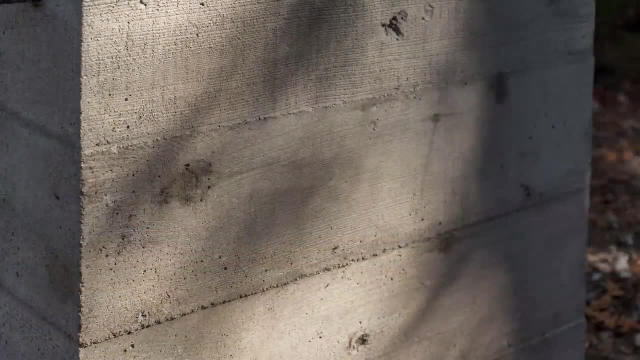 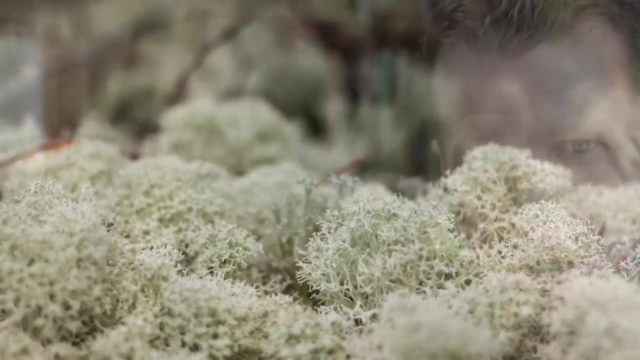 helps the building to recede into the site: Board-formed concrete references. the wood graining and the process of making Its patterns will host mosses and lichens as the building weathers. Is this a separate concept? No, it all feeds into an attitude about a place. 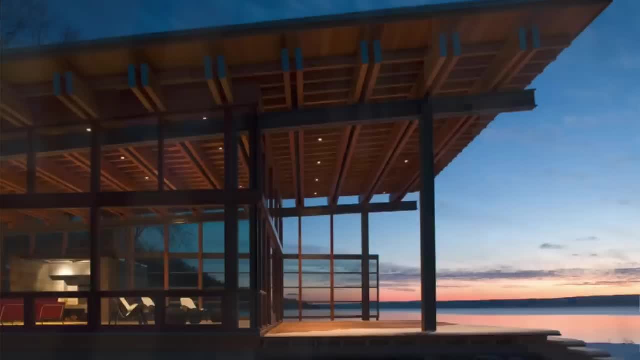 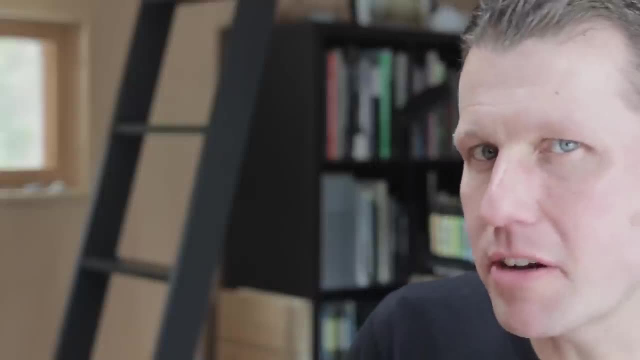 construct it: Local stone or wood, aggregates, tradespeople or special techniques- These can all be called into service of the architecture, and the spaces can be enriched with meaning. Materials have very specific properties by which they're bound. Steel conducts: It's strong and 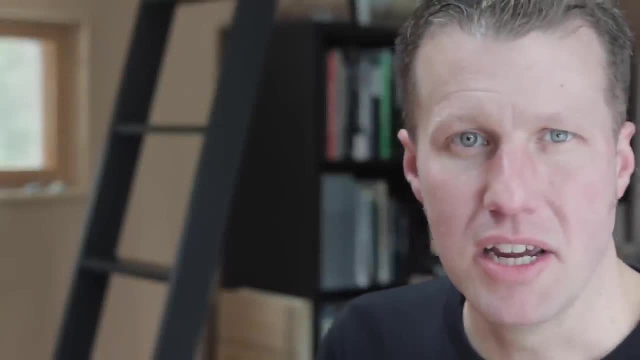 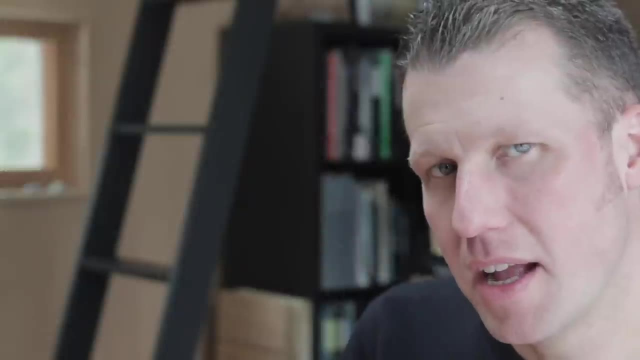 bending, It can be welded. Stone is heavy and thick and imposing Glass is light and ethereal. Bricks are the size of the human hand and lend texture and scale and warmth to a space. Ask yourself how these materials, or combinations of them, tell a more interesting story. 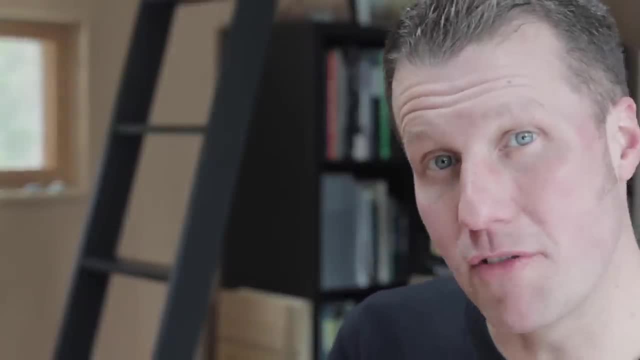 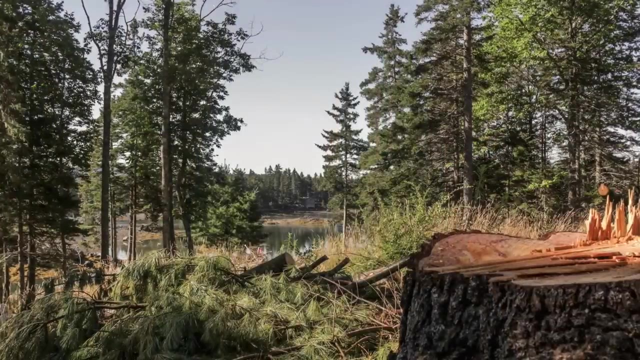 For my work I'll always use the underlying narrative concept to reinforce the material concept. Here we're using dark-stained local cedar shingles as the siding for our project: The spruce pine and fir forest. here is a variegated dark green, The shingles and the wood grain. 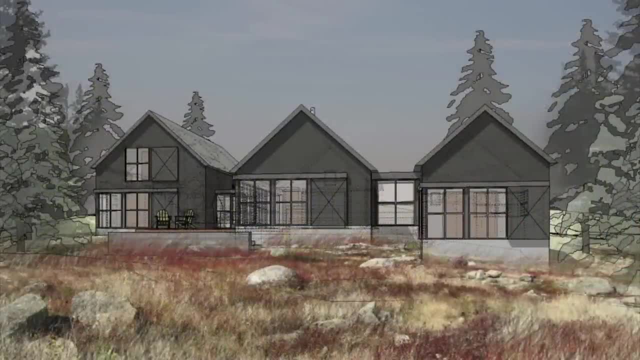 replicate this subtle tonal difference and the green helps the building to recede into the site. Board-form concrete references: the wood-graining and the rubble. In a wood grain installation, the slag board keeps the foundation of the entire building from falling apart. transitional. 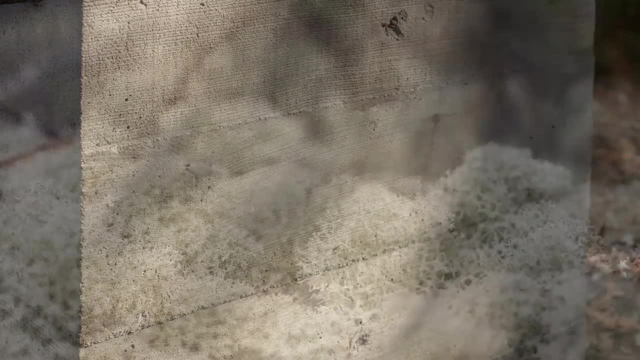 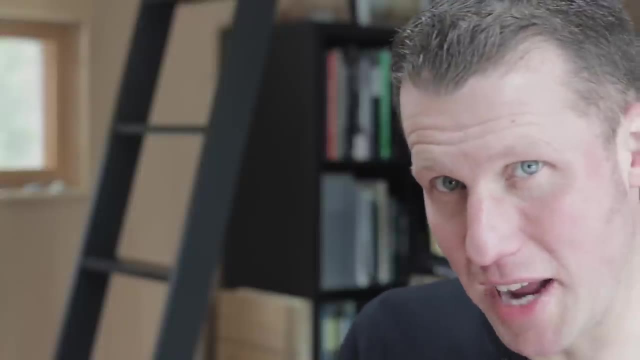 to recede into the site Board- form. concrete references: the wood-graining and the southern side of the building. the wood graining and the process of making Its patterns will host mosses and lichens as the building weathers. Is this a separate concept? No, it all feeds into an attitude about a place. 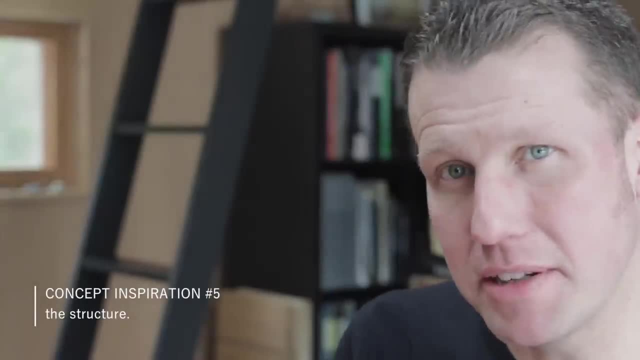 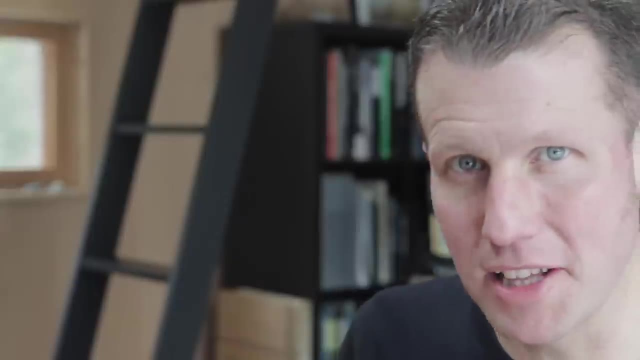 Next, a structural concept. The expedition and the camping narrative that we've been talking about helped us develop the structural strategy too. The gable form is a tent. Glazed walls let ample light in, and we're employing lightweight cabling elements reminiscent of tent poles or cordage to 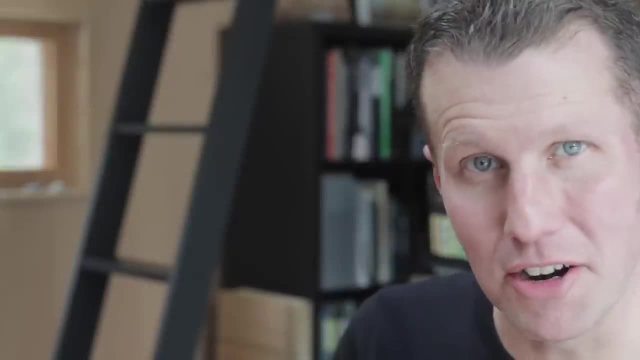 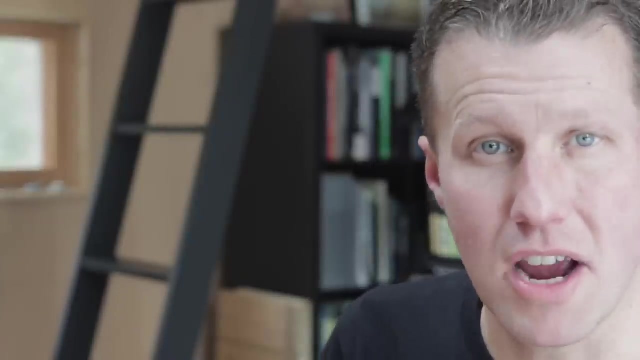 tie the walls together, And of course, there's nautical references here that are pretty strong as well. Now you could also write a manifesto. What do you believe this architecture's role is in society? What are the larger questions it's proposing? Check out Dieter Rams for a famous 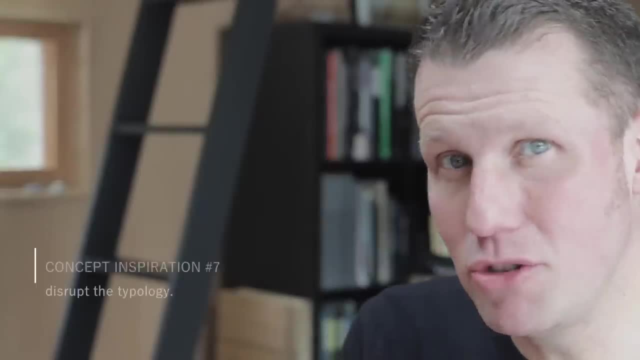 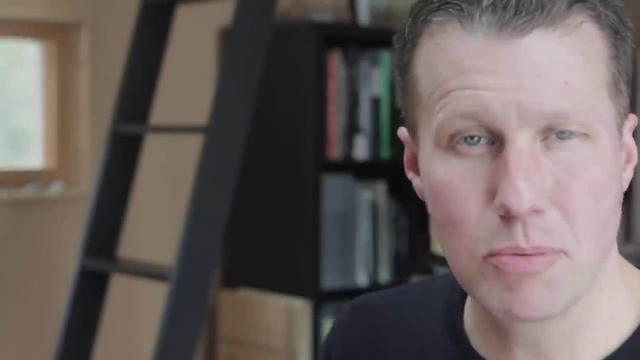 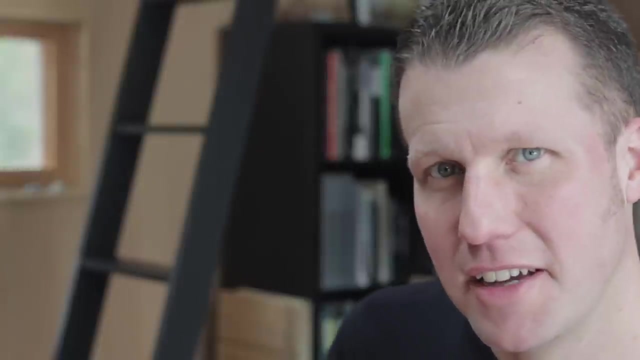 manifesto. Having researched your building typology, how can you disrupt long-held beliefs or organizational layouts, See Biggs Power Plant, for example? Perhaps you could explore a formal concept, the idea of architecture, parlance, the bird's nest, The chicken that sells chicken, And, of course, there's always the process of making Charles and 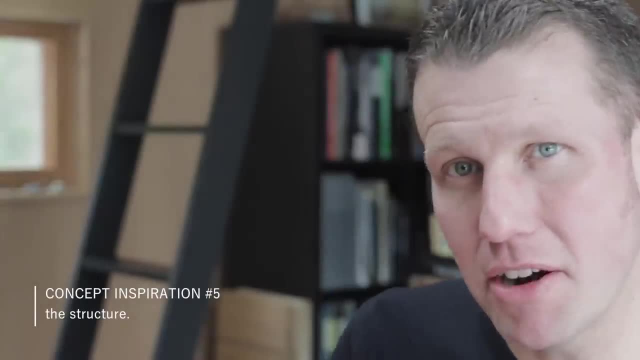 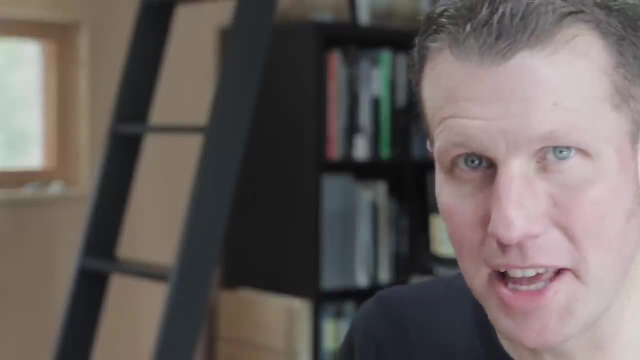 Next, a structural concept. The expedition and the camping narrative that we've been talking about helped us develop this structural strategy too. The gable form is a tent. Glazed walls let ample light in, and we're employing lightweight cabling elements. 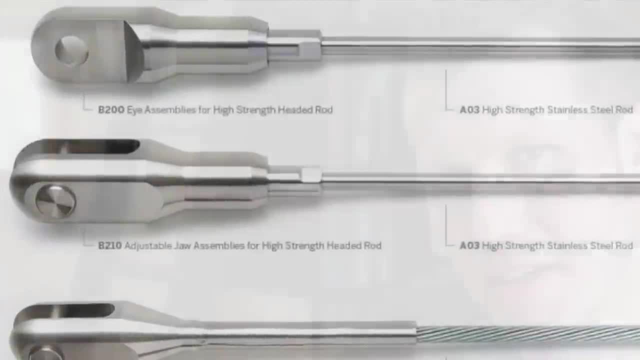 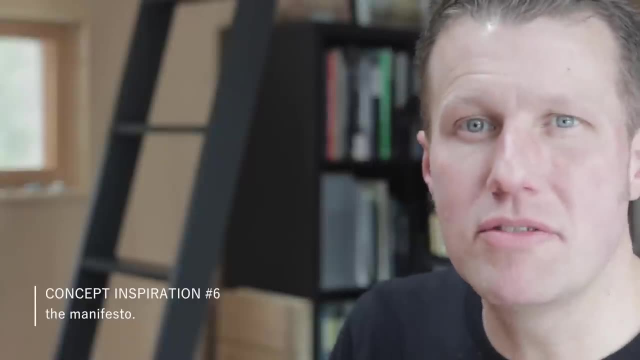 reminiscent of tent poles or cordage to tie the walls together, And of course, there's nautical references here that are pretty strong as well. Now you could also write a manifesto. What do you believe this architecture's role is in society? 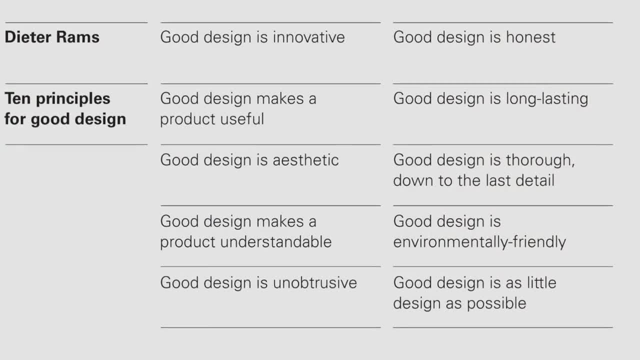 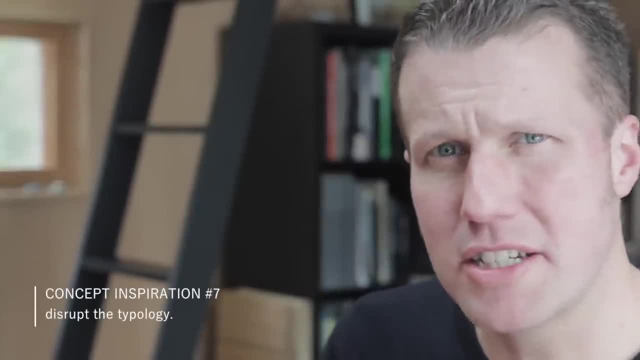 What are the larger questions it's proposing? Check out Dieter Rams for a famous manifesto. Having researched your building typology, how can you disrupt long-held beliefs or organizational layouts? See Biggs Power Plant, for example. Perhaps you could explore a formal concept. 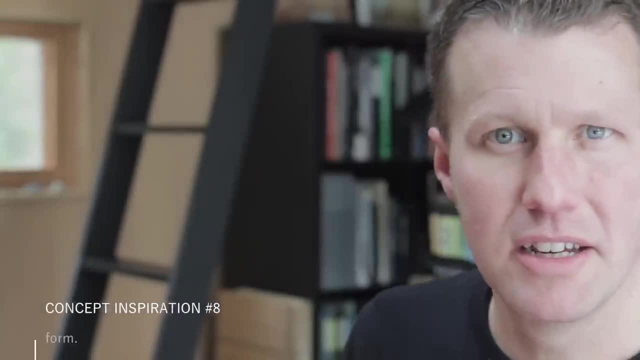 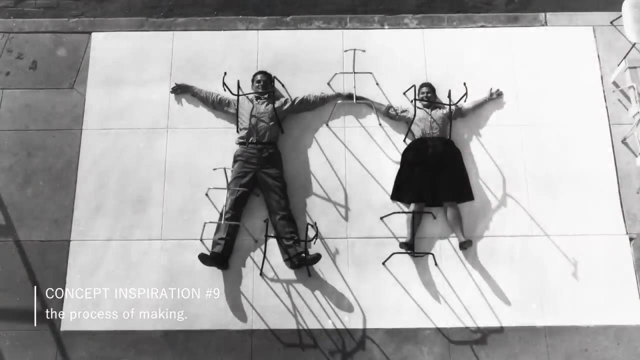 the idea of architecture, parlance, the bird's nest, the chicken that sells chicken, And, of course, there's always the process of making. Charles and Ray Ames used their journey from ignorance to knowledge as the motivation for many of their designs. How can you bring a fresh perspective? 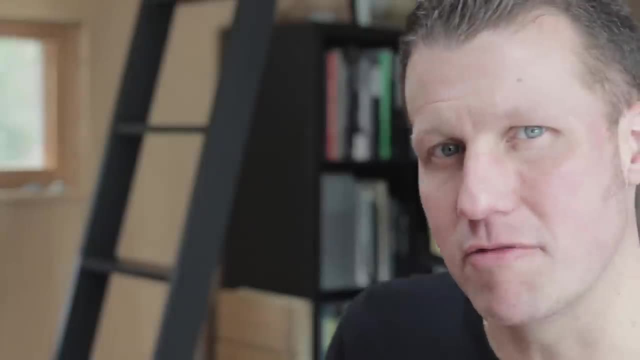 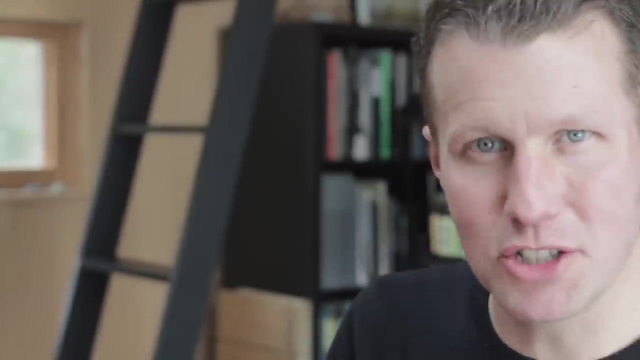 to the problem you're facing. Is there something inherent in the process of building that reveals something novel? The design process isn't singular or linear. We don't create a concept and stick to it in the face of changing information. Use what you're learning to pivot. 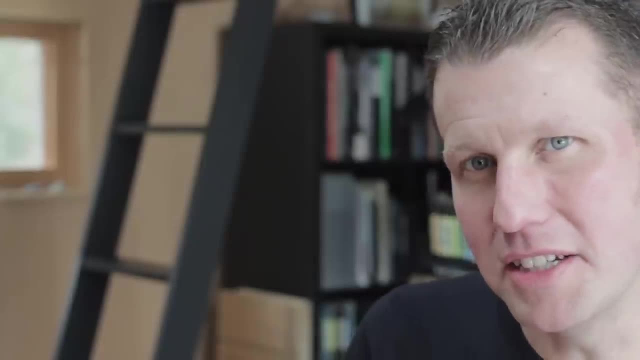 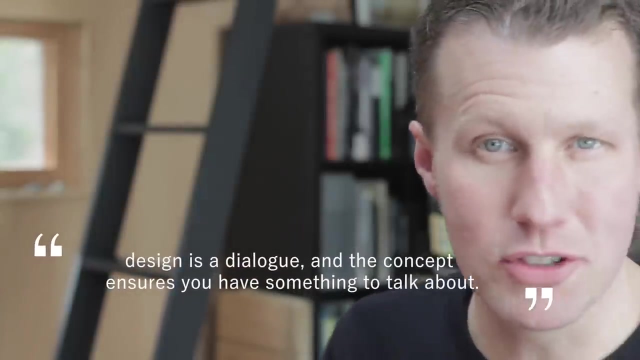 That's perfectly acceptable, sensible, even. You'll present ideas to your clients. You'll talk to your client or professor and they'll react. Design is a dialogue and the concept ensures you have something to talk about. Return to your design and tweak it. 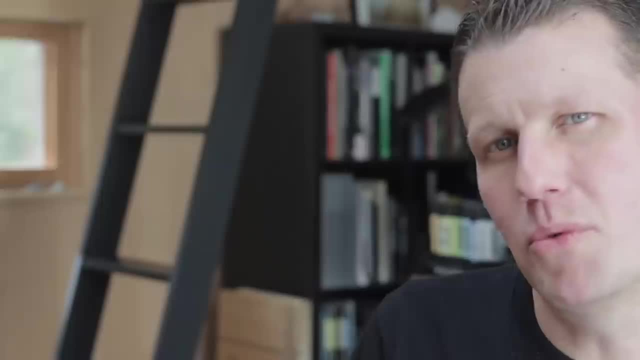 using the new information you've gathered. Each time we learn a little bit more about our client, about the design, and new opportunities arise. Now, in the next part of this short course, we'll look at how we begin turning the concept into architecture. 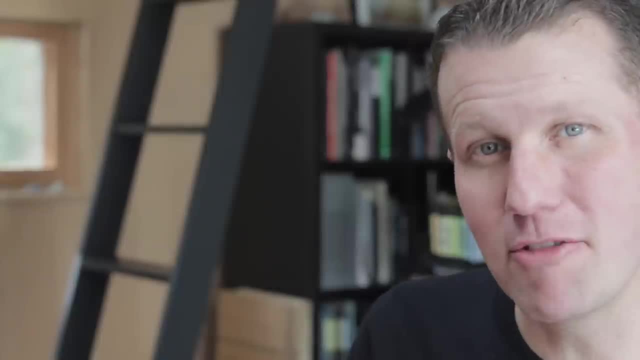 If you found this video helpful in any way, you can help me by giving me a thumbs up below and sharing it. This is how I know what I'm doing is helping you and it'll allow me to continue to grow the channel. Thanks for watching. Cheers.